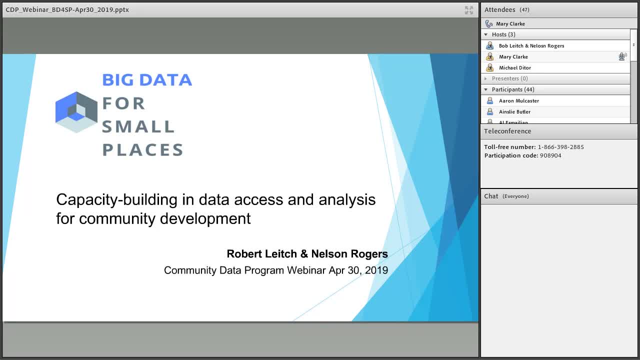 educator, administrator, an analyst on educational outreach projects, community consultation and capacity building, project partner engagement, strategic planning and project management, working with many different partners in public and private sectors. So they're really passionate about these project-based projects. So they're really passionate about these. 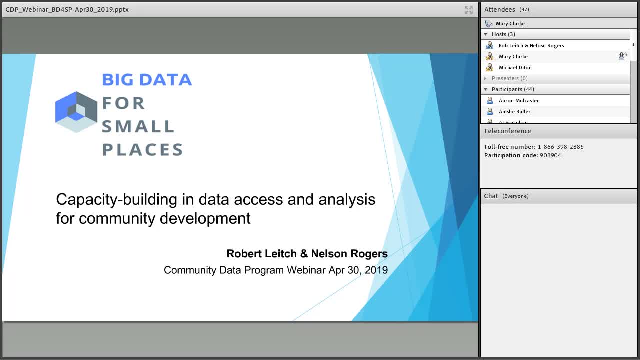 projects And I'm really hoping that you're going to see the potential here in what they're doing And we're looking for, hopefully, some potential in your own work And you can see how it might relate, how it might boost your own capacity and what you're doing. And then we're also really 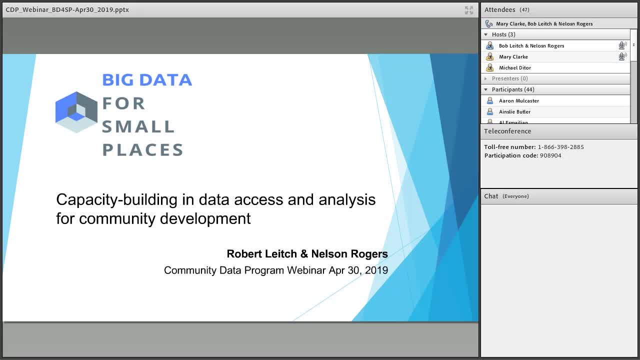 looking at how this would be a good partnership with the community data program as a whole and what the potential could be to work together. The first project they're going to present is a model and module, and it's called big data for small places. And then the second presentation. 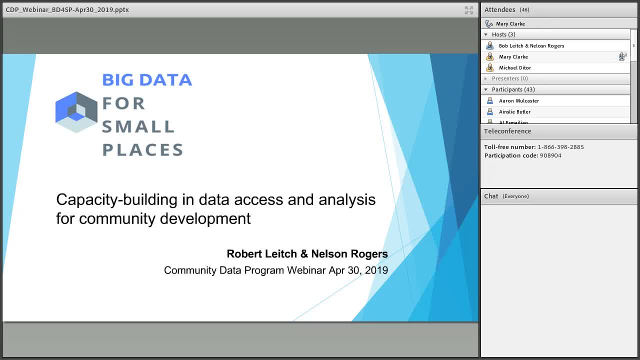 is going to be on a tool called data analytics for world transformation. So welcome to Nelson and Bob and thank you very much for giving us all your time today. Thank you, We're glad to be here. This is Bob, This is Nelson. So good morning, Good afternoon everyone. We just wanted to do. 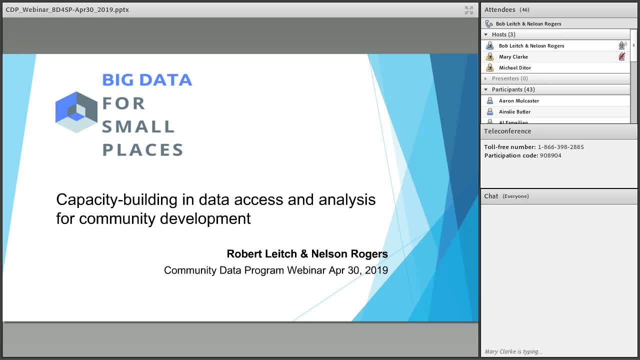 a little bit of an introduction, In addition to what Mary has shared with you as to how this all came about. Mike Dider, who most of you, if not all of you, know and who is online today, He and my son, Jonathan, are good. 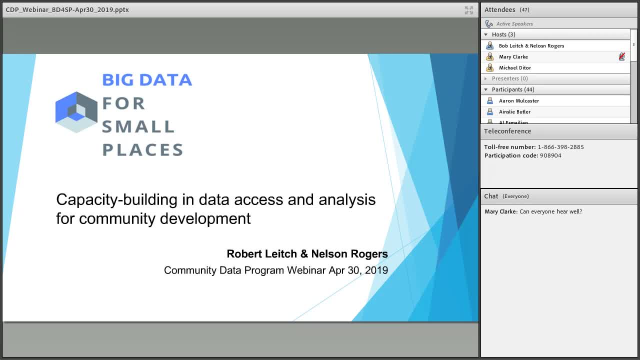 friends and have been for many years since they met at McGill And, as it turned out, we got into a conversation and one thing led to another, And Mike shared with me the work he was doing with the community data platform, And we're going to talk a little bit about that. And then we're going. 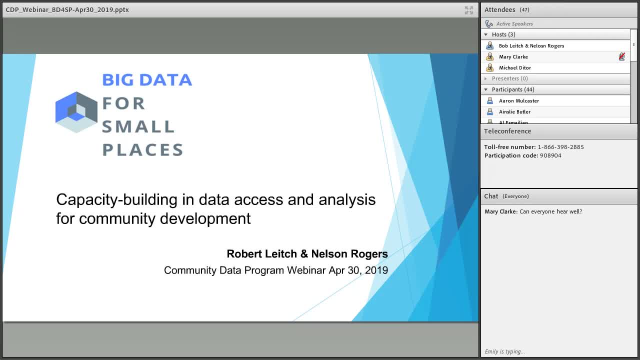 to talk a little bit about the community data program, And that resulted in us meeting with Michelle, the CEO, and talking about how we might work together going forward. We feel that what we're going to present today is very much a collaborative kind of joint venture potential. We 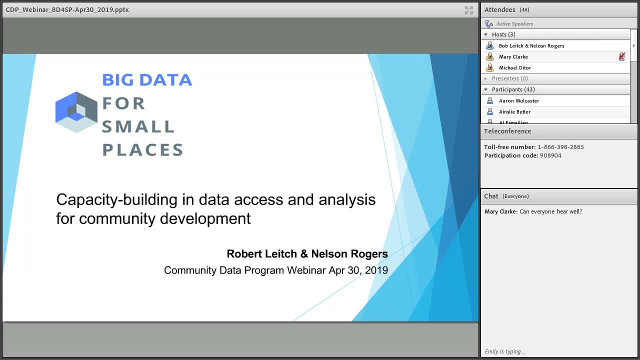 have no formal agreement between ourselves and the community data program, But we feel that there is a synergism there that we would like to have, And so we're going to talk a little bit about that And then we'll go over some of the things that we've been doing and what we've been doing And 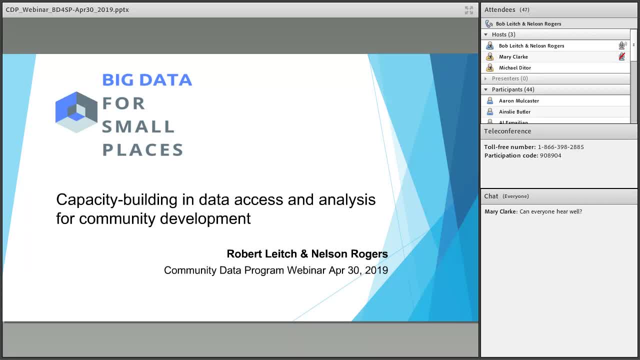 what we want to do today is to explore further. What we want to do today is to let you know what we've been doing, And we acknowledge that many of you on line today are fairly expert in the field of data and data analytics, And so we're not going to pretend that we're going to know more than you. 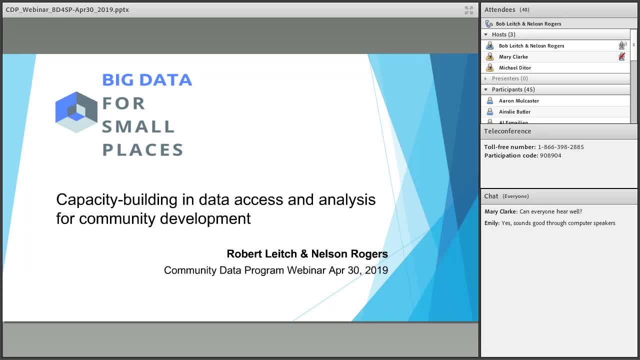 do about this sort of thing, but rather share with you how we've been approaching this over the last few years. We're hoping that this will be of interest not only to you personally, but perhaps to the people you are talking about, And so we're going to talk a little bit about that, And we'll 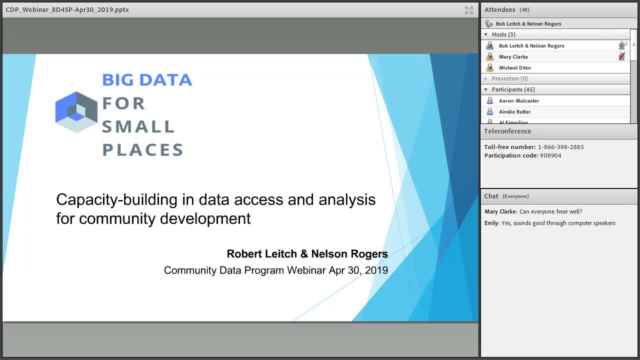 look at the work that we've been doing on a daily basis. But we're going to talk a little bit about you work with- I think probably more so- the outreach kind of programs that you do. I also wanted to share with you that during our discussions with Michelle and Mike, we did touch on the 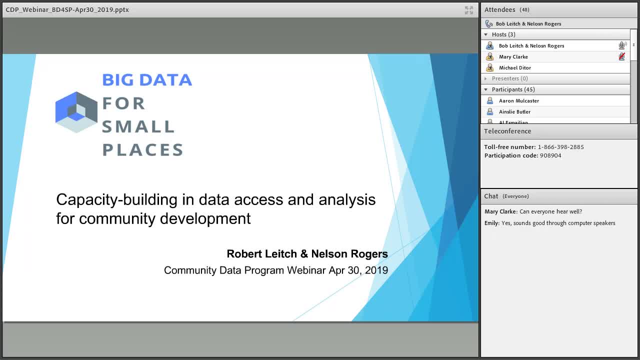 strategic plan that the Community Data Program has. I believe it's still a draft plan, although we went online today to see if there was a final one and couldn't find it, but perhaps it already exists. However, the point of me bringing it up is that in there there's a section on training. 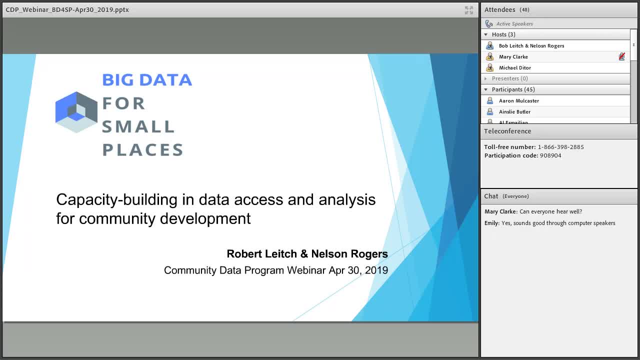 and capacity building, which talks about, basically, data literacy, And that's really kind of the focus of what we're going to talk about today. So that's kind of a quick introduction as to how this came about, And, Nelson, would you like to add anything to that? No, that's good. Okay, So let's begin. 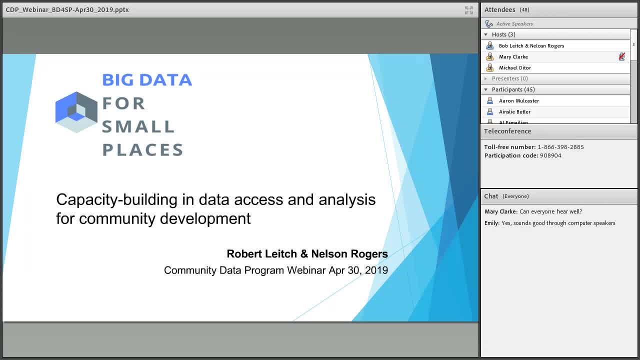 And first of all, Big Data for Small Places is a term that's really kind of caught on for us. We've had a lot of good results from that terminology. Interestingly enough, Mary Clark, the lady who introduced us today, brought up an interesting concept when we spoke not too long ago. We kept referring to 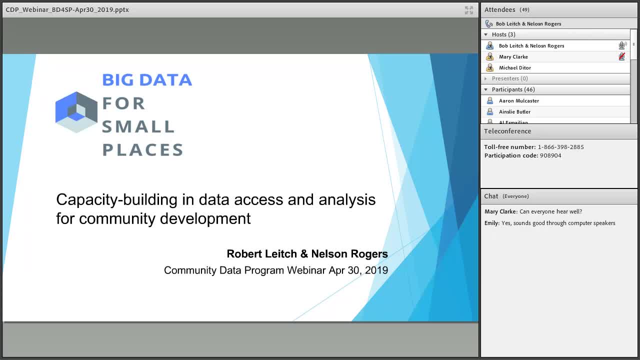 Big Data for Small Places in the rural context, And while that's our primary audience and objective, we also were reminded by Mary that there are a lot of communities within urban centers, So smaller communities as part of larger urban centers have some of the same data issues as rural communities do. So interesting kind. 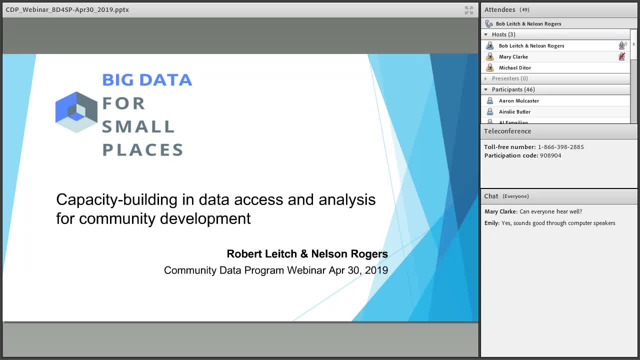 of perspective that we took to heart And we've been talking more about that more recently. So it's this program and it is a program, And I think off the top, we want to mention that this isn't really a traditional course. It's not where we have a curriculum per se, but we do have a very strong 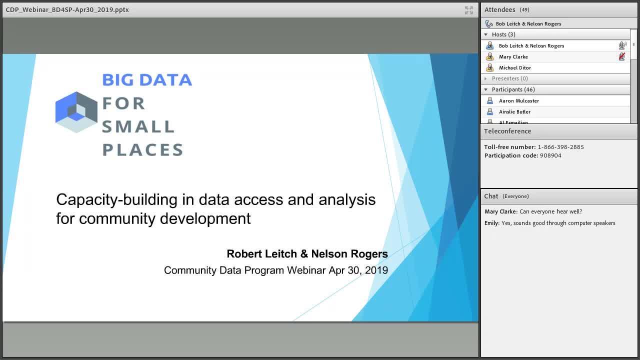 framework, which we'll talk about momentarily, But it's more of a capacity building program than a course. So, as a capacity building program, our focus is around accessing data, where to find it, analysis of data and then, ultimately, how to present it to the public, And that's what we're going to talk about today. 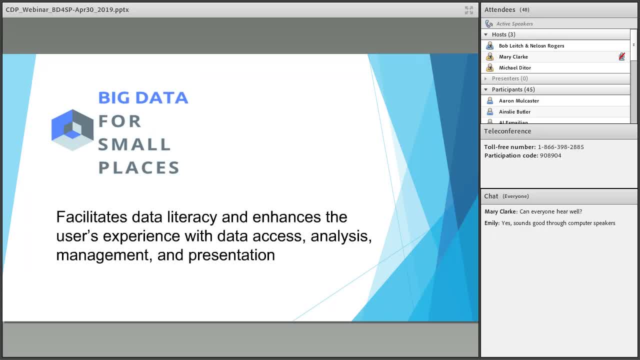 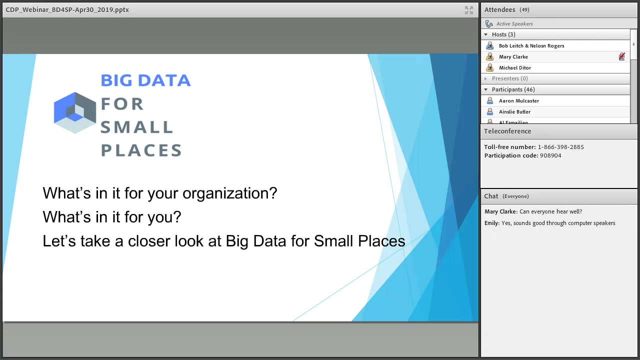 That's going to talk about smaller places and how we utilize data to meet the local needs and how we might evaluate and determine and visualize data to helpね us connect and practice and visualize of data and presentation of data. so we want to try and deliver to you today. 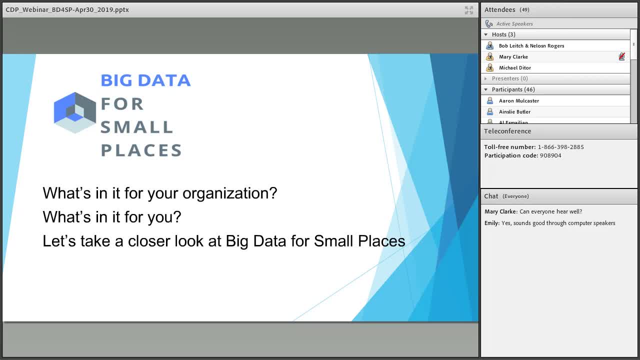 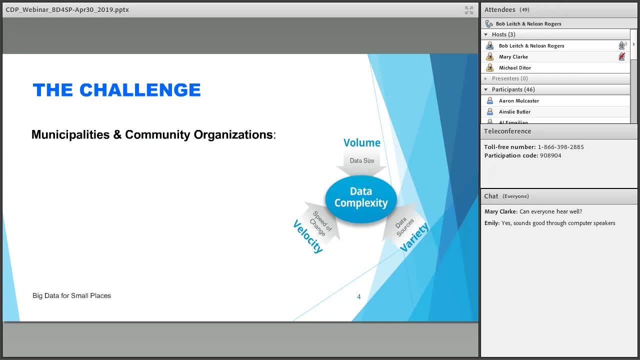 what we feel this might have for your organization, for you as a person who works in the world of data, and to take a closer look at what our program, big data for small places, is all about. so Bob and I've worked in rural research and consulting together for several years. before that, I worked for Algonquin. 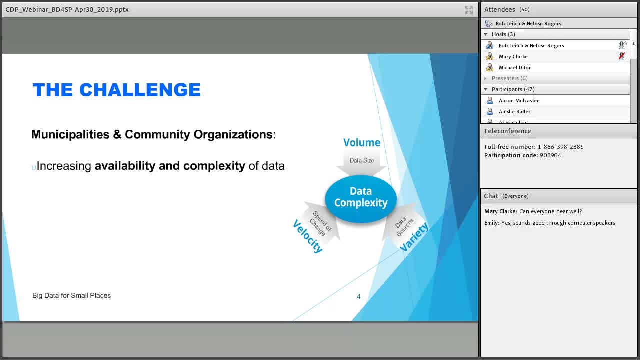 College for about 30 years, and a chunk of that was it a rural campus and I also worked with a network of rural college campuses and our approach has been to. you know, we've been doing a lot of research and we've been doing a lot of. 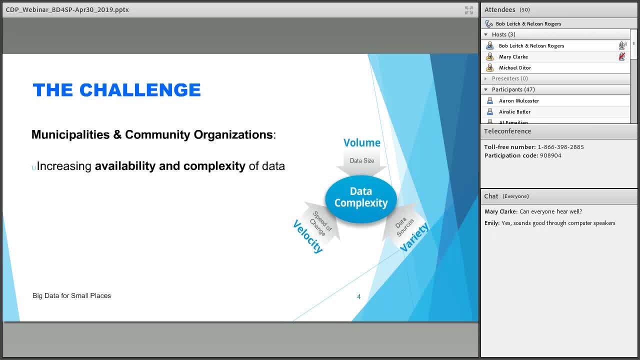 to try to listen to what we're hearing from rural communities and then respond to local needs. so we're we're a little bit in the mold of what I call on consultants, where we're trying to use our consulting services to put to help our clients use consultants less so we listen to what municipalities and 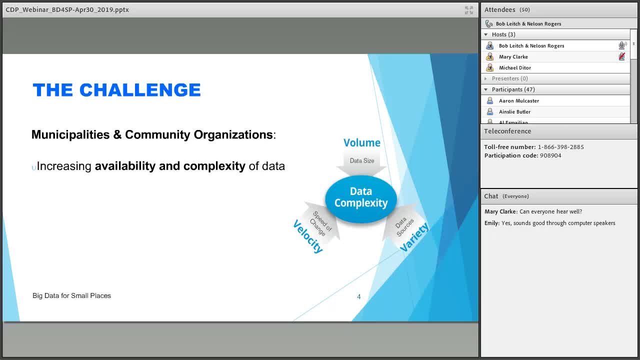 community organizations were telling us about their data issues and what they were saying is that there's so many open data initiatives. we're located here in Ontario and OMAFRA, Ontario Minister of Agriculture, Food and Rural Affairs, has over 200 to open data products available just in one ministry of the Ontario government, so increasing. 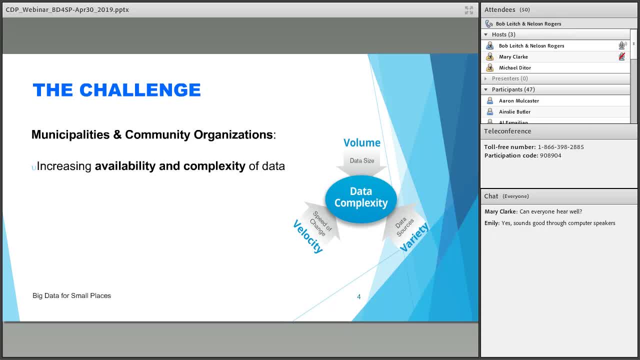 availability of data and data in a lot of different kinds of formats and accompanying that is. community groups are facing increasing requirements to use data that they can't apply for a grant, can't complete a grant application or or complete an annual report without extensive use of data and and many groups are finding they're contracting. 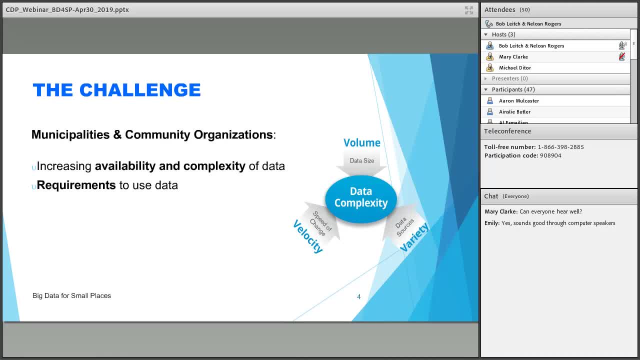 that out because they don't have the internal capacity to to deal with that. of course, this is all under the the theme of evidence-based decision-making, and that's in increasingly important for a lot of organizations, and what we were hearing from the groups that talked to us was that they felt they were missing. 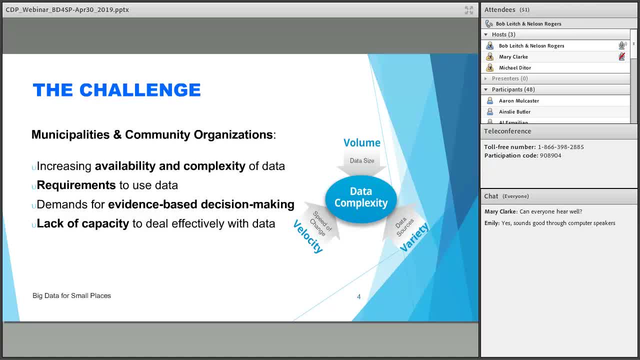 opportunities or missing a deep understanding of their local community because of their lack of capacity to deal effectively with data and and, as a result, we're often relying on popular opinion and local knowledge rather than what some might consider hard facts, and and so we took all of this into consideration in 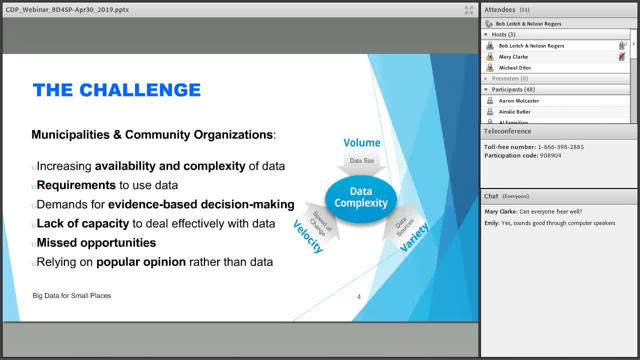 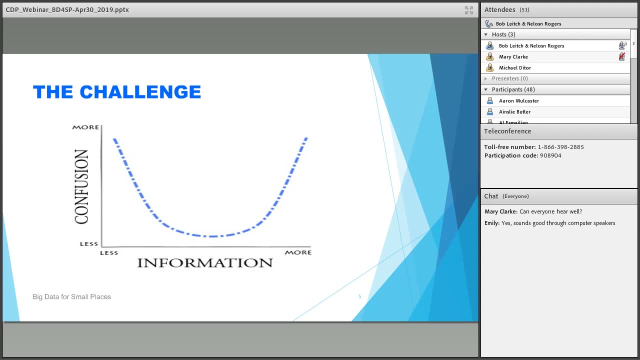 designing the program, we used instructional design expertise from a college and from some retired instructional design experts that we happen to know personally, and we put this into a into a program format that can easily be shared and replicated. I guess it the situation we're dealing with this on the slide about the 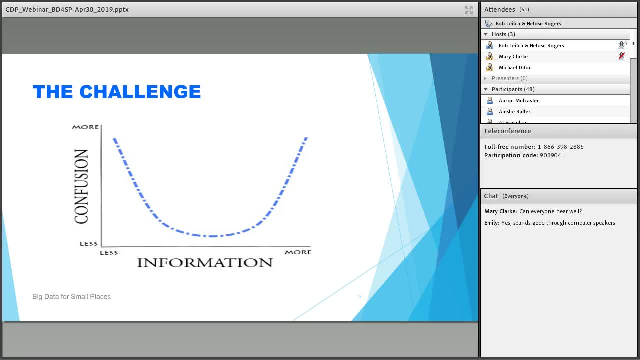 challenge of the confusion information graph is: it is a u-shaped graph and we found, as we're dealing with community groups, some are feel they're they're high on the confusion level because they don't have enough data and some feel they're high on the confusion level because they have way too much data and 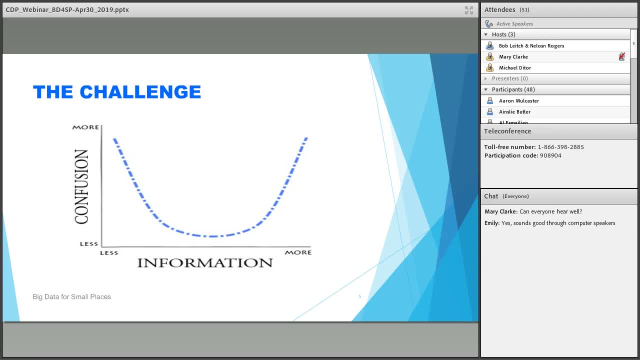 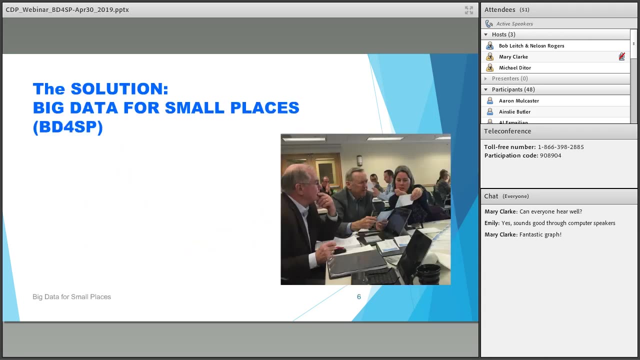 we're trying to work with groups to help them find that spot where they're comfortable with having adequate data and adequate local understanding to make reasonable plans and and evaluate their programs are adequately. so our goals for the big data for small places program is really about building capacity, not about reliance on external 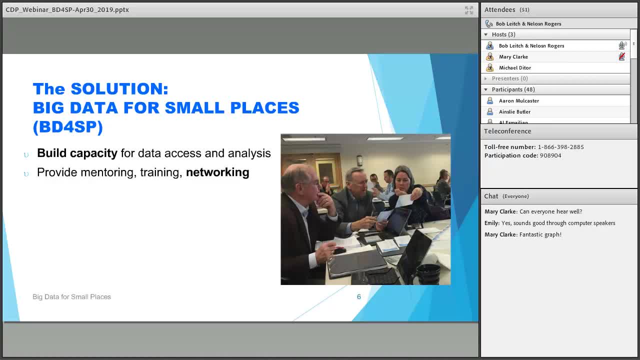 expertise. we use a series of activities around mentoring, some training modules and and largely around networking, and you know so. the community data program is an example of one of the networks that we refer people to, but there are a number of data related networks that local groups find useful and and 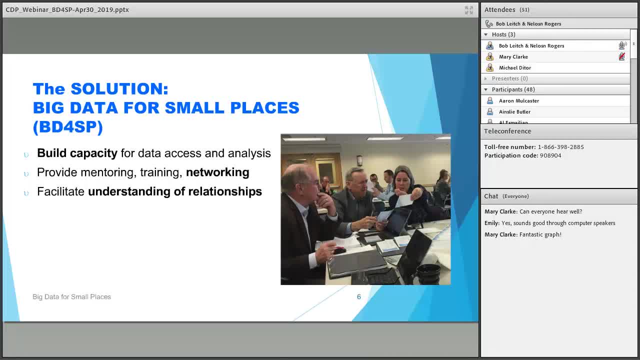 and we have some tips on how to identify the right networks and how to use them, how to understand the relationships between local and distant networks. and we also find that 20th century Community Development- this is a broad brush statement was- was largely siloed into compartments of economic, social or cultural development. 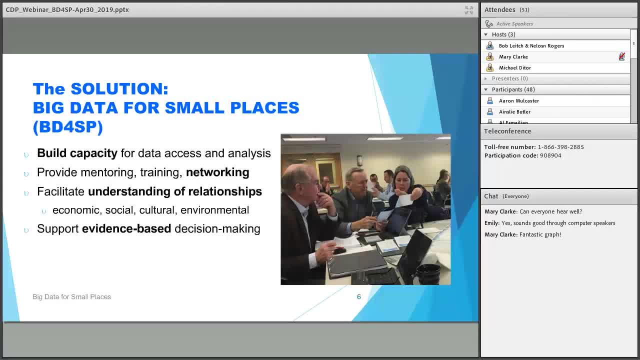 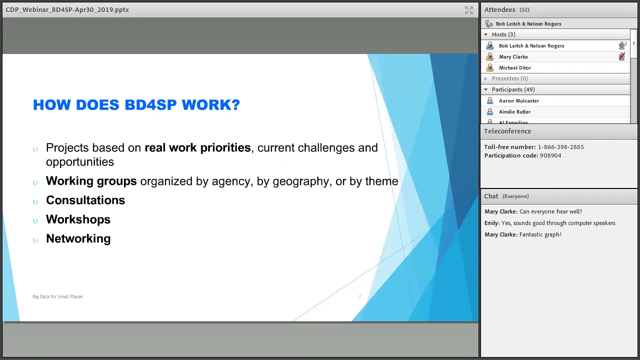 where the 21st century community development is more integrated and requires a broader understanding of various issues that can feed into evidence-based decision making. So, as Bob mentioned, ultimately the program is about increasing data literacy. So how does it work? Each working group that comes into the program has to have an actual work priority, a challenge. 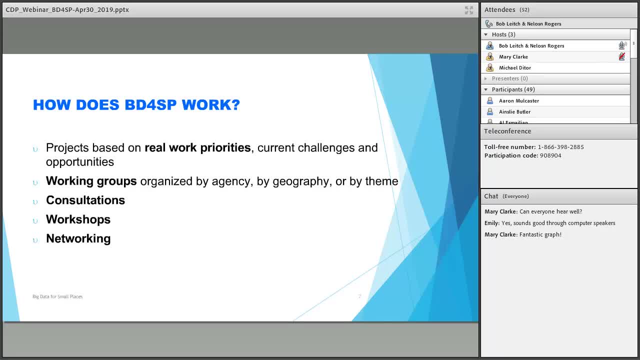 an opportunity, a question, an assignment- sometimes it's a grant application or something- and they bring a real project to the session to work on and then we coach them through the process using something that matters to them. So it's different from an academic course where the group work is theoretical. 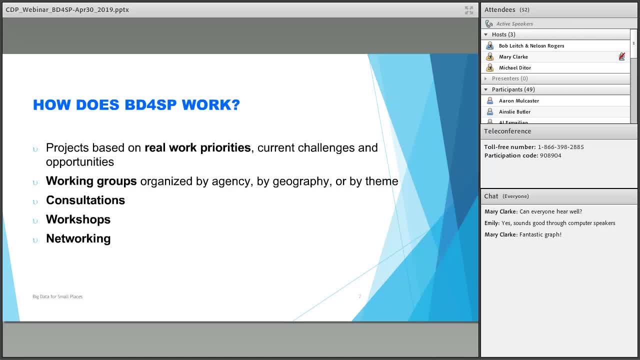 Working groups have come to us wanting to be people together, sometimes by agency, by employer, sometimes by geography, because they're working with a common issue around a particular locality, sometimes as small as a village or a neighborhood, And we've had some interesting groups. 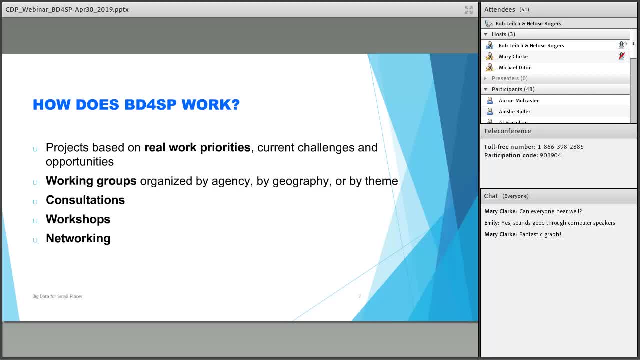 Some groups come together by theme. For example, the rural school closure theme attracted people from quite a wide geographic range because there are a lot of different communities in different places and people interested in the work for different reasons. And then the program works through a process of consultations with individual working groups. 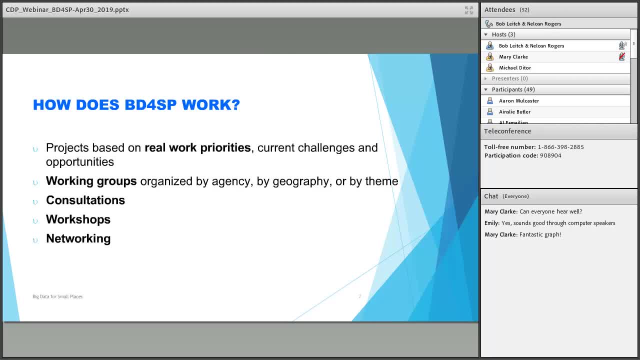 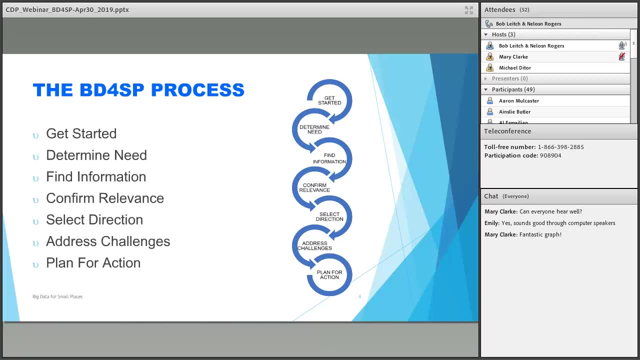 before the group session starts, Then a series of workshops And then the facilitation of networking. that will continue on after the program ends. So we have a kind of a hand-off process. We've developed a process map that gives some guidance, and this is explained in much more. 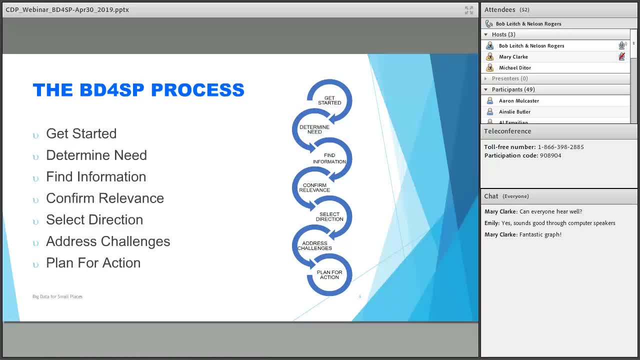 detail in the workbook that we've produced for this. There's a user handbook that was produced with some assistance from Rural Ontario Institute and the Ontario Ministry of Municipal Affairs, But just walking through how you determine community need and we've adapted some modules. 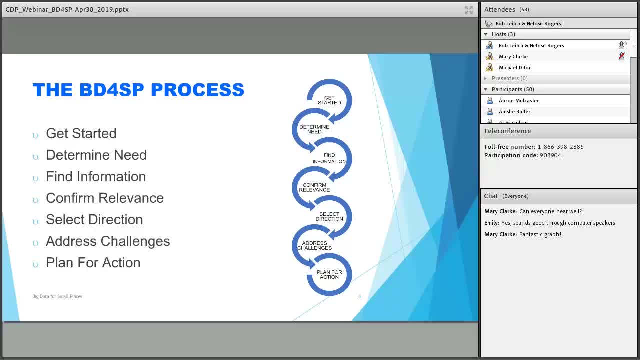 from some training that's been quite successful in the UK in training groups around county services on how you determine what a community needs, Then some processes around finding information And then we've also developed a process that's been quite successful in the UK in training. 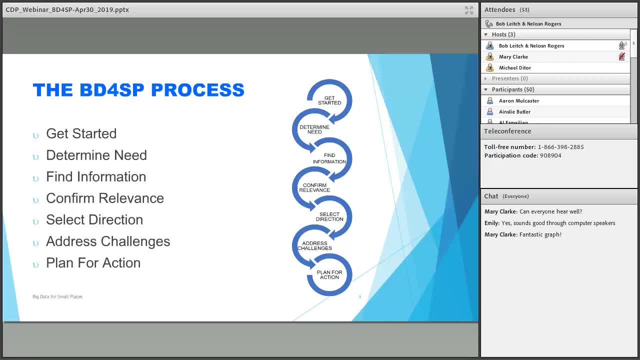 groups around county services on how you determine what a community needs And finding the right balance between, say, official statistics and local knowledge And confirming that the information that's been found or provided. in some cases the groups find they have information data reports dumped on them and they have to sort through. 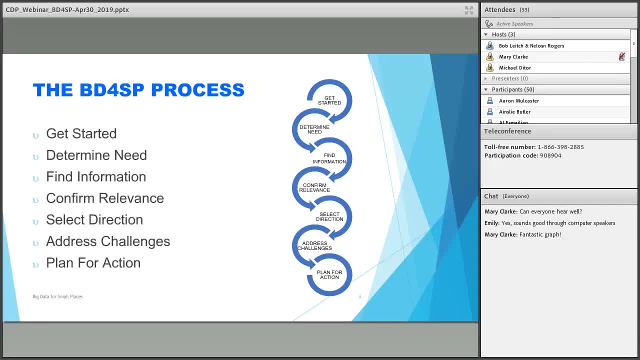 to find what's most relevant. So, working through refining a direction, We use the metaphor of a funnel around the direction setting because we find groups often come into this process with pretty broad general goals. So you know, I want to make the world a better place, sort of goals. 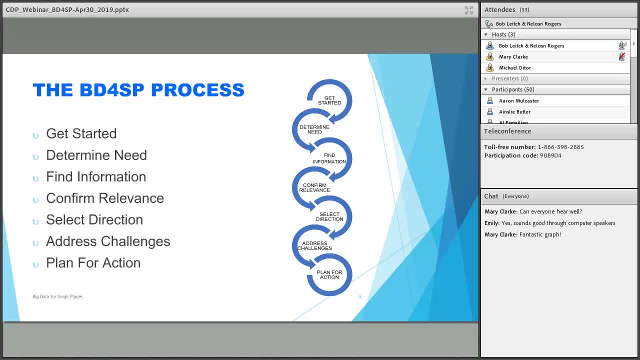 And we help them work through. let's work this down to something that has an achievable goal and measurable outcomes and visible results, And 711.751.TOE.8.007. associated with our scenario, And uh, kind of refine the direction that way, uh. and then the address challenges section is: uh, there's. 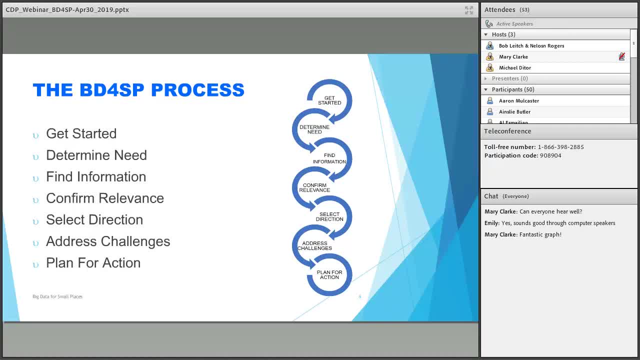 always some bumps in the road where some groups come along and say: well, you know, what we found out was a complete surprise to us. now we realize we've got to rethink some of the things we're doing before we get into an action plan, and so we have some processes that we help groups work. 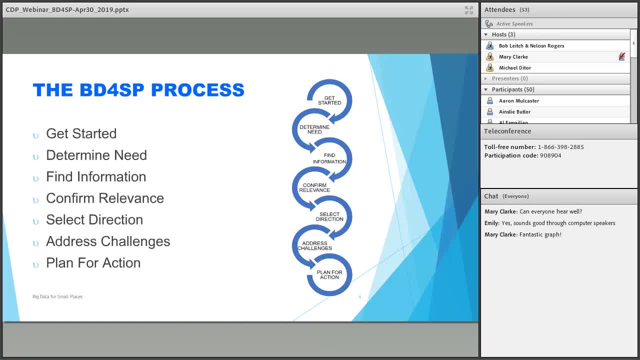 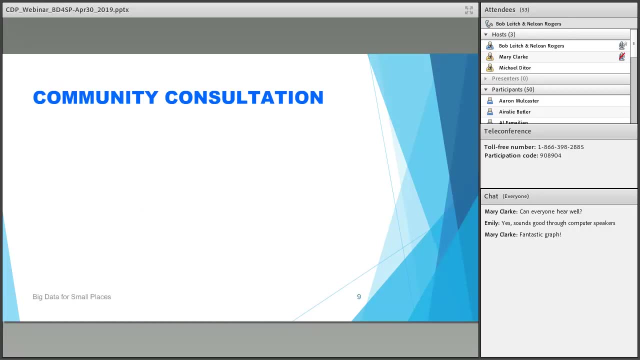 through on on getting over some bumps in the road and actually, by the end of the program, they should have an actual uh action plan, something that they can take home and work on. so that's uh. that's the process in a nutshell. just um, we're going to switch over to bob here now and we, um, i guess one. 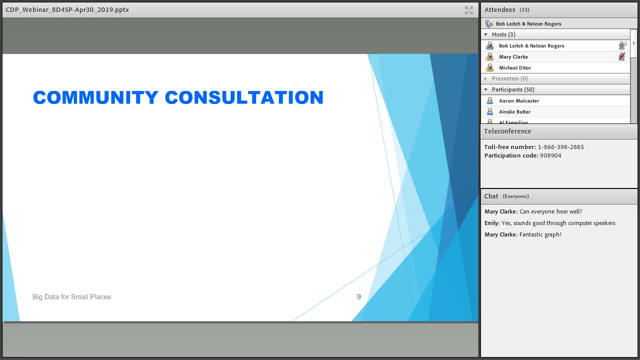 of the things that's really important about this program is that we talk about data plus. inference equals information, because so often you have to apply local experience, local knowledge, to make sure that the data is relevant to what it is you're applying it to. so that's one of the areas that we try to. 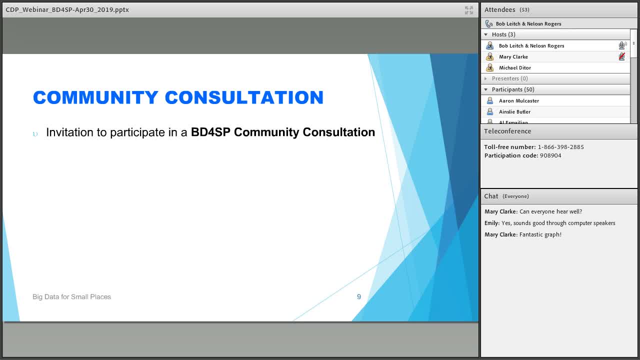 strengthen people's thinking around. so we begin the program with a community consultation, so before we have the entire group in one room and this is an in-person kind of program, we are working on the idea of having this as a interactive online version of this, but at the moment that doesn't exist. that's certainly one. 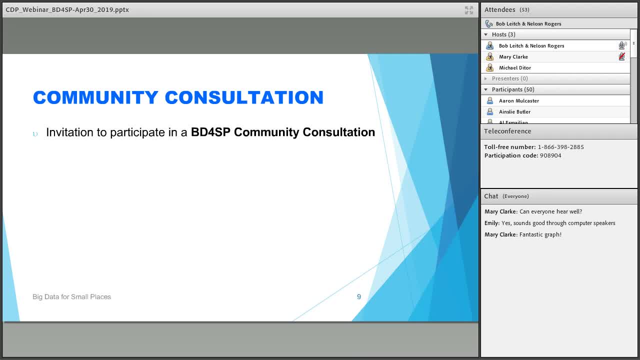 of the objectives we have. but before we bring the groups together- and typically we'll have groups of five or six in a working group and we'll have five or six groups, so anywhere from 25 to 30 people typically take part in one of our sessions. they may be working on different projects and 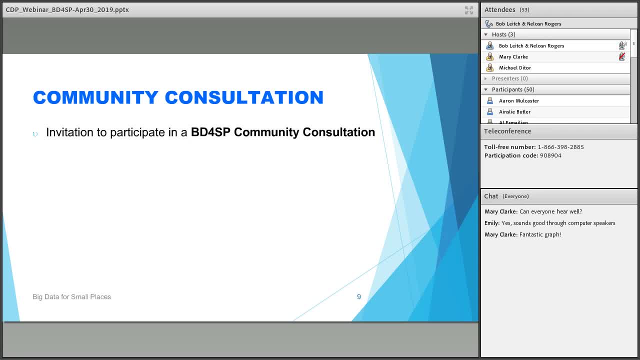 different uh focus on different projects and different uh projects and different uh focus on different topics and they may be from different organizations working together or from one organization. it depends on the circumstances. so we send out an invitation initially to put together a community consultation and we find the people who are interested uh in clusters of the teams. 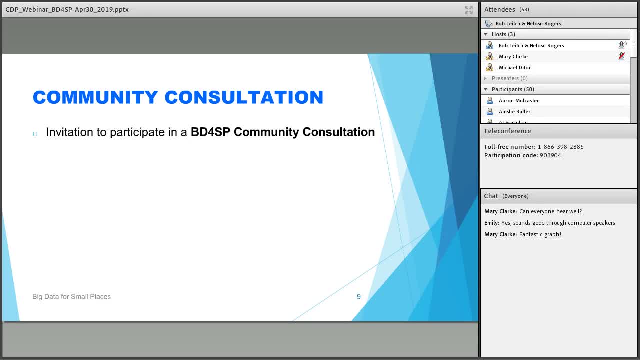 that are going to be brought together and we start the process by meeting with them individually before we get into the classroom situation. this helps us identify, uh, first of all, their level of knowledge and where they are on the continuum. uh, they may be very experienced. they're not experienced at all. so we like to know those things. 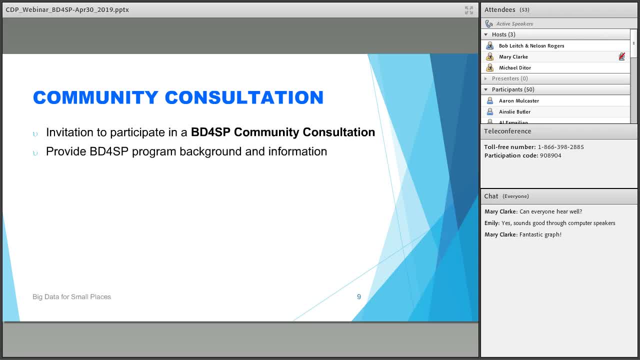 we also hope to try and help them focus their attention. so we provide background to the program, so they understand what they're getting into, and then we explore the prospect, the prospective list of projects, and that's really an important part of the program. it's an important part here because nelson was mentioning that sometimes people bring a much 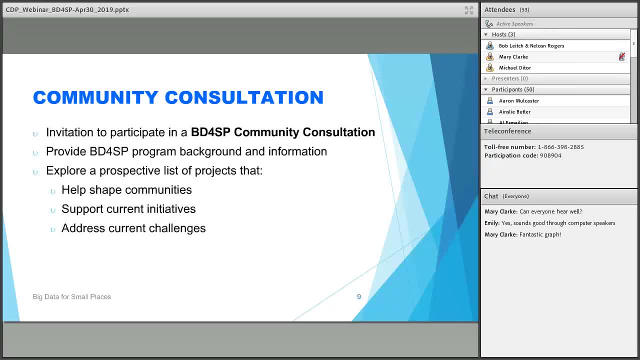 too large an issue to the table and we have to help them sort of narrow it down and make it manageable so that they can be successful. so, um the um, they're either addressing current challenges or they're looking at supporting initiatives that they're starting, so it could be anything. 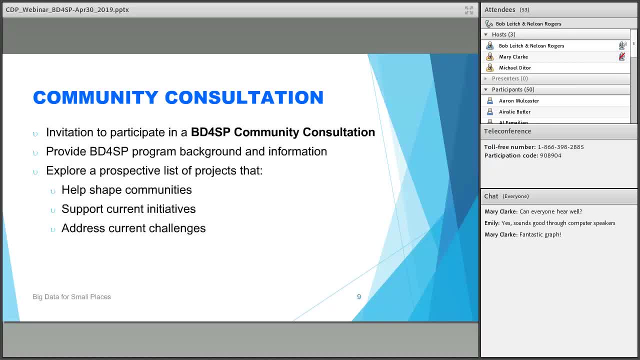 from a new program they're trying to introduce, or one they're trying to, or one that they're trying to defend in terms of funding. we, of course, then solicit participation and we answer questions that they have. so this opening session, or consultation, is really meant to strengthen and bring people together so that 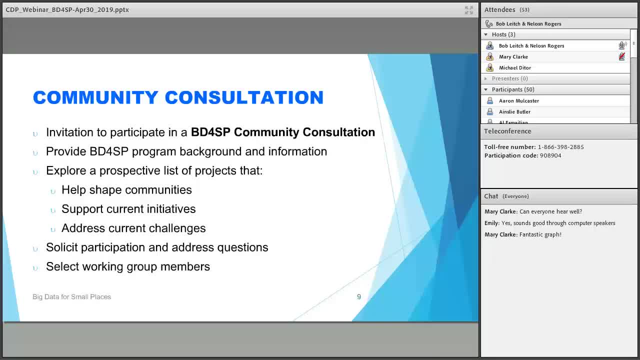 we can get each of the working groups, uh, more focused and so on. now the last point about working group members. we learned- and this was of we've got this feedback from the sessions we've done previously. initially, uh, we, this wasn't a focus we had, but it's become one and that's the makeup. 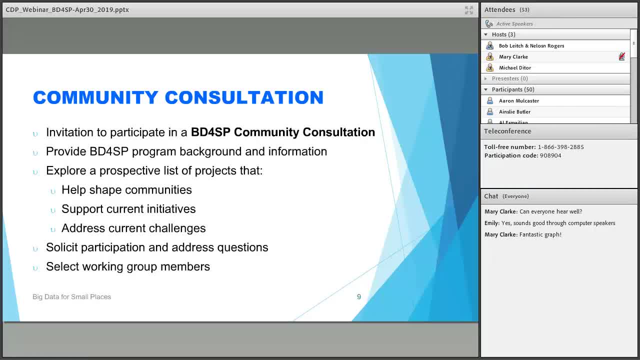 of the groups, of the working groups. um, typically we will want to see that they've got a mixture of some of the- and we're talking about skill sets here, not individuals. clearly, we don't always know who the individuals are, but we want them to have some. 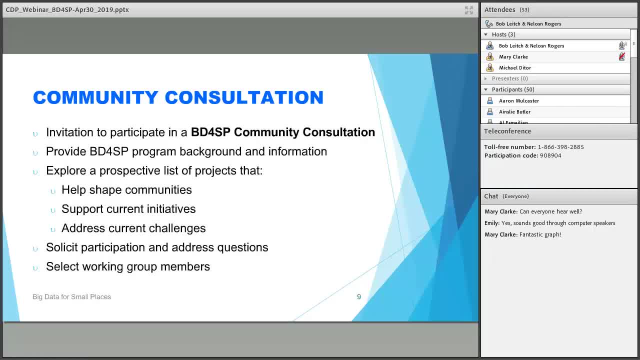 skills, uh, in communication. we would like at least one person on the team to have some research skills. might be a public librarian, might be someone who just simply has that background. we want someone to be on the team that's a content expert of whatever the focus of their group is. so 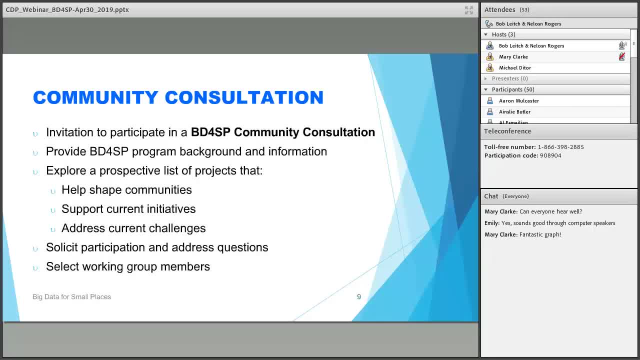 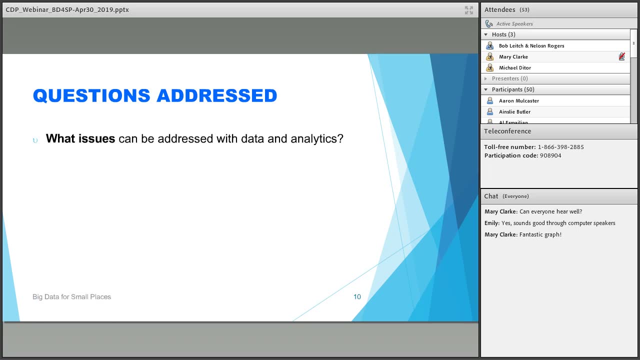 if it happens to be rural transportation, that somebody on the group knows something about rural transportation and the issues around that. so this examples of the kind of makeup of the working groups. so we we look at, uh, how questions can be addressed and we're interested in what the issues can be addressed with data and analytics. we know that. 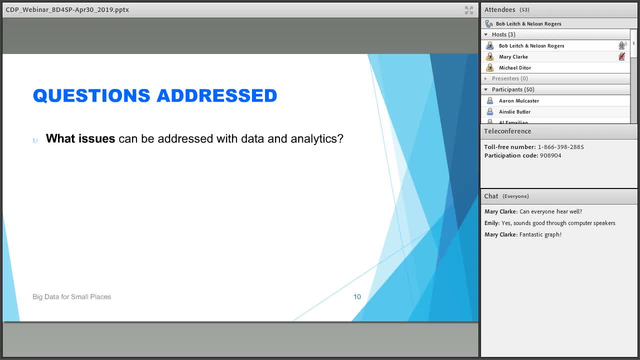 some things are not going to be easily addressed by data and analysis, so we try to identify those questions. um, we look at, uh, how data can improve or understand the community needs. we have a whole chart, it's in the workbook. but, um, nelson could maybe speak to that just for a second to. 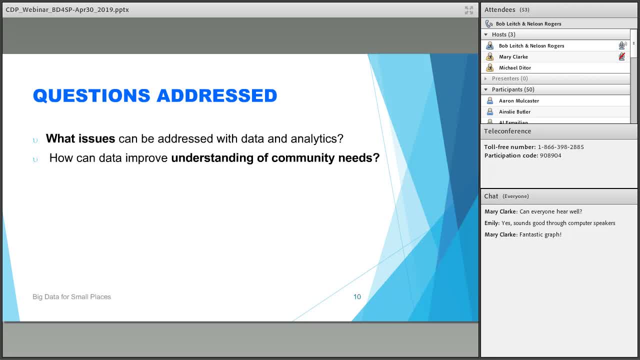 talk about community needs. uh, well, as i mentioned, based on the um training modules that have been used in the uk, we have a framework for understanding community needs and how to to choose an approach that's appropriate to the project or the organization. so in some cases, uh, community need is established by 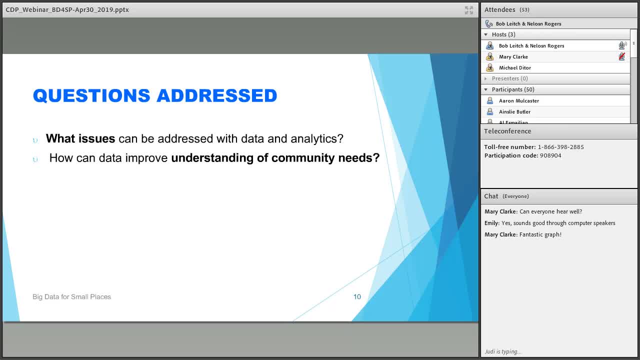 expert opinion. this is, you know, particularly around things like, uh, measles vaccination. uh, you want expert opinions on on what level of vaccination the community needs to be resistant to an outbreak of measles. uh, in other cases, it's a more comparative approach: how does our community compare with what other communities have? so are you comparing to? 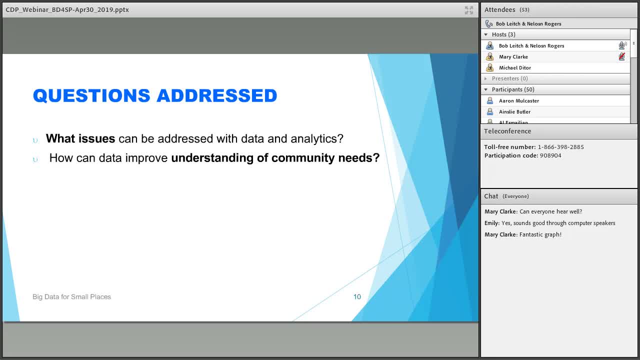 a similar community. are you comparing to provincial averages? are you comparing to national averages and why did you pick those comparisons and why is that an appropriate way of defining community need? in other cases, it's responding to spontaneous demand. that has your organization had a lot of people? 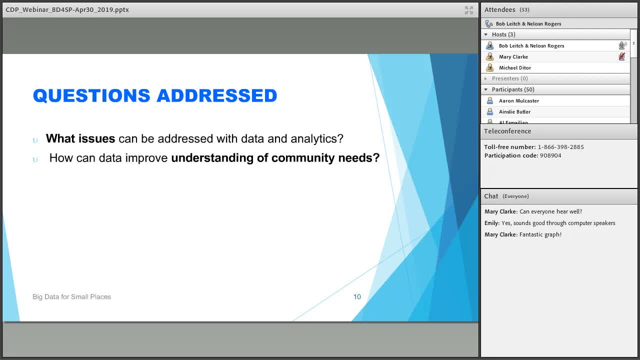 who've inquired about something and this is what they've. uh, this is what they believe they need and this is what they're asking for, and uh is that? uh, you know, provide enough information to uh develop a program to address it. uh, ontario 2-1-1 has just done a study of that around. 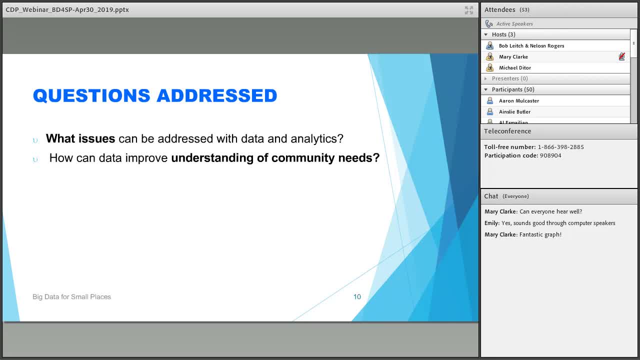 people who call 2-1-1 requesting help with something for which there doesn't seem to be an obvious answer, so that data provides some, some information about spontaneous demand. so then we have: sometimes responsive demand is an indication of community need, where you go out to a community with 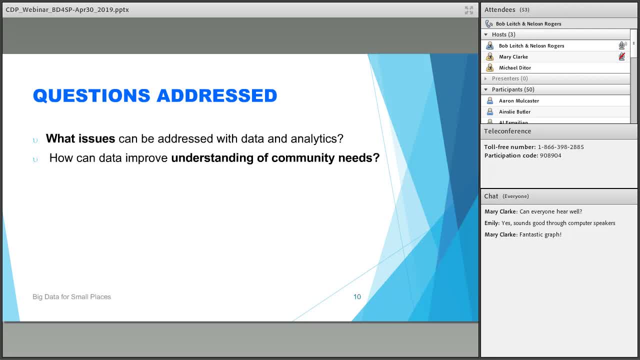 with a survey or with interviews or with focus groups and, and particularly, probe an issue and see what comes up with that. with that. so, anyway, we have five approaches to assessing community need and some guidelines for picking an approach that is most appropriate and then using that as a framework for understanding. 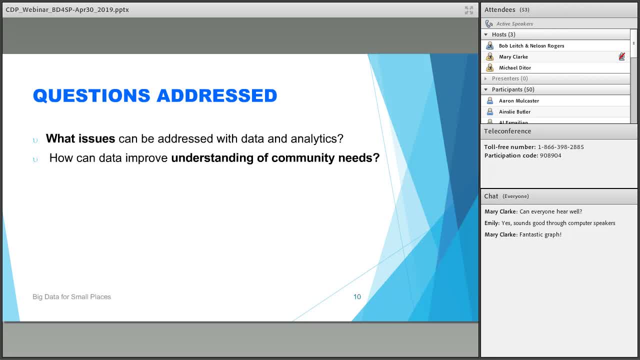 what data do you need to verify that and how would you communicate the results of your findings? that's just an example of one of the modules we're probably repeating ourselves here, because we, of course, also try to make sure that people know where to find relevant data- reliable should probably be there as well: reliable, relevant data. 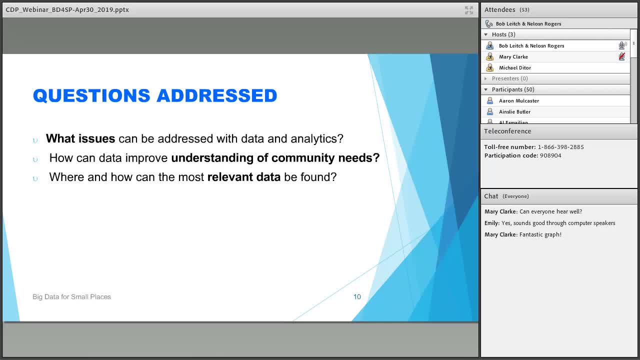 uh, and that's sometimes a mystery, depending on the pean, the, the teams, uh, some of the um working groups, uh, might have someone on their group that's got some expertise here, but some, many of them, do not, and they simply are not aware of where they can go. there's usually the obvious places they can. 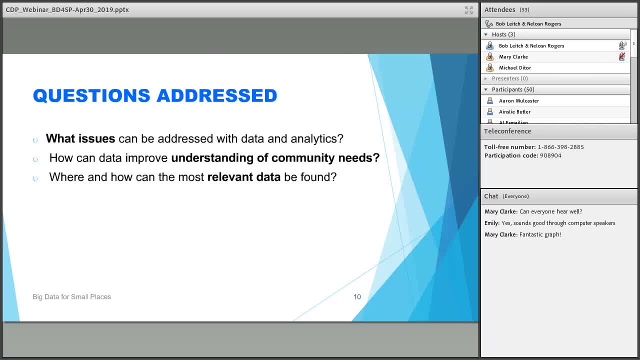 go like stats canada. but there are so many other good, reliable sources, as i'm sure you all know, uh being part of the community data program, uh, and we would not know exactly where. so with that i'd like to close now. um, there are some other good, reliable sources, as i'm sure you all know, uh being part of the community data program. 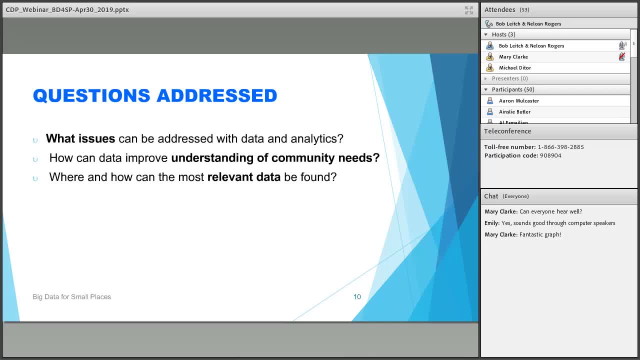 but, um, there are so many other good, reliable sources, as i'm sure you all know, uh, being part of the community data program, being part of the community data program, but when we meet with municipalities, particularly in small rural areas or community-based organizations and rural areas, many of them don't do not have that capacity, that understanding and 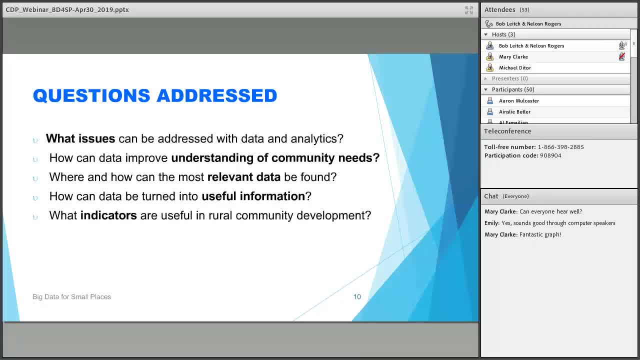 then how can you turn it into useful information? some of these points are: we've talked about a bit already and what indicators are useful in a rural community development. we find that some of the indicator systems that are out there we can. we can use some examples of this. there's one that the Ontario 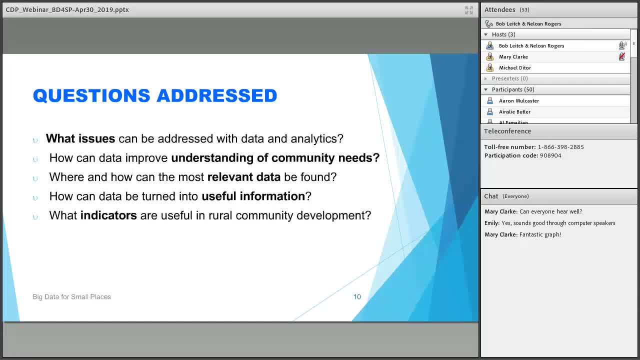 Ministry of Agriculture, Food and Rural Affairs has- that's on me, I forget the name of it now- the newcomer and youth community indicators, that's. that system has been mothballed because of one of the really important indicators that we've talked about and we've talked about. 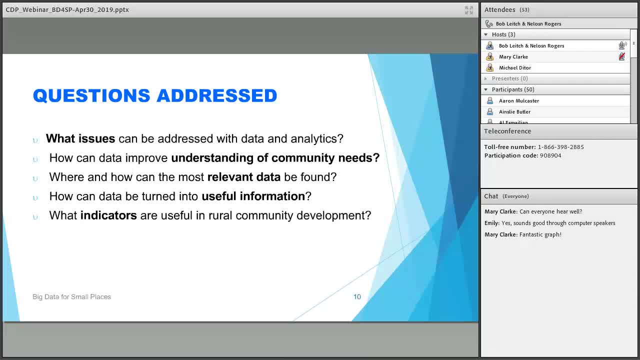 reasons is that the large percentage of the indicators were really developed for urban areas and didn't translate well to rural areas, so that you ended up with these indicator systems and scores that didn't really tell the show the picture of what the community situation was like on the ground. and last point here is that 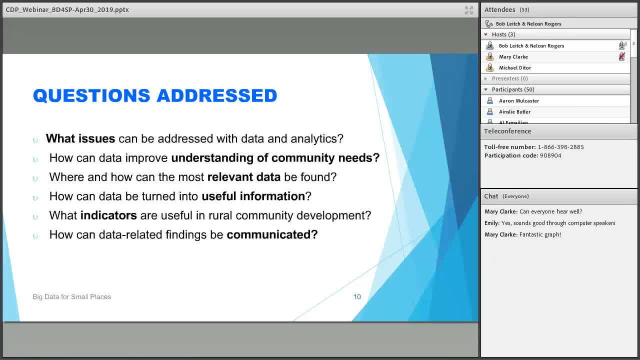 how can you communicate what you find? so the whole notion of visualization of data into charts, maps, graphs etc. is extremely important, and we were just before we started this webinar today. we were on the community data program website and there's a section there talking about taking the data and putting 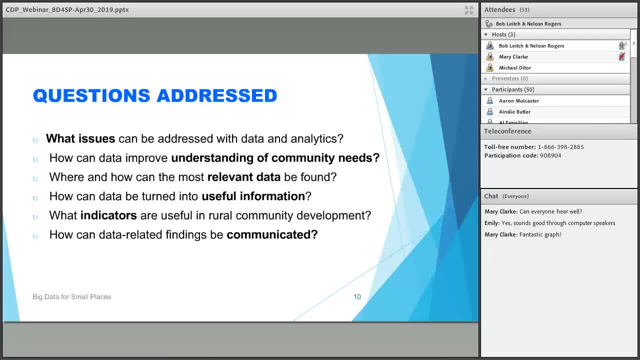 it into a visual format, and so that's what we're talking about here as well. in addition, we talk about communicating at two. each piece is kind of a 1800 per hour, and and it's gonna be for until, but we like to leave them with some general guidelines around clarification. 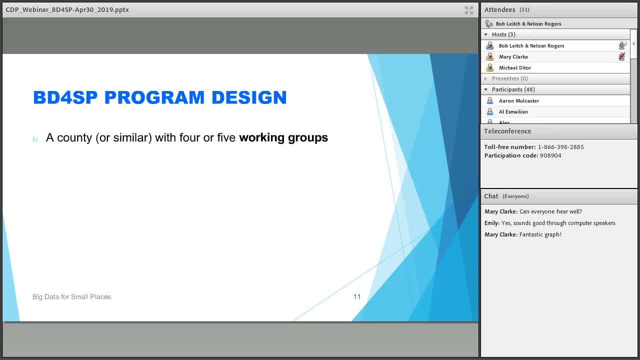 So a little bit about the program design. So I've mentioned previously that we usually have four or five, sometimes six working groups. Often it's within a county, but we also look at geography in what we refer to as the functional community. So we live in the town of Perth, Ontario. 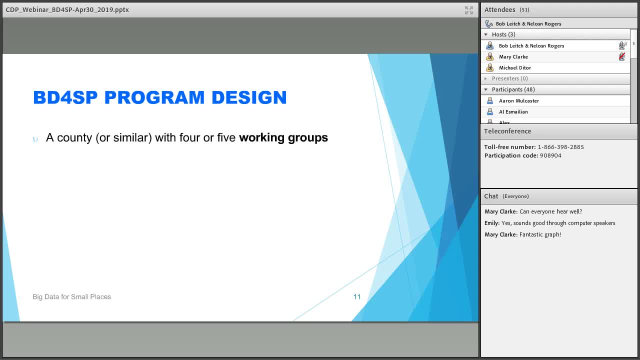 which is midway between Ottawa and Kingston, And if you're familiar with that area, you'd know that when you talk about looking at your community of interest, it may very well be a functional community, not a political boundaries geography community. We want to make sure that people bring a real, practical problem to the table. 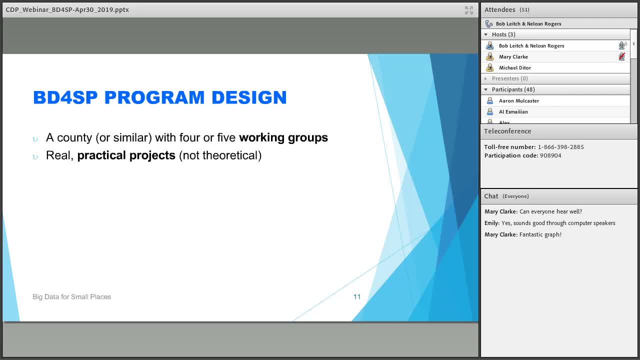 Our experience was with when we first started this program. we had one team who came with a vague idea about what they wanted to do, but it really wasn't something that they were, at that point, trying to resolve or deal with, And so it was more theoretical and hypothetical than practical. 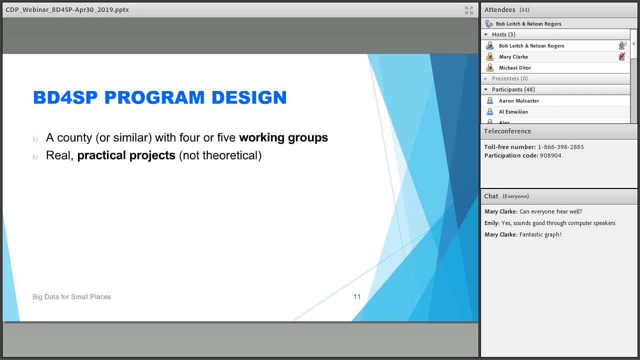 So we really emphasize that it needs to be practical And it's also a selling feature, because the resistance today is: why do I go and participate in this program? I haven't got time, but if you're taking something to that program, this program. 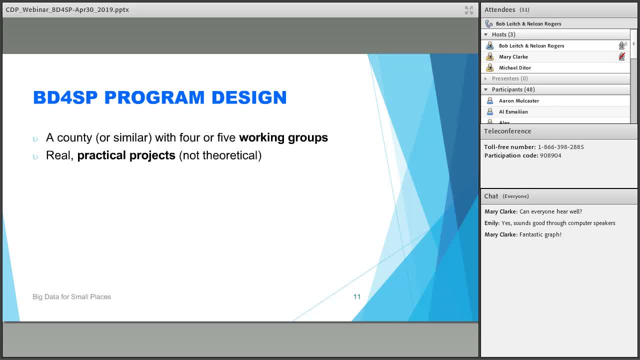 big data for small places you're already working on, and it'll help you accelerate the process of addressing the issues or questions. that then it's actually time on task, as opposed to just simply going to an event that might be interesting but not particularly immediately useful to you. 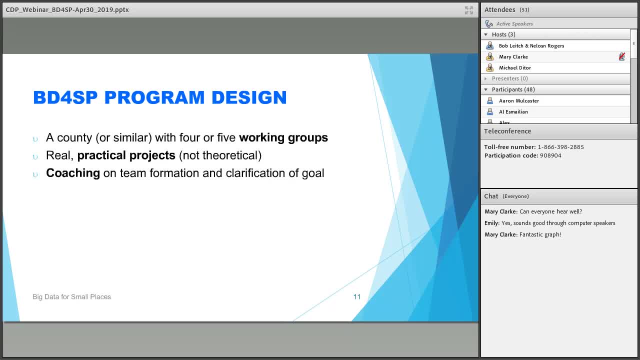 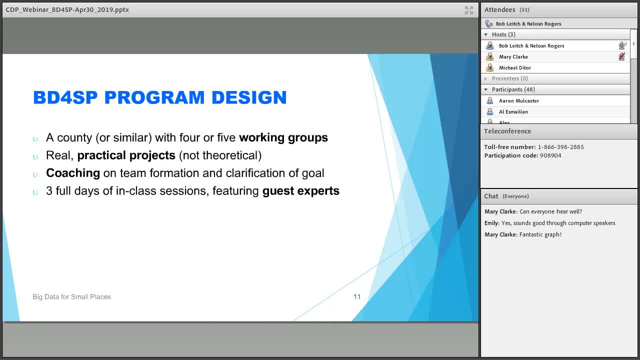 We have the confirmation, the clarification, the goal, And then there's three full days of in-class sessions and we bring in experts. So once we know from our consultation process that we start with that, we know what the areas of focus and the topics. 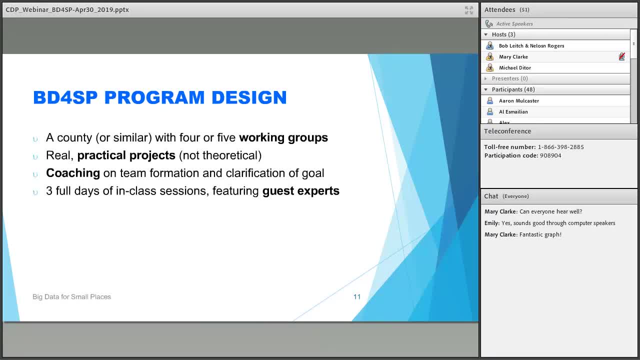 that are going to be dealt with. We try to find guests that are willing to come and speak to the sessions and we've had absolutely no pushback by from this at all, because the people we usually approach already have as their mandate to try and do outreach. 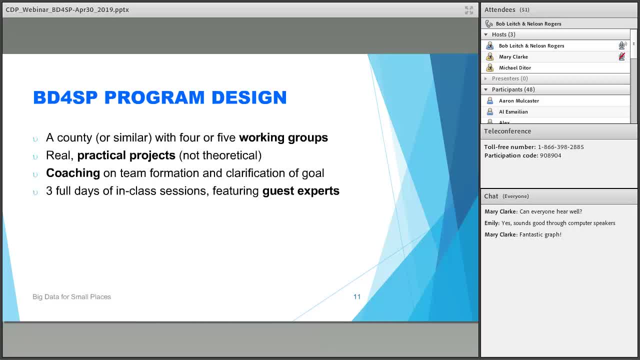 to the kind of questions that are being dealt with. So their expert opinion and their knowledge and experience can be brought to the table and help within the context of applying data to the question. Between the in-class sessions, we do provide not major homework, but we do give. 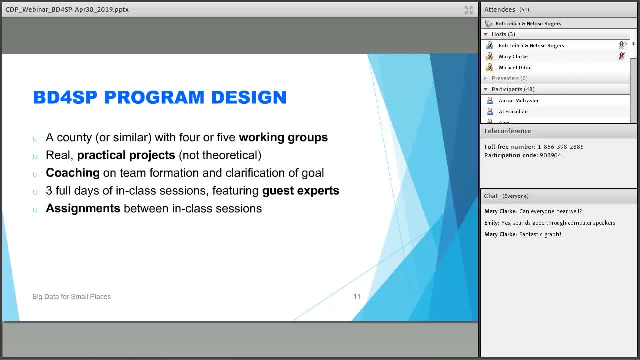 each group assignments so that they go away and they work on what they've learned so far and bring it back to the next in-class session. And we do, and we've developed a very extensive list of other organizations dealing with similar problems or concerns, And they often are ones that people 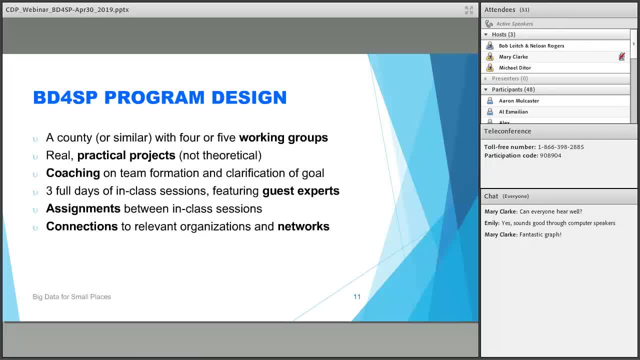 would know, but not always, And we've had some classic examples there where we were dealing not too very long ago with a parks and recreation question And we were able to point the group to other examples and best practices elsewhere that they could use as comparators or to find. 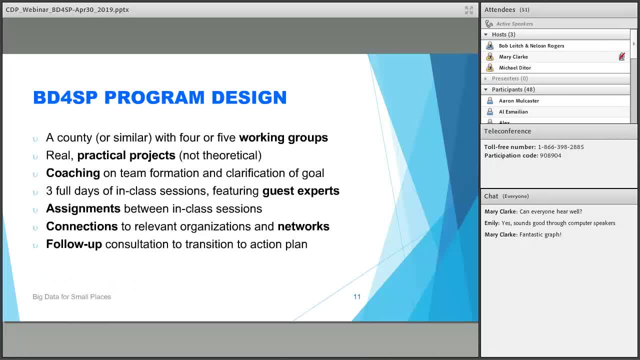 more information and sometimes create a network that they hadn't had before. After we do the inquiry, we do a follow-up consultation. So this is done with each individual group, not as a whole, And that's on purpose, because we then try to help that team who have come up with an action plan. 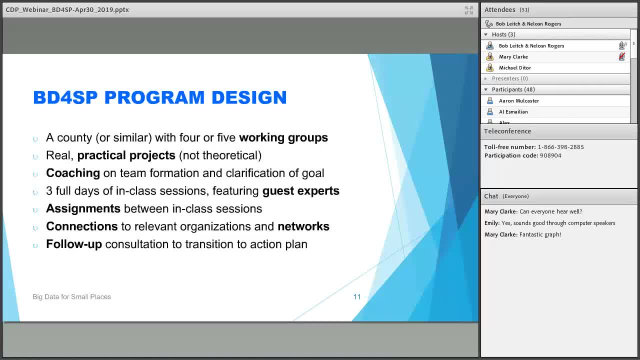 as to how they're going to transition that into, or a plan how they're going to transition that into action. So that's an important step and maybe further consultation is required or further information is required. So we learn that And then we do a follow-up consultation with each. 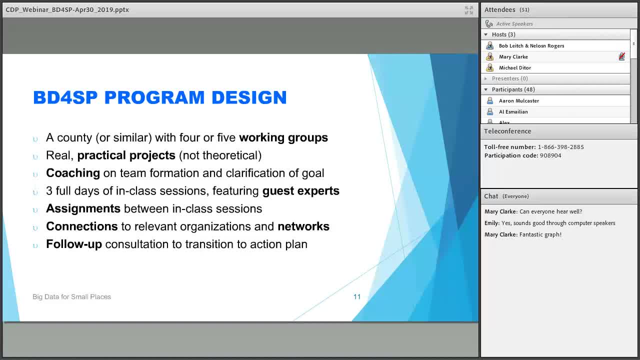 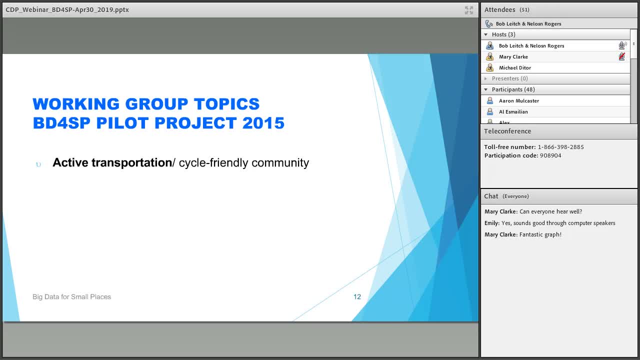 other, And that's still a fun way to achieve a much better outcome. who wants to do a pitch, a presentation with a which they want? So here are some examples of some topics that were the focus of working groups in our pilot project in 2015.. So the active transportation group- and that's an interesting example of the 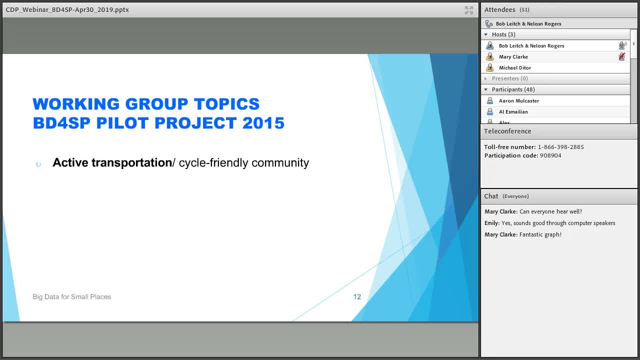 kind of final approach, because the group, the municipality, had produced a transportation master plan that covered absolutely everything fromvarious platform. Are you gonna open up a Thank you, Apologies, Are you good today And I'm good Be my guest? 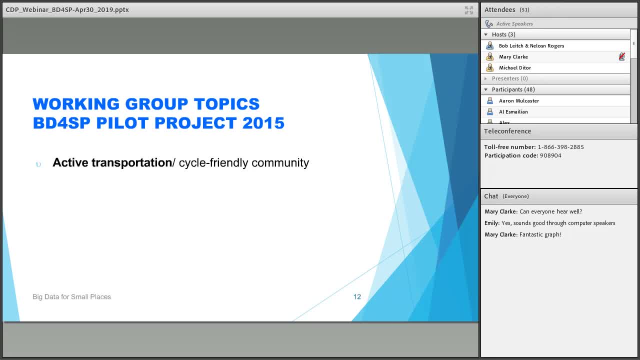 All right, That's all right If you have questions. Thanks Okay, mem. Well, thanks again, Bye, bye from roads and bridges to commuters, to sidewalks and a lot of different things, And this working group wanted to do something. 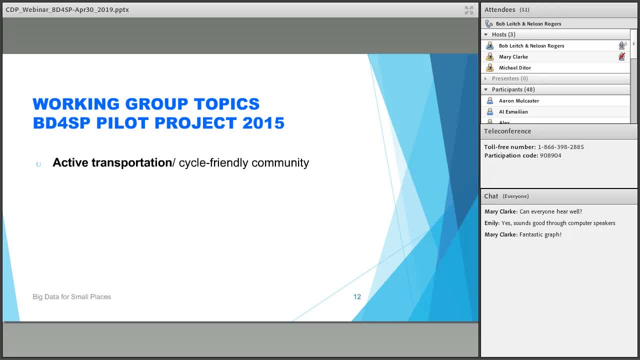 specifically around active transportation And we helped them work through clarifying their goals, setting achievable goals, targeting some visible results, targeting results that would be stepping stones to larger goals And by the end of the program, they focused on getting a designation as a cycle-friendly community. 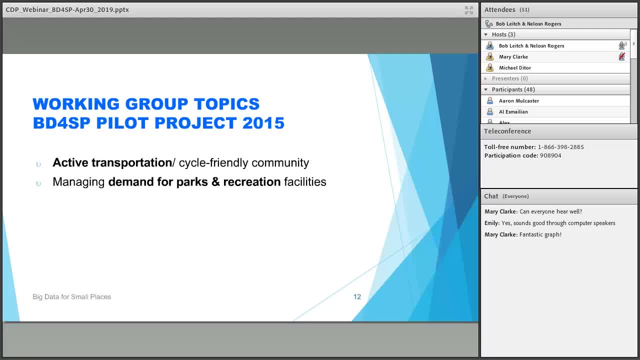 So going from a very broad general interest in transportation to a very specific outcome was part of their process. And then Bob alluded to this one, the managing demand for parks and recreation. And this was in a small community that was growing and their historic figures didn't really predict. 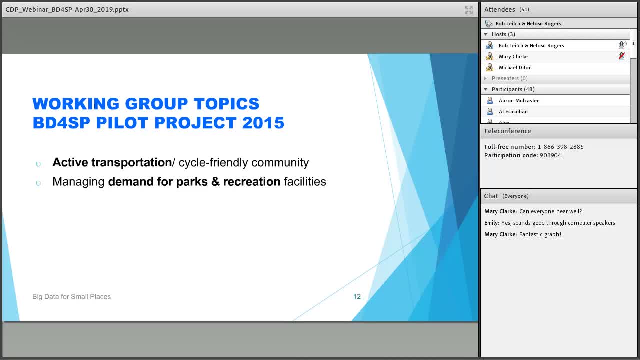 what their future demand would be And they were trying to work around that And we put them in touch with some province-wide groups that were researching trends in parks and recreation demand And we also were able to connect them with some resources around getting a better handle on their own record keeping. 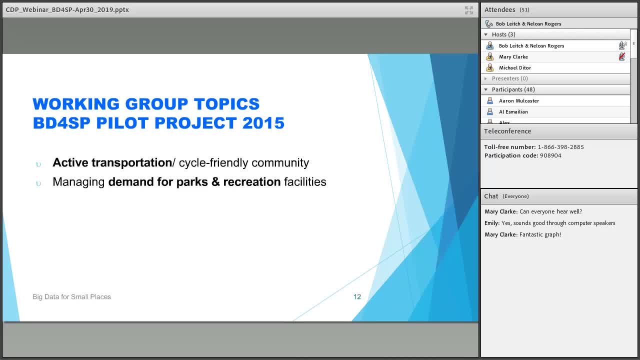 and their own internal data so they could use it more readily for planning purposes. That group told us that they cut their consulting budget in half After they participated in the Big Data for Small Places program because they realized there was so much they could do internally. 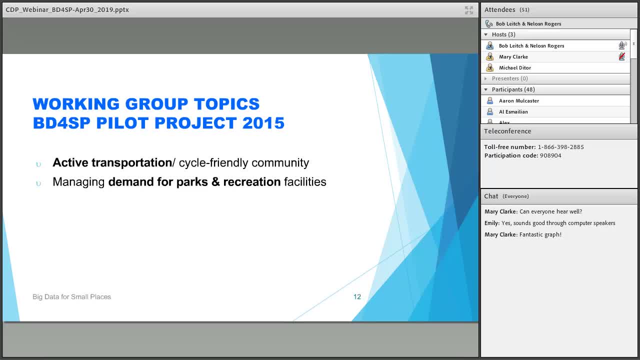 by building their own data literacy skills and so much free resources they could obtain from other networks that they could really reduce the get better results with fewer consultants. So that was a success for us. Yes, we had another one around indicators of mental health. 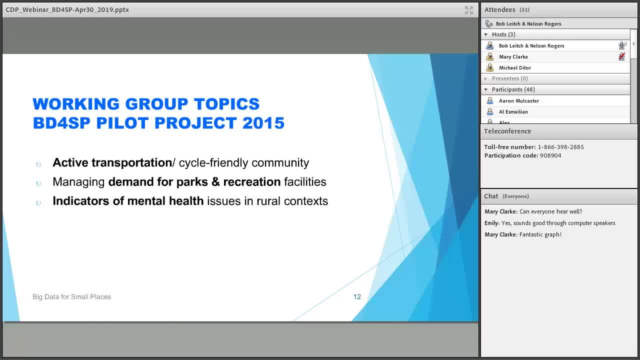 and mental health related. Yes, we had another one around indicators of mental health related issues that were particularly appropriate to a certain geography that this social service agency was working with. Then we had one around community attractiveness, and that was. it started out as an immigration program. 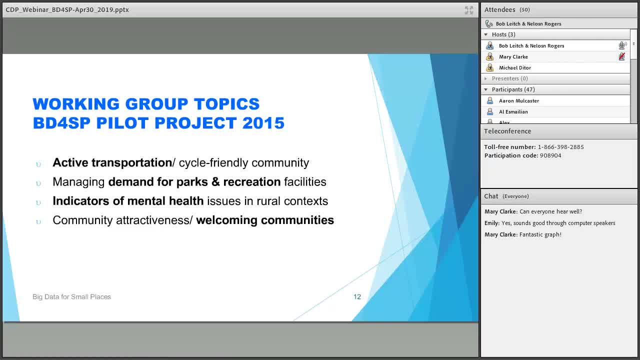 but ended up being more focused on secondary immigration. And it's here. if you're working in rural areas, you often know that people come from other countries, come to Canada and they come to the big cities And then, after they've kind of settled in, 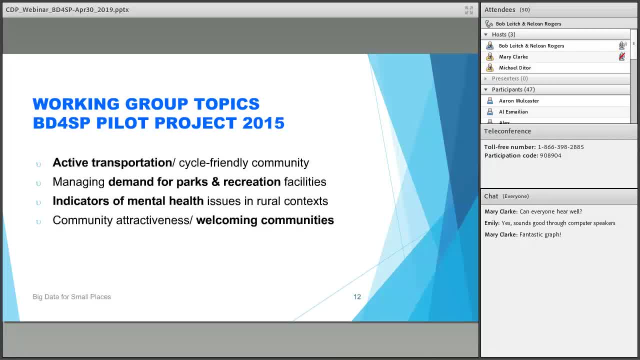 and found their place in their career or whatever. then they're more interested in relocating to a rural or small town area And we looked at some ways of indicators of welcoming communities that would facilitate secondary immigration to rural areas. And then another one on well-being of children and youth. 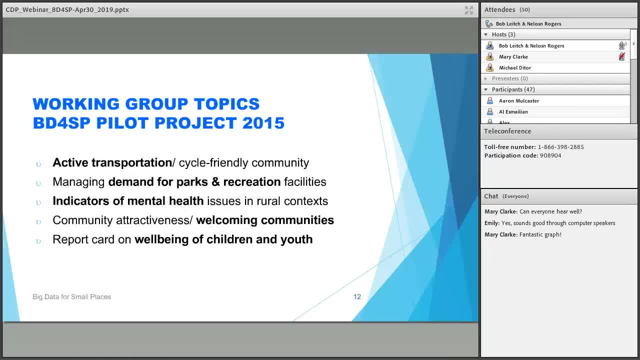 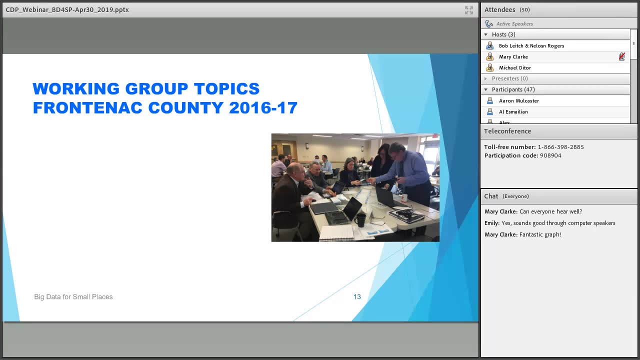 and some indicators of well-being. So they started off with some pretty broad topics and ended up with some fairly concrete action plans as a result of the program In our more recent group, just for example of the kinds of things that were dealt with. 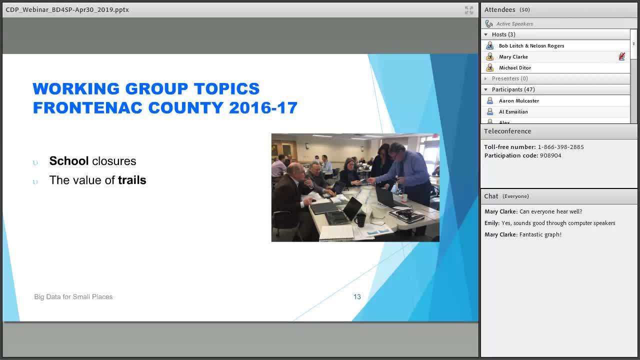 the working groups work with school closures and work particularly on: what are the? how you measure the impacts on a community of the value of having a school or losing a school and what are the related factors? The same thing around the value of trails. There's been a lot of trail development in Eastern Ontario. 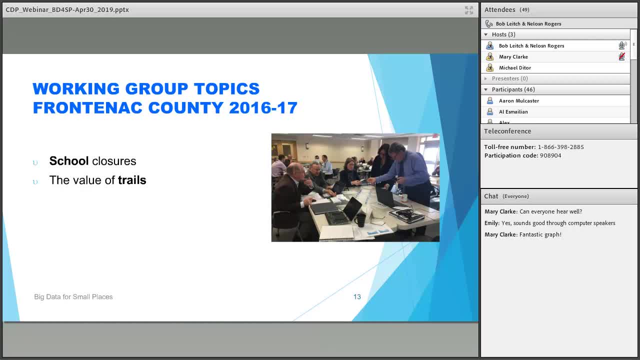 both hiking trails and trails for motorized vehicles, ATVs and so on, And how do you estimate the value of a trail to make a reasonable decision on the cost benefit of investment in trails and its impacts on the attractiveness and the well-being of the community? 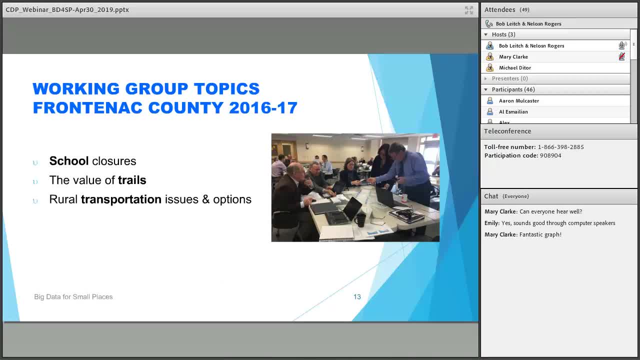 We looked at some rural transportation issues and options and some of the groups came to the table wanting to talk about commuters and commuting to work. But the rural transportation issues are much more complex than that, where you have people that need transportation for medical reasons, for social service reasons, 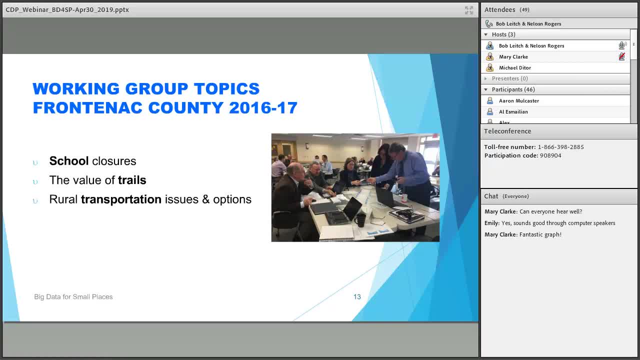 for retail reasons, for recreation reasons and need to look at the breadth of service to the entire community in the area. And then this was an interesting one. It seems rather technical Compared to some of the other ones, but it was communal services around shared water. 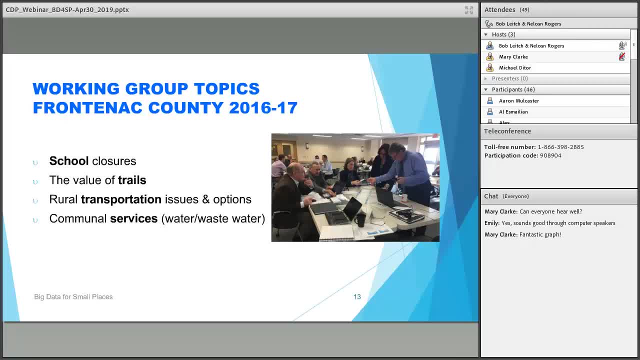 and wastewater facilities, typically for six to 24 homes, typically adjacent to a village that does not have municipal services. And again, looking at the impacts of setting up a communal service system and what that means for not just the population and the real estate assessment value of the village. 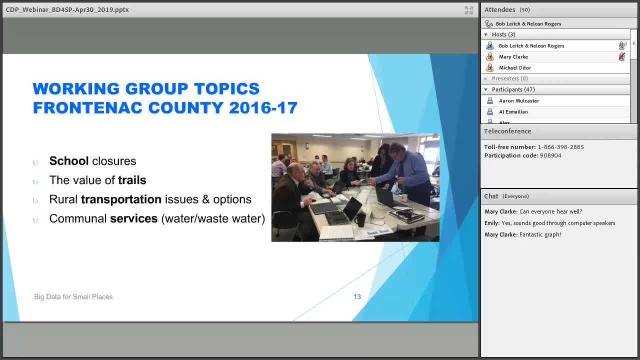 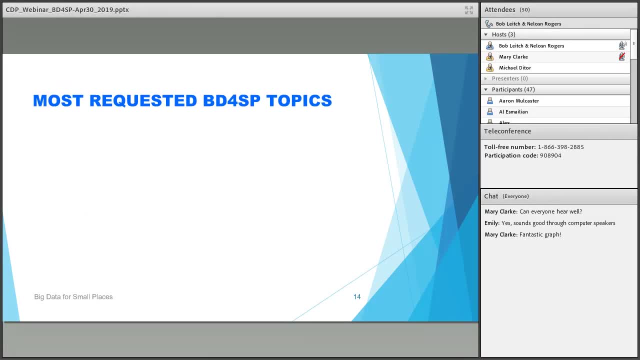 but other spin-off benefits to the village where it can have impacts for the schools and for the availability of volunteers and so on. There are lots of impacts of what seems to be a rather technical issue. So these are some of the more recent topics that again. 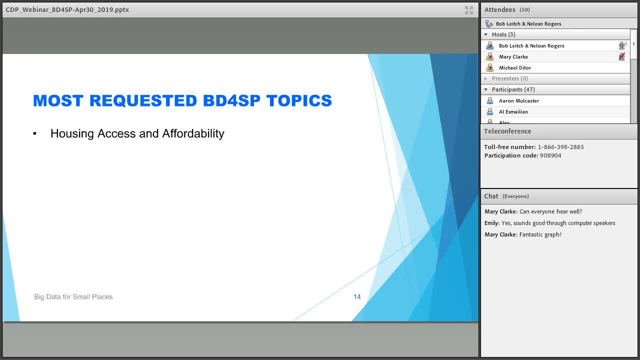 these topics, of course, have been around before, but they are ones that have become more prevalent more recently, and certainly in our region, And so these are some of the new ones that we've discovered. Yes, well, these are just topics that have come to us. 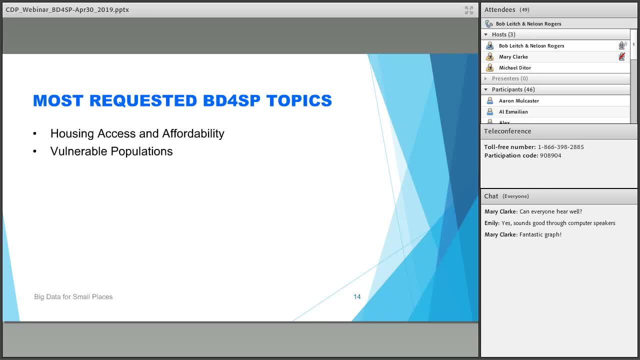 for consideration with housing access, lots of housing issues, and then our portability in the broadest sense- not just meeting some of the technical definitions of portability- and some work with vulnerable populations and, in different ways, vulnerable due to economic, social, medical issues, age-friendly communities. 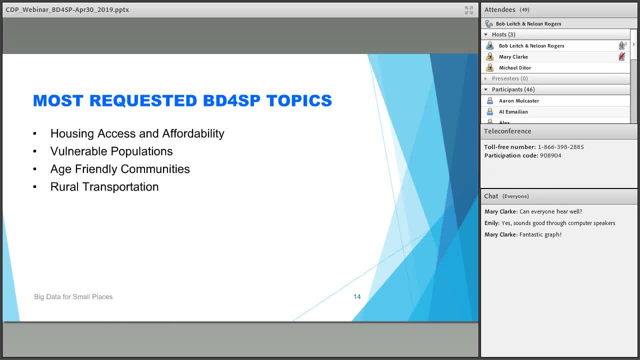 and communities that support aging in place. We've had different kinds of questions around rural transportation, rural broadband and some of the things that we've been able to address, And I think that's been a more recent one that's come back on the table again. 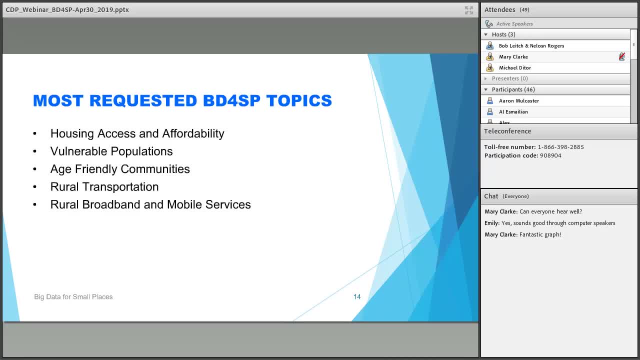 There have been some initiatives on this field that have made some progress in some areas, but we work in areas of complicated geography and sparse population and where rural broadband is still difficult to access, And so we're looking at some of the things that we've been able. 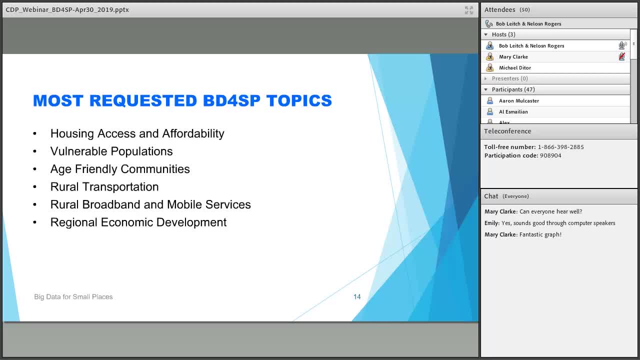 to address. And then I think there's been some questions around economic development, and particularly economic development around functional communities rather than just by municipal boundary, and some things around health services. There's quite a number of things that have come to us lately. Social planning, value for service. 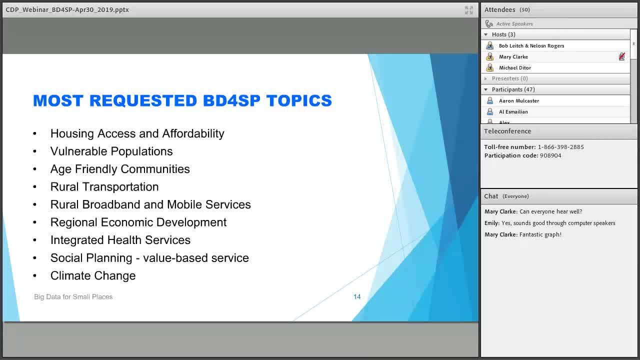 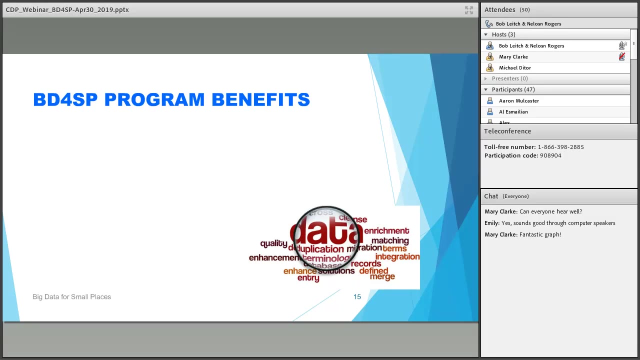 and those questions have come up. We're just close to where we live. We're experiencing an unusual, record-breaking flood season and it seems to be climate change related, And we're looking at issues around climate change preparation and mitigation adaptation. So probably you could almost draw your own conclusions. 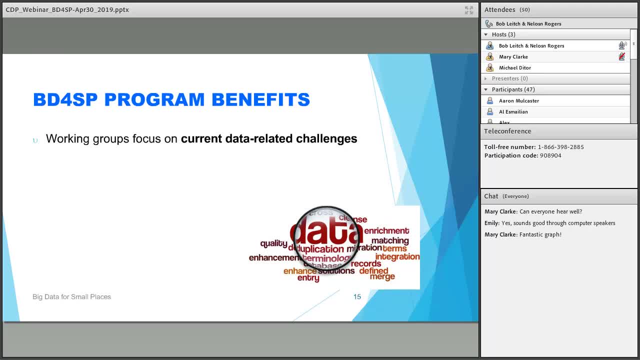 and assumptions about what the benefits of this program are, and especially those of you who work in this field as much as you do- And I'm on the survey at the beginning of the program- Over 80% of you are working with data all the time. 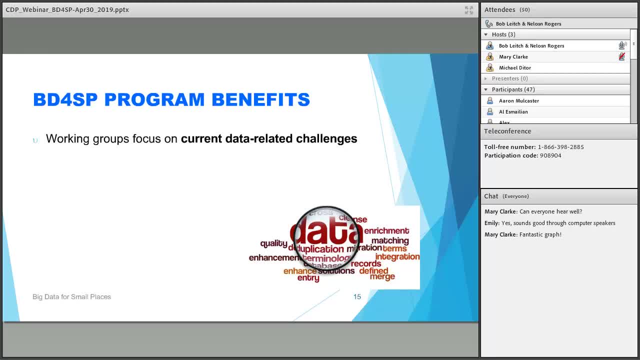 But we feel that the working group focus on current data-related challenges really helps them get their minds around the potential that data has in resolving their issues. We're obviously. I have a question. I'm just going to go to the next slide. I'm just going to go to the next slide. 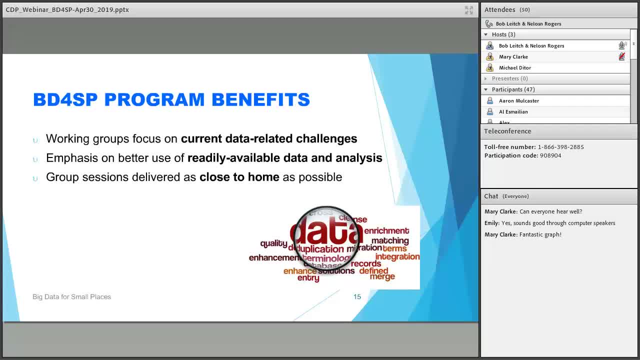 and I'll let you go through the next slide- And I think it's a good idea And I think that's a good idea. So we're really emphasizing the better use and readily available data and analysis And we try to run the sessions as close to home as possible. 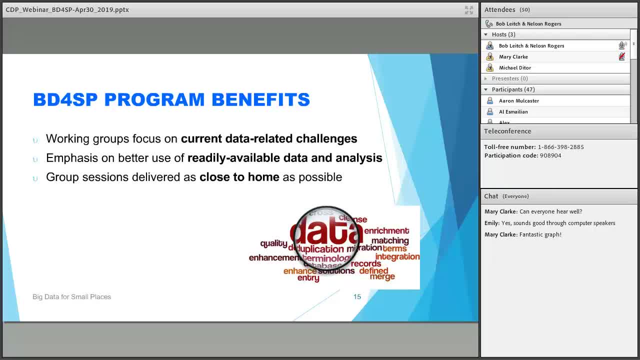 I mentioned about us having an online version at some point. That would allow us to do more outreach across the country and we're hoping that we may be able to work with community data program in the future. The combination of in-person and online. 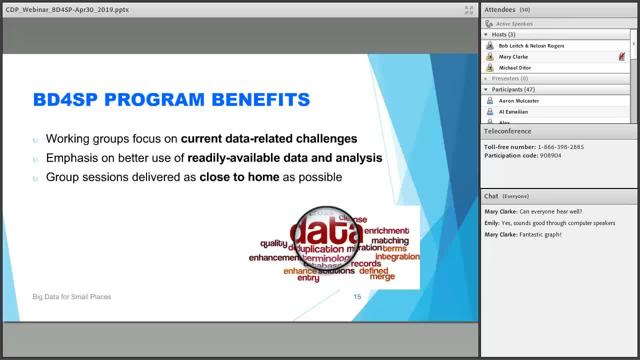 we think there needs to be a balanced in-person and we think there needs to be a balanced in-person, and we think that there needs to be a balanced in-person and we think that there needs to be a balanced in-person is always good, particularly in the consultation sessions. 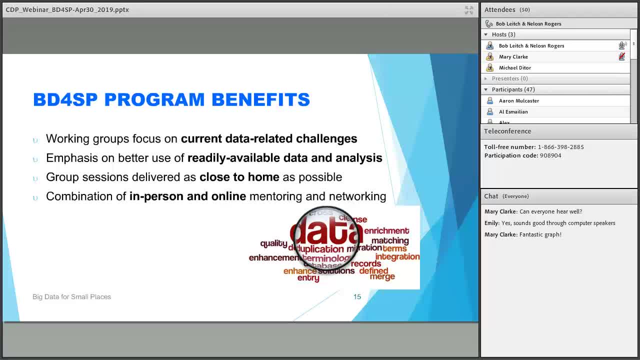 But I could see us taking a good deal of what we've done in our workbook, that we've written- and we're working on a facilitator's manual as well- that those could be, of course, used online, And then exposure to experts in the relevant fields. 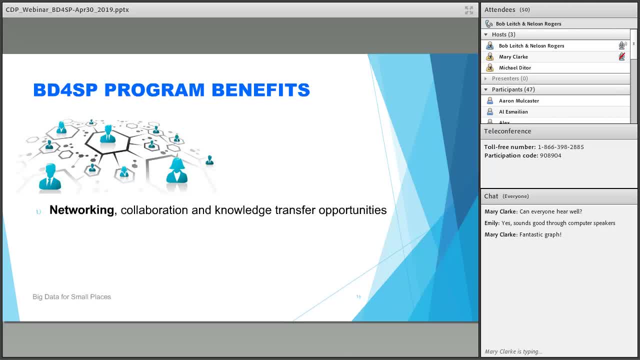 Of course, we mentioned networking before, but we did the follow-up evaluations to each session that we've done and the one that came back very strong was the opportunity for networking and collaboration that resulted by having people in the room that were doing similar things. 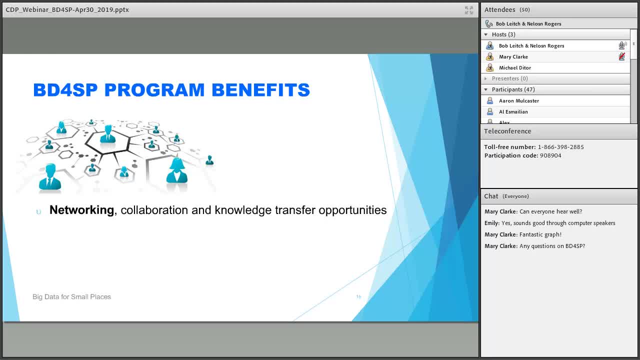 Sometimes not just the topic, but rather the challenges and where they were finding the data, how they were using data, how they were visualizing it, even if the topics were different. And then, of course, the networking with other people in other places. 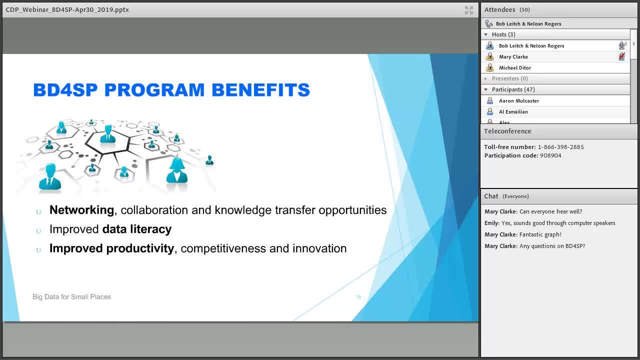 Improving data literacy productivity. This is a particularly important one because certainly in Ontario, but I'm sure elsewhere, the pressure on Particularly in Canada, Particularly in municipalities and community-based organizations to do more with less- Unfortunately that seems to be the trend. but by improving the productivity of your 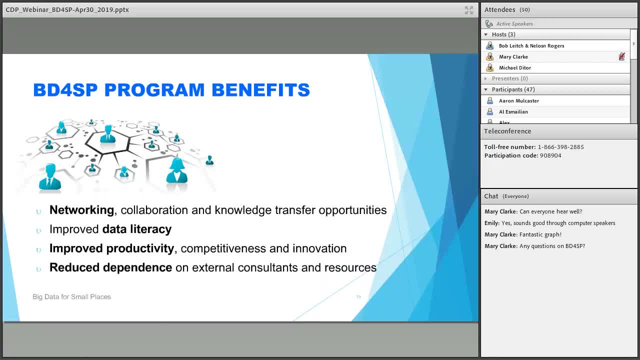 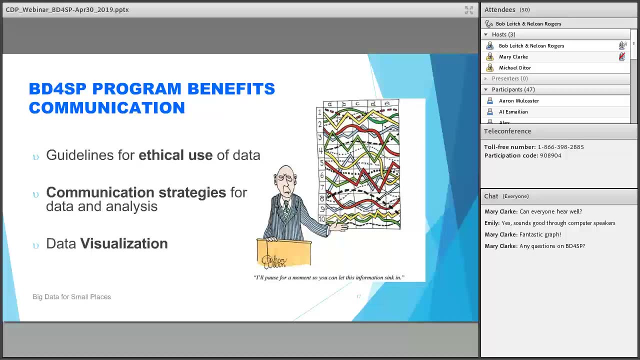 use of data sometimes can help resolve some of that And reducing dependency on external consultants. we saw evidence of that over and over again. We also touch on the guidelines for ethical use- Ethical use of data. Those of you who work with data know that at a certain point you have to be careful. 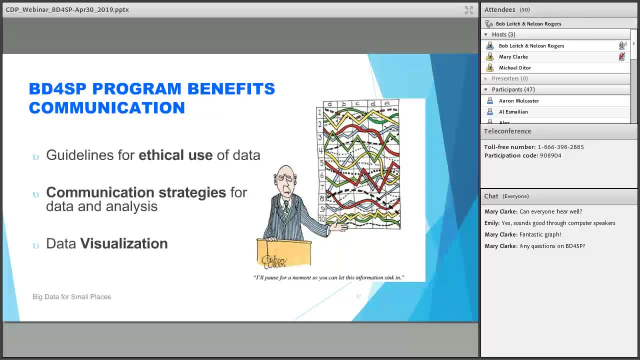 about how you extract particularly personal data, and the smaller the numbers, the more difficult and challenging this becomes. So we do talk about this, and guidelines for ethical use of data is part of our program. Communication strategies: How do you communicate most effectively in data visualization? 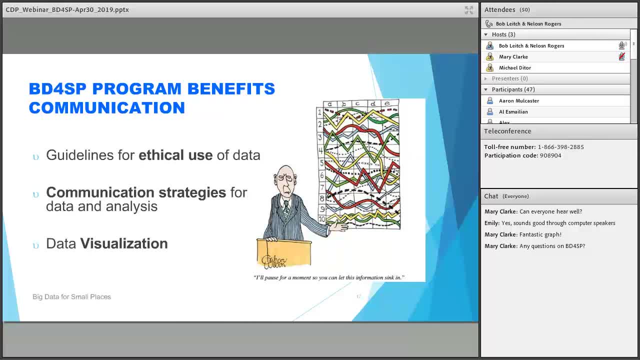 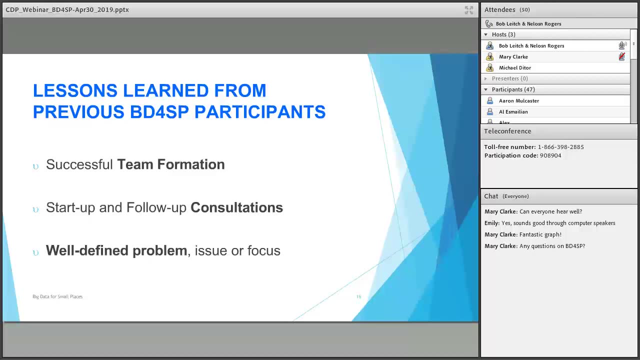 In fact, we had a video That we were going to use today, but unfortunately it's too long, We decided to put it. We can send you the link to it on data visualization that you might find interesting. And these are the lessons learned. 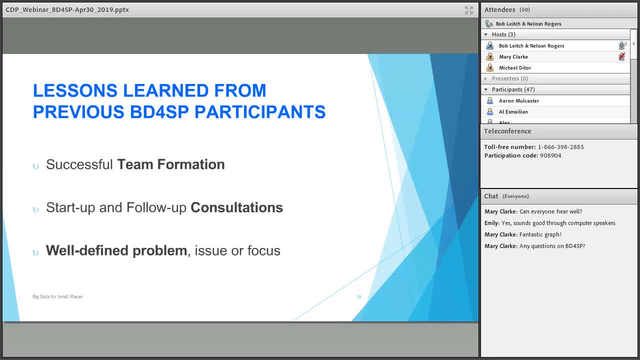 Team formation was really, really positive. That was really a major part of the success of the startup, and follow-up consultations Really helped people get focused In the beginning and to find results at the end and take them forward And then to have a well-defined program. 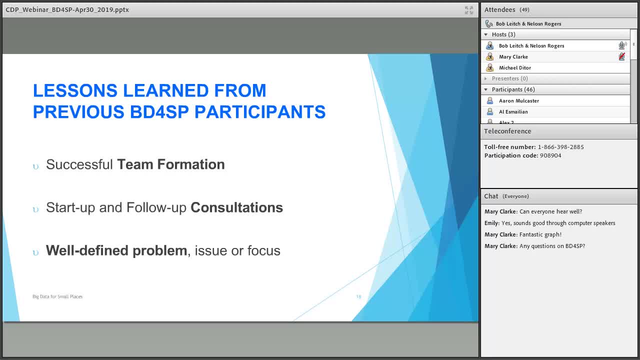 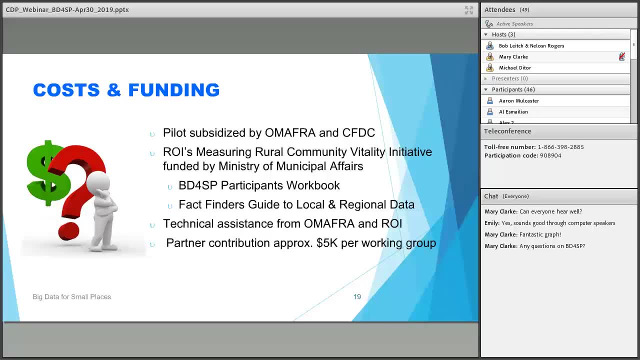 Those are the three most important feedback items we got from our participants in the sessions we've run Yeah. So we always get questions about what does it cost And the pilot that worked out the Yeah. The design and testing of this program was heavily subsidized by OMAPRA through the Rural 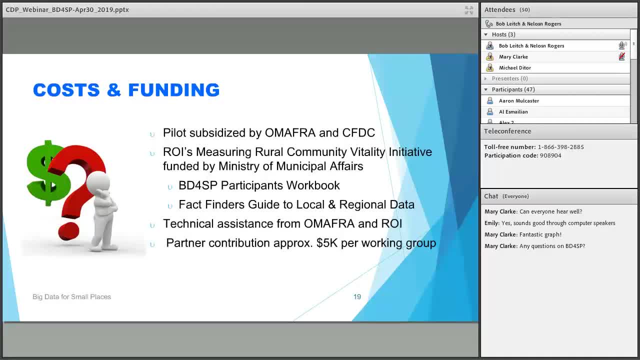 Economic Development Capacity Building Program and by our local Community Futures Development Corporation. Then the workbook and the research that went into producing the workbook, and if you download the workbook from the Rural Ontario Institute website, the link's in it for further information, additional resources. 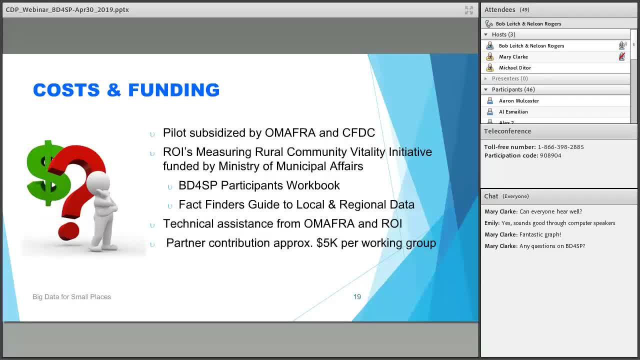 Those are live links built into the workbook And all of that research and development that was paid for by the Ontario Ministry of Municipal Affairs through the Measuring Rural Community Vitality Initiative. A companion volume was also produced under that same program and some of you may know. 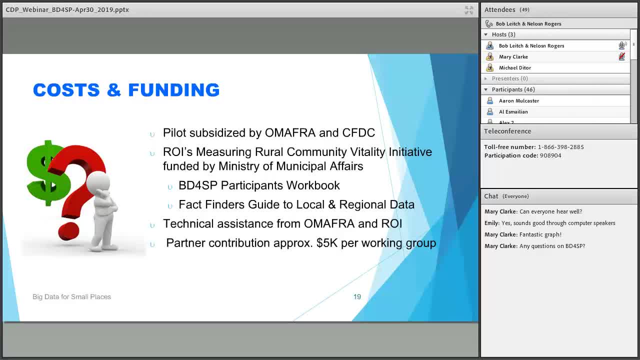 the name. Ray Bollman, who was head of Rural Statistics at Statistics Canada for many years, now works as semi-retired like us and works part-time with Rural Ontario Institute and has developed this guidebook. I refer to it as Yellow Pages for Rural Data, but it's a guidebook for how to find data. 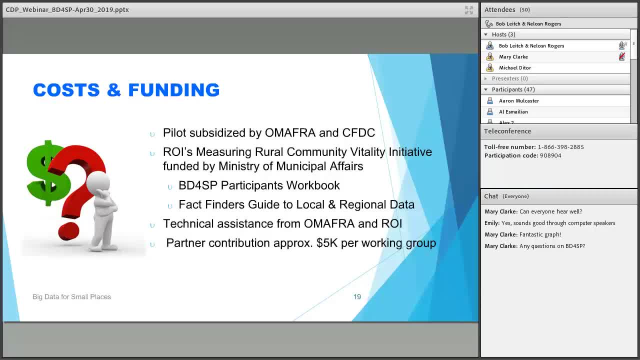 on local issues And that was also funded under the same program. we worked on the development of those together. Now there's lots of value in that. Yeah, There's lots of variables in how much this program costs to deliver, but we generally 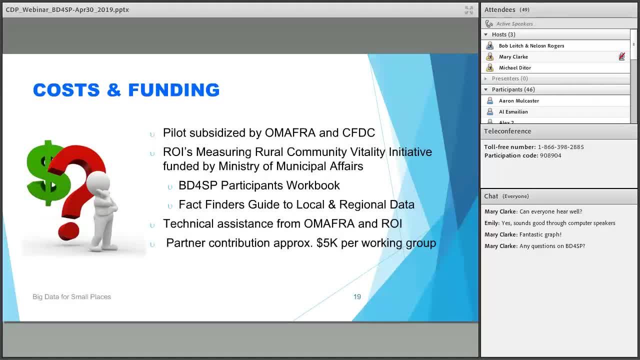 find that the costs work out to be about $5,000 per working group. but some cases there's because of the nature of the program. there's subsidies available or we'll find a community group that donates space and technical support- different things, so the prices can be quite. 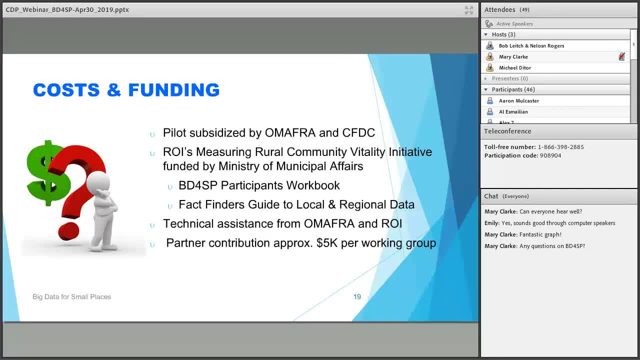 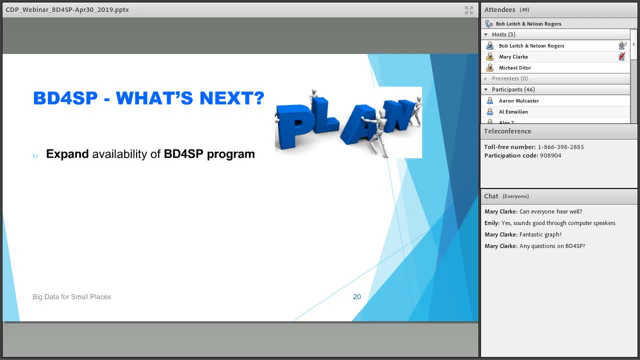 variable, but that's just kind of a ballpark difference. Okay, So we're looking at expanding the availability of the program and we have sketched out a concept for a facilitator's guide and a facilitator mentoring program. We have applied for funding to support that. 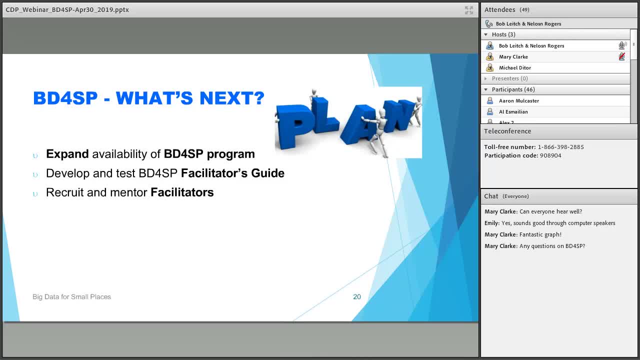 That's been unsuccessful so far. but we have had. we have a list of people that have come out of the woodwork, that have said that as soon as the facilitator program is ready to go, they'd like to be, they'd like to participate in it, and we think that this is really the 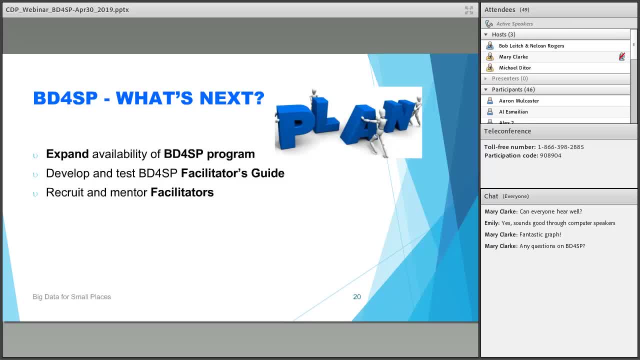 way this needs to go in capacity building and that local groups and local organizations should have their own in-house facilitator that can work a group through the Big Data for Small Places process, and we would be available as resource people and as mentors, but we wouldn't need to be directly involved in the delivery of this program. 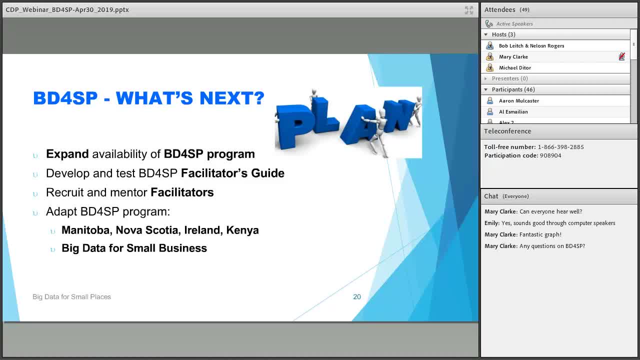 And we've had inquiries from this from quite a number of areas, from different groups in Manitoba and Nova Scotia, Ireland, Kenya, Norway, other places, and we've had a number of requests. We've had requests around a specific version of this in Big Data for Small Business and 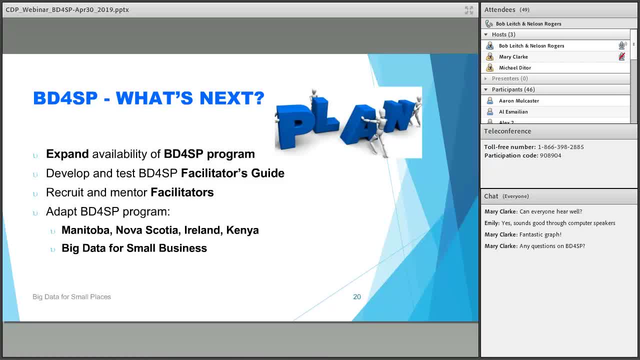 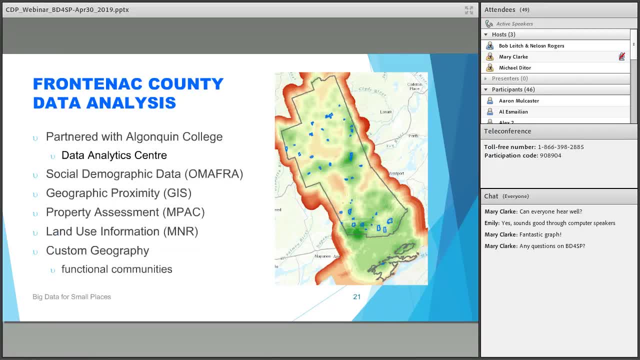 we've sketched out a format of concept paper around what that might look like and what kind of partnerships we'd need to bring that forward. So we've got lots on the table of what we'd like to do in the future and we think that. 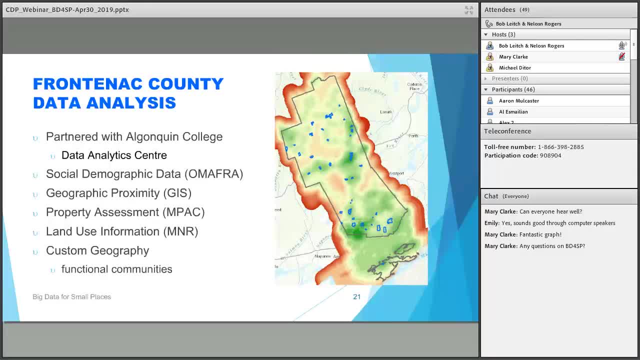 working with the community data program may very well be a good step toward that. We're going to probably come back. we're going to come back to an example when we talk about the next session section of our presentation today on data analytics for rural transformation. 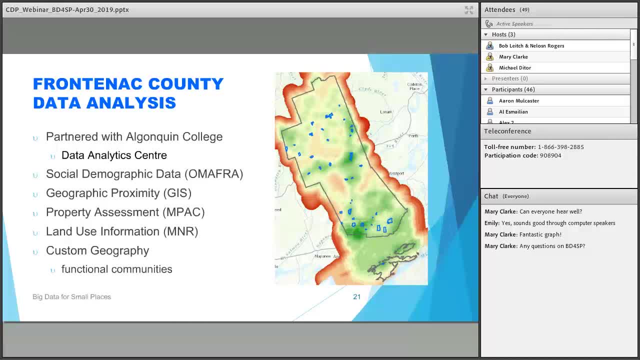 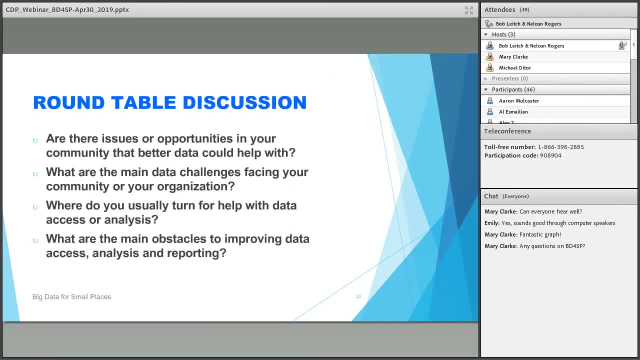 We're going to talk about some of these factors that are here that you see under the Frontenac County data analysis. So I think we'll just skip ahead because we don't want to run out of time. So we had some questions for you, but I'm going to stop there, Mary, if you want to. 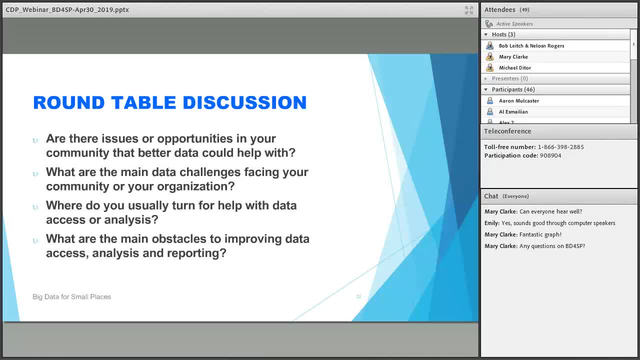 pick it up? Sure, Yeah. Do you want me to switch over to the other presentation now? Yeah, So the question is: do you want to take any questions on this program first, or do you want to just do them both and then do the whole thing? 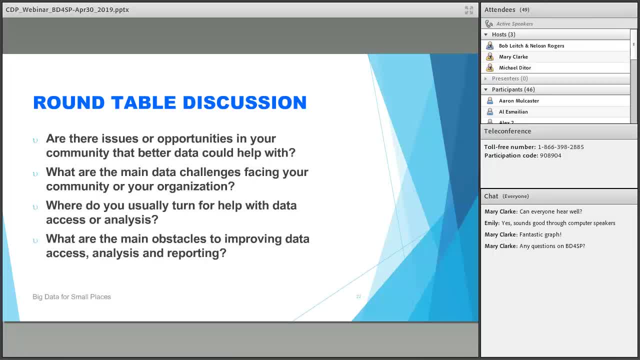 Well, there's no questions right now in the chat box, so I would say: let's keep going and then we can always come back to this during the questions, because we're almost at. I'm doing time conversion in my head: we're almost at 2 o'clock. 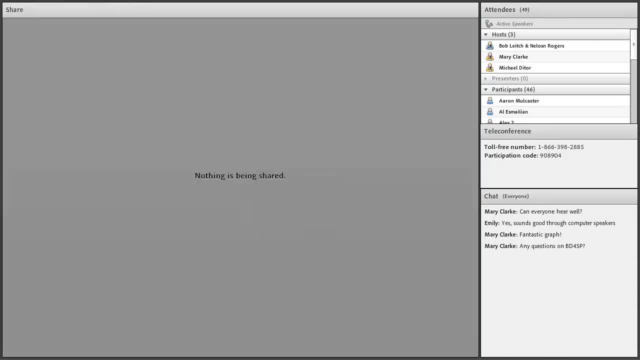 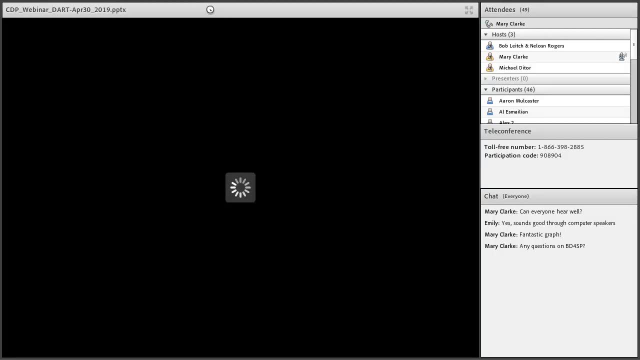 So that's fine, Let's get going, because I do want to get through the next part of your presentation, Okay, Okay. So give me one second. everybody I'm going to bring up, As we said, this is actually two distinct projects that certainly work very closely. 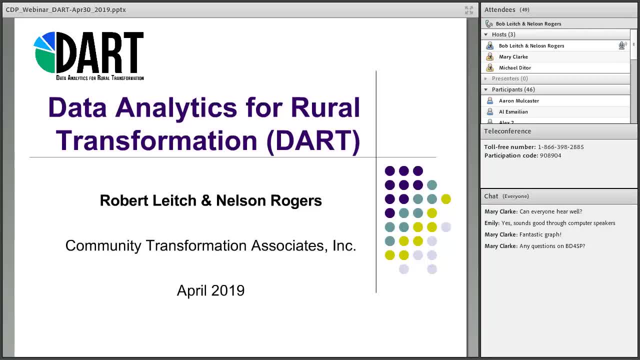 related to each other, but this is the second part of it. Yeah, We'll quickly make the linkage between the two. So, all of the work we've done with Big Data for Small Places and our hands-on in the in-person work with community groups, what became apparent was that there was something. 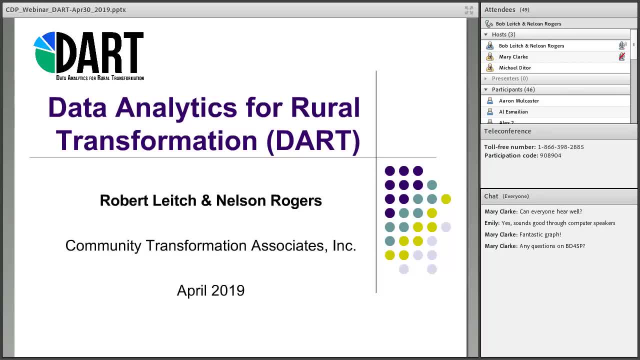 else missing, And that was a tool that would allow for collecting, analyzing and visualizing data, And that's so. what has happened is that we have developed this program called Data Analytics for Rural Transformation, So we're going to walk you through this. 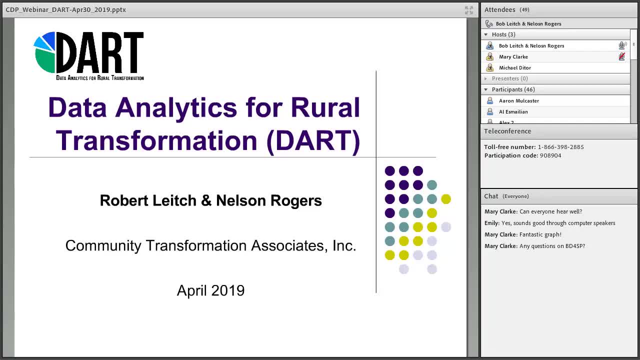 This isn't going to take nearly as long as the Big Data for Small Places presentation, So we should have time for questions at the end. So we have formed a new company. Nelson and I have worked separately, together collaboratively, but worked separately through. 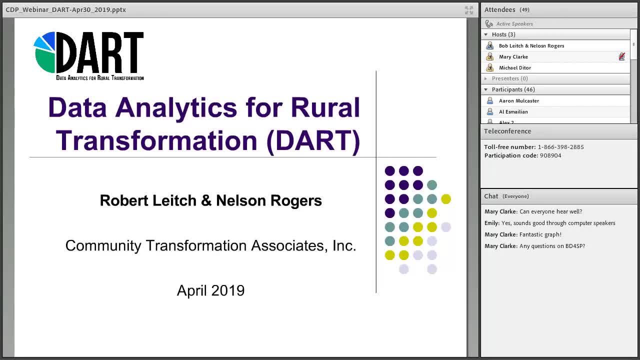 our own personal companies, But more recently we formed Community Transformation Associates And the purpose of that is to have a common place where we'll have the opportunity to collaborate. We'll have our consulting services, but also this DART project and the Big Data for Small. 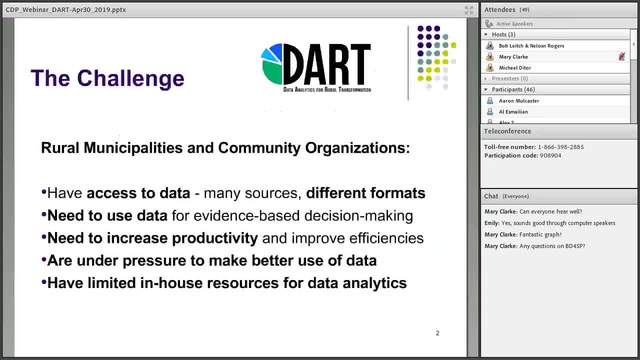 Places, among other things, I expect as time passes. So what we saw was the challenge that we saw in rural municipalities and community organizations, or smaller communities within urban centers, as Mary pointed out to us, And the reality is that they have access to a lot of data from many sources in different 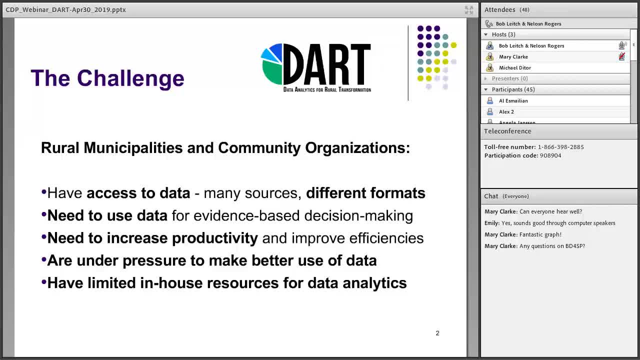 formats, The need to use data, as we've talked earlier about, for evidence-based decision-making in support of their programs and their application for funding or budget. There need to increase productivity and improve efficiencies, And they're under a lot of pressure to use data. 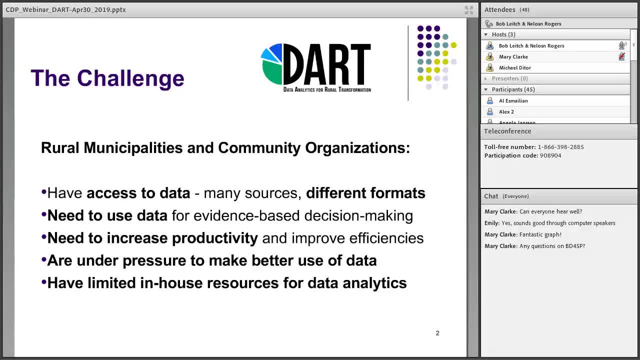 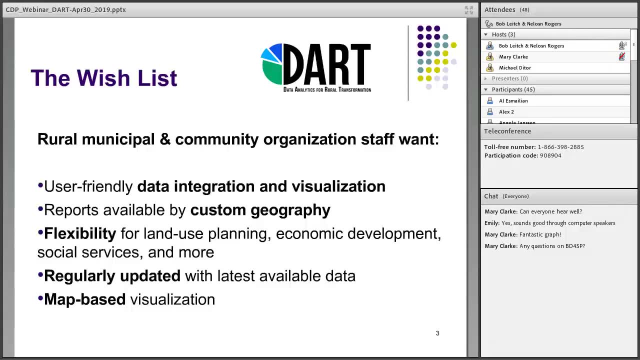 And the data. a pool of data is significant and it's a challenge for many to manage that properly and they have limited in-house resources, some of which we've talked about under big data for small places. When we talked to municipalities and community organizations, they told us they would like to. 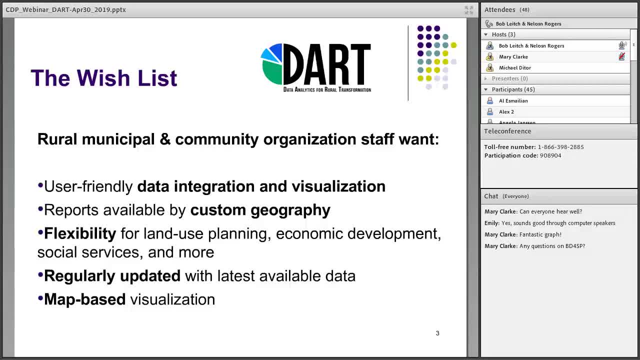 have a user-friendly data integration visualization tool. They wanted to be able to report using custom geography, as opposed to municipal boundaries- Often it was a functional community- was more important to them. They wanted the flexibility to be able to use it for land use planning, economic development, social services and more, and they wanted to be able to access. 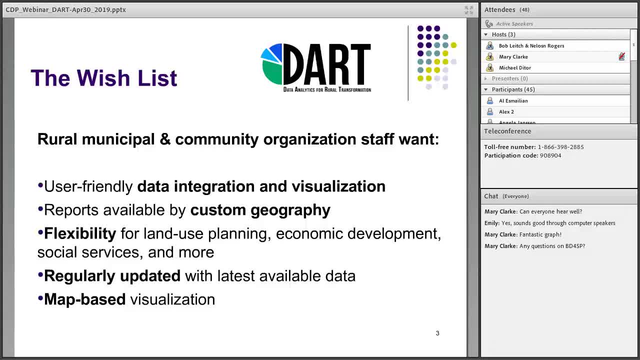 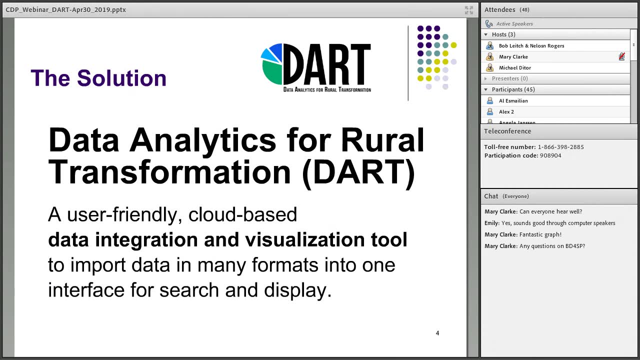 regular updates so that they were current with the data they were using. and surprisingly- maybe not surprisingly- the number one visualization tool that many of them wanted was maps. Not always, but often was So. we created Data Analytics for Rural Transformation- DART. 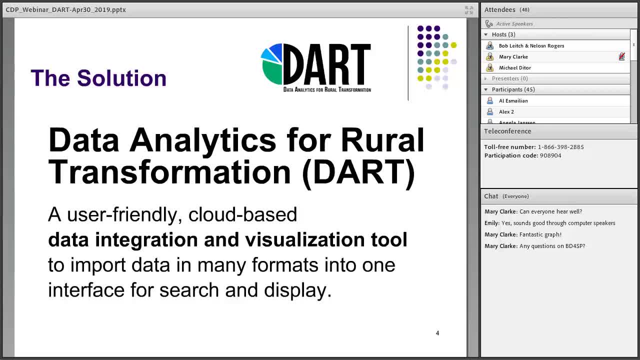 and we describe it as a user-friendly, cloud-based data integration visualization tool to import data from many formats into one interface for search and display. So my common description is: it's like a hard drive. I mean it's much more intuitive to search when you have the device and it's very 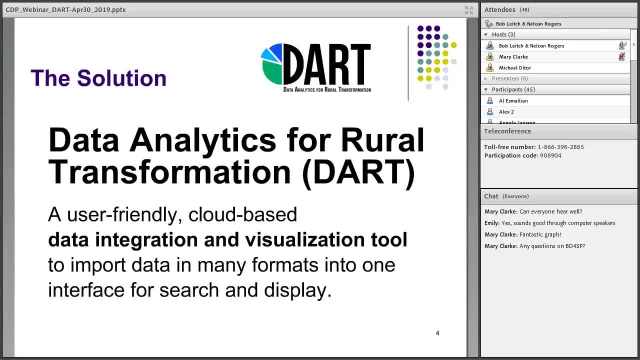 very easy to find and it's very easy to navigate within the browser. Rural Transformation is very, very easy to do. It doesn't take any kind of programming to inventory any kind of data and it's also very easy to figure out where these robots. 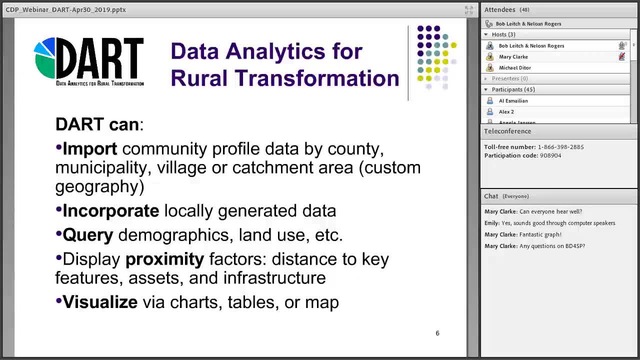 are from, Rural Transformation is a very, very easy tool. We actually started developing it a few years ago. I'd already utilized it from the start and I was like, wow, there's really no way I can do this. I don't know if you've got any experience with it. 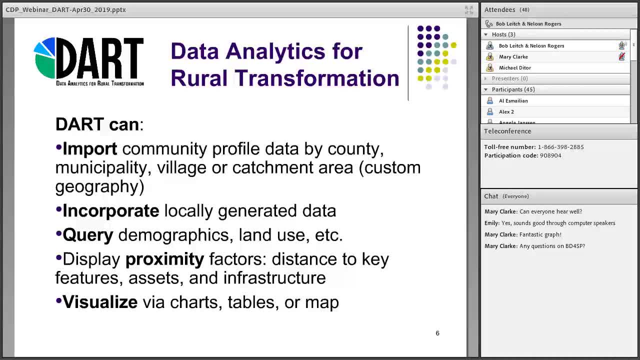 Good Yep tool was done by the Applied Research Group, the Data Analytics Center at Algonquin College in Ottawa, And the Algonquin College Applied Research got a major NSERC grant for applied research in data analytics And we took this- the results of focus groups that we had done with rural. 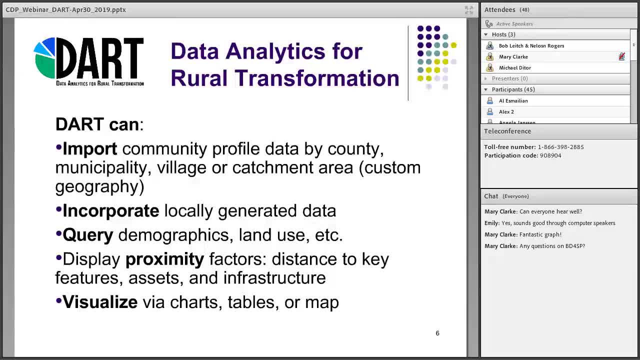 communities about their search for a data tool. We took those results to the college and they put a group of professors and students on this, and the DART system was developed by the college for us based on the feedback and input that we provided. So the DART tool is capable of importing. 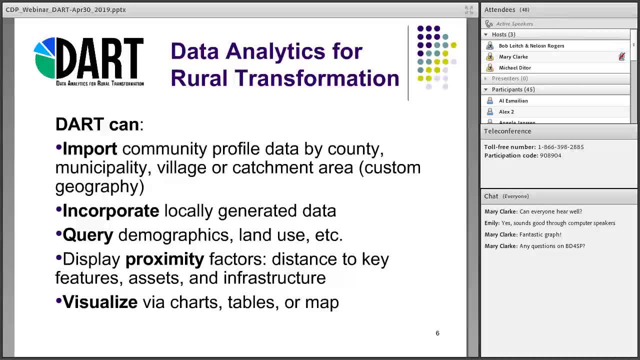 community profile data, different kinds of geographies and custom geography options can incorporate locally generated data, So that one of the townships that we work with has a system called Citizen Scientist, where they have people that are designated to collect data on very specific things and 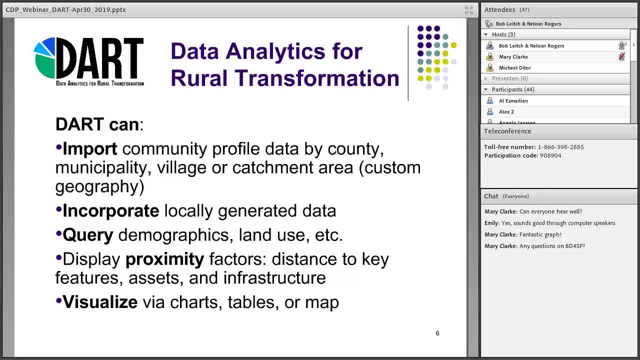 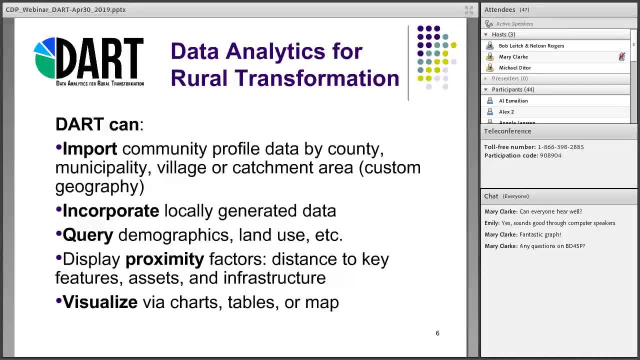 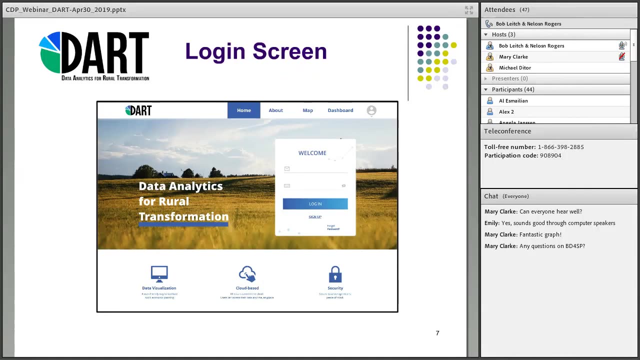 We have multiple menus about how to do queries around demographics, around land use, around specific features, around proximity, And then we have a number of options in visualizing the results of the queries. So the login screens and the user interface screens were developed for us by the college- A lot of these. 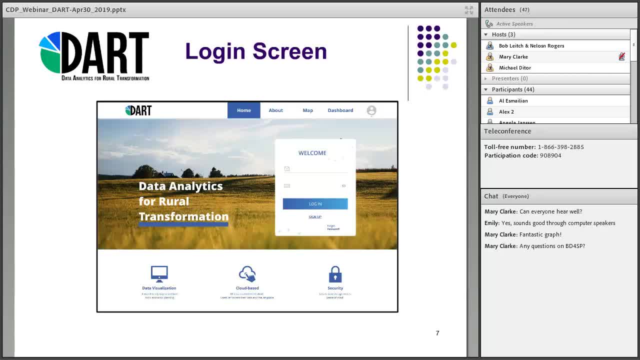 were student projects, students in different programs- interactive multimedia design and in computer science, computer programming- And we have screens that can give you access And we have the ability to compartmentalize the data so that there's, for example, confidential social service data that was uploaded. We have the ability to compartmentalize the data so that there's, for example, confidential social service data that was uploaded, And we have the ability to compartmentalize the data so that there's, for example, confidential social service data that was uploaded. 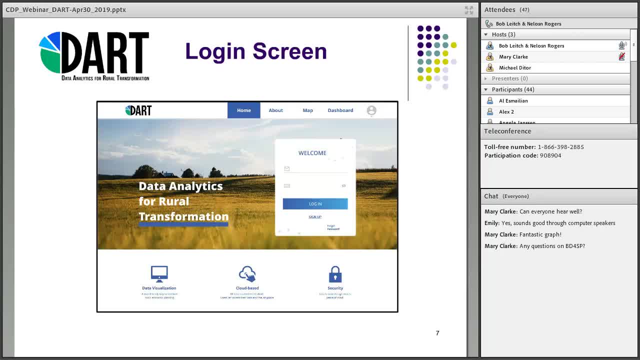 And we have the ability to compartmentalize the data so that there's, for example, confidential social service data that was uploaded to the system. Only the people who are authorized to see that would be able to see it in the DART tool, where. 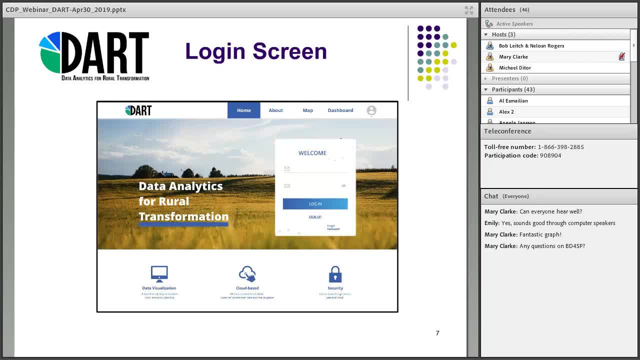 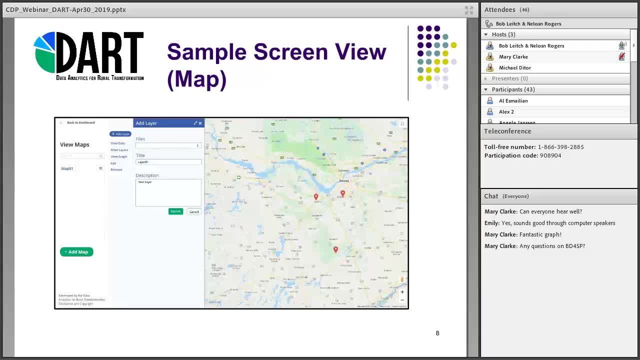 there might be other users that could see economic development data that would be not as confidential. Then we have the ability to. in the map view you can build up layers on the map. So if you're dealing with an issue of where to put a certain kind of business, you maybe want to. 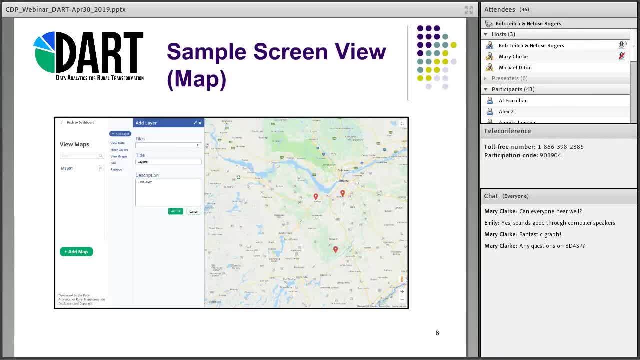 establish an outfitter business in a rural township. you can build up layers on the map on which villages have a high percentage of young adults, which villages have access to a public boat launch, which villages already have an outfitter, which villages have other features of land that's owned for commercial use or whatever. 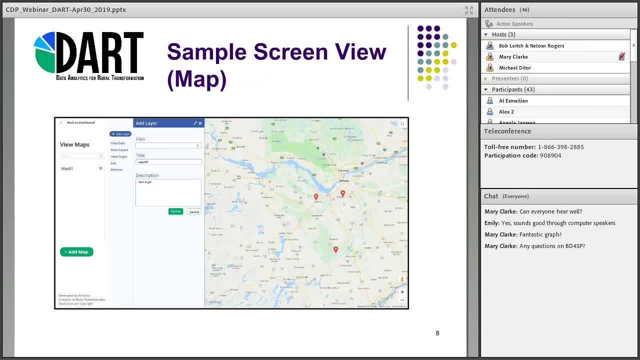 You can do a number of queries and build it up on a map and start to see a cluster of points around certain issues and that can really simplify the decision making. Just another quick example of how the map has been used to be been proven to be useful. 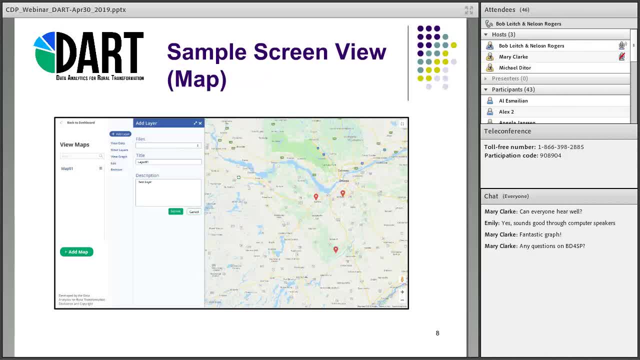 Frontenac County looked at response times to 911 calls, which they had, all the numbers and the success rates and percentages and everything and overall the statistics look quite good. But when they put their best data in the map they're not going to get that. 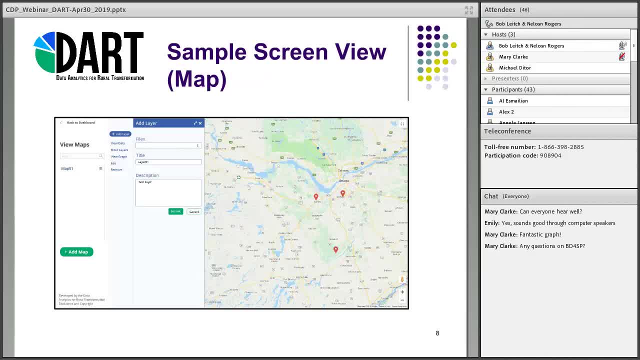 on a map. they realized that there were some hot spots where the 911 response times were not as good and they were really clustered in certain areas. that became highly visible on the map and the issues had lot to do with cottage roads and cottage country, poor road maintenance, poor signage. I really had 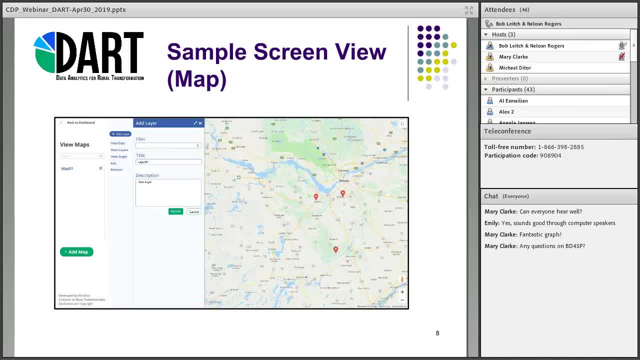 nothing to do with the, the quality of work done by the first responders, by the volunteer firefighters, or or that there were other issues that were relating to the problem, and it was only when they saw the data on the map that they were really able to understand what's the core problem and what kinds of solutions. 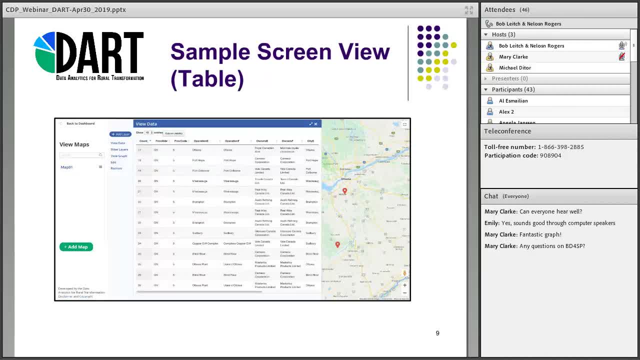 would be helpful. we also had requests for different kinds of table outputs because often the data analysis that's done in a tool like this needs to be output into a report that that goes somewhere to a government department or goes to council. so we've built in different kinds of table generation features, then different 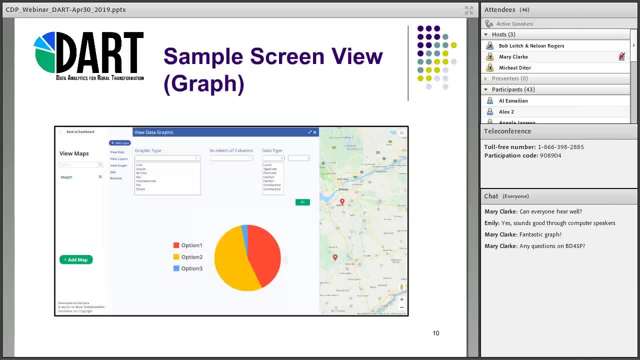 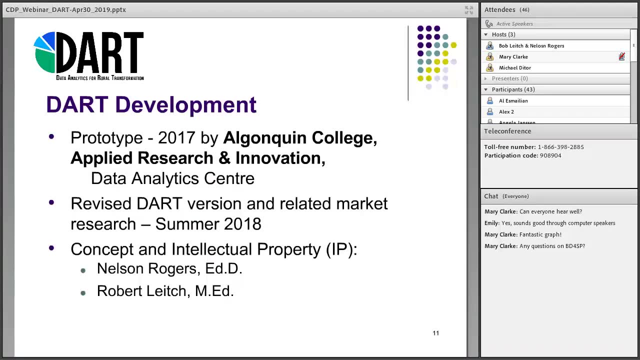 kinds of graphing features next screen there. so we have line graphs, bar graphs, pie graphs, that are options for outputs from the data that comes out through the tool. so we then initial kind of quick and dirty prototype put together by the applied research center at Algonquin College in 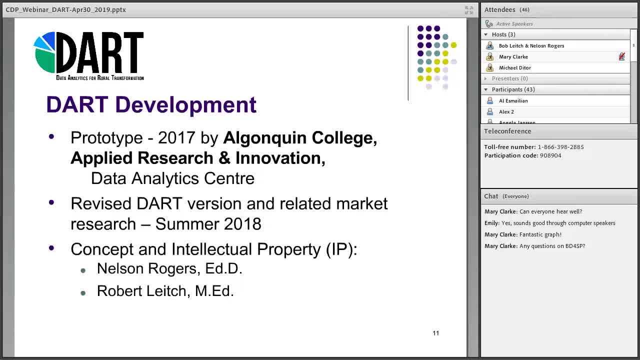 the summer of 2017. we have that being field tested. it's it's not particularly user friendly, but it really proved its value and what it could potentially do. so we use the learning from the prototype to develop a more sophisticated version, much more user friendly, much more elegant system. that was most of the 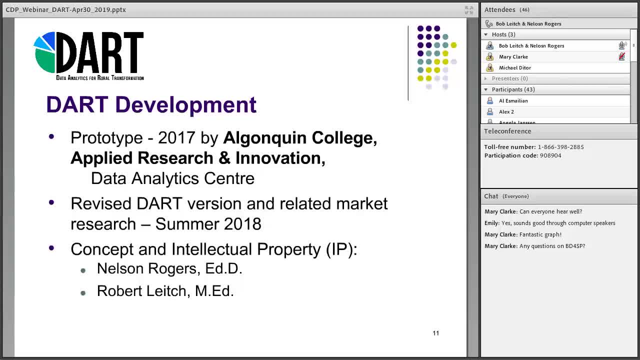 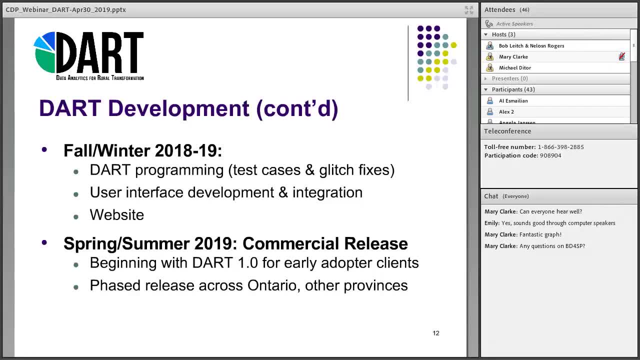 development was done in the summer and fall of 2018 and we're just in the process of working towards the release of that. we're right now working through some system integration and testing a few glitch fixes and we're very close to having this available on for commercial release and 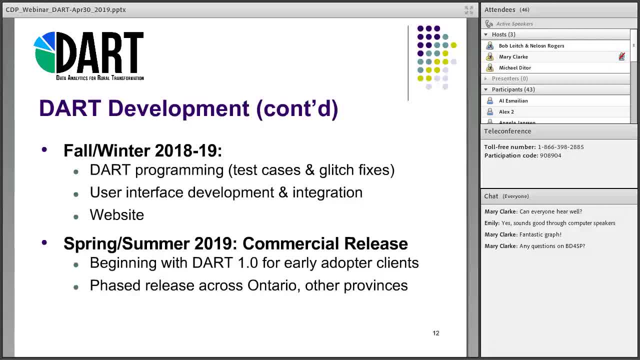 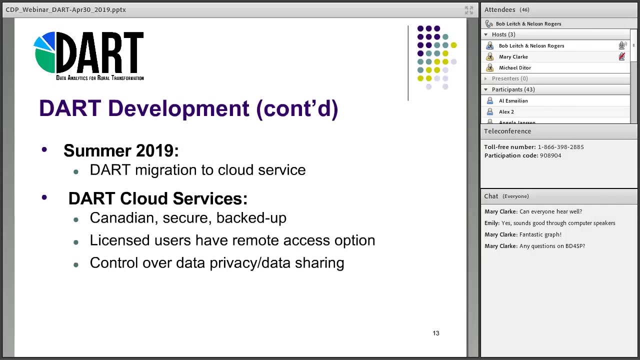 we have been accepted into the canary program for cloud service to have access to a very robust federally sponsored cloud service that we can use for this, for testing with our early adopter clients before we go to a full commercial release. and we're looking at that- we're probably a few weeks away. 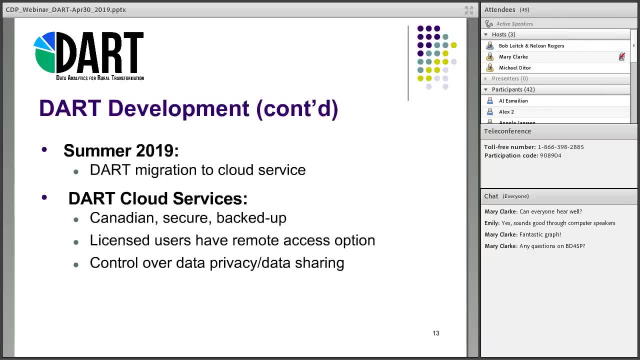 from making that available to a select group of early adopter clients. so, um the at the moment we have uh one dedicated um uh programmer working on the uh linkage between the back end system and the front end system, the dashboard. uh, that work is probably going to. 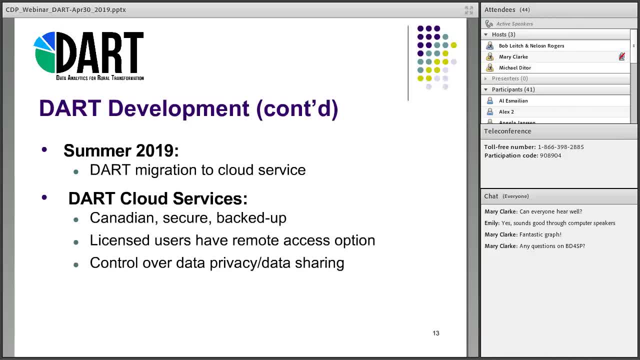 be complete within the next three weeks, uh, and then we'll have a model or not a model. we'll have a product that we can demonstrate, um. and so, if that interests you, uh, at the end of this um session, if you wanted to let us know um about your interest, we'll make. 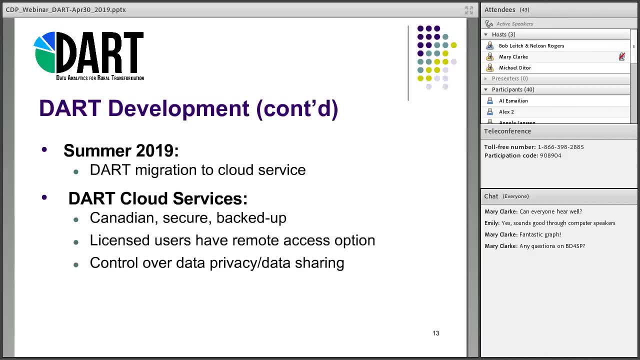 sure that you're notified when the time comes that we can do a demo online for you. um and um the um. we're planning that. the cloud service, the cloud service, that the canary service, is the federal government department. if you're not familiar with canary, they deal with all things. 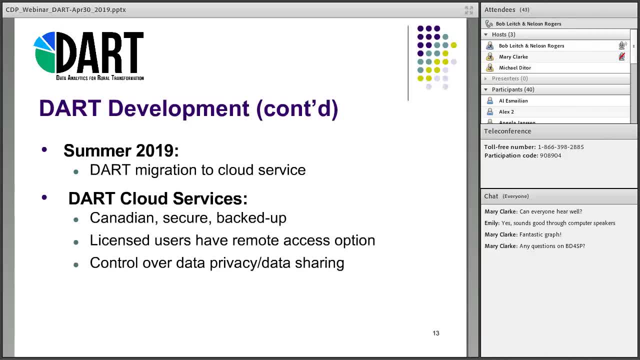 relating to Canada's involvement in the internet: rules, regulations, policies, etc. but they also do have a research center and they have approved us to be on their secured service to do the test run-ups and so on before we go commercial. and that's going to be happening imminently, probably next week, and that'll be there. 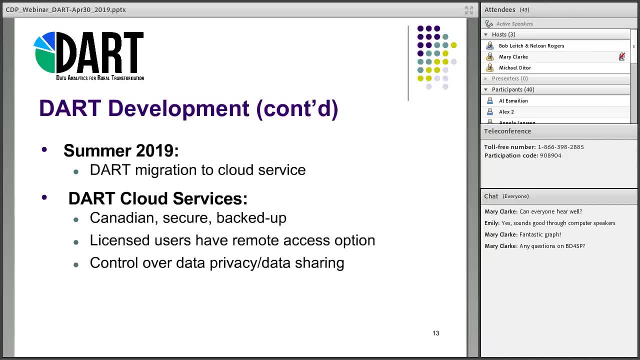 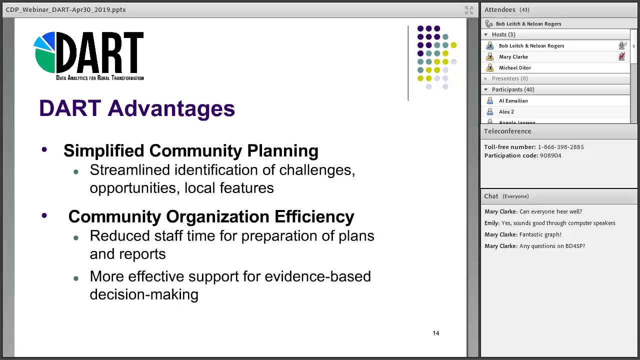 for, and they provide technical advice around, certain features that we may want to build upon, such as using artificial intelligence for combing for updated data from the sites that provide that service. so that's our, that's our immediate situation and the advantages that we see of this tool. 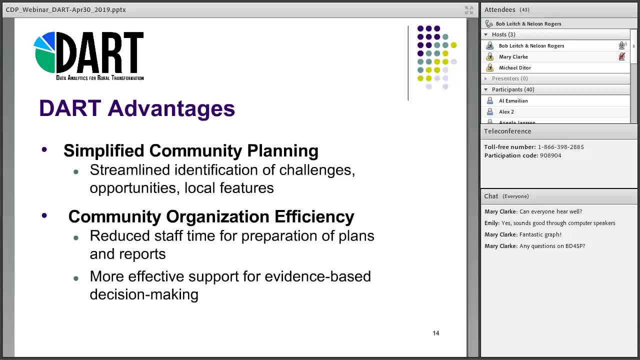 you is that we we firmly believe that it's going to be create some real efficiencies for those community organizations and municipalities that struggle with data collection, analysis and integration and visualization. so we're expecting that's going to really be of particular interest to them as we move forward and that's 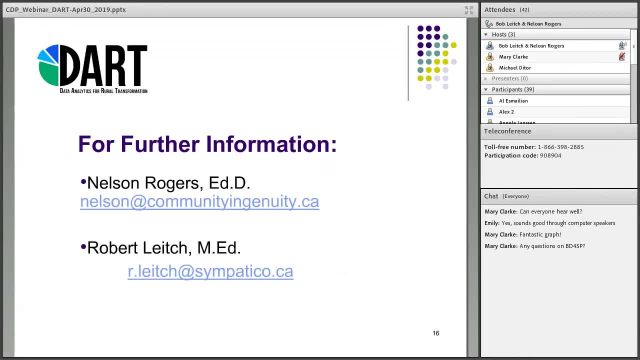 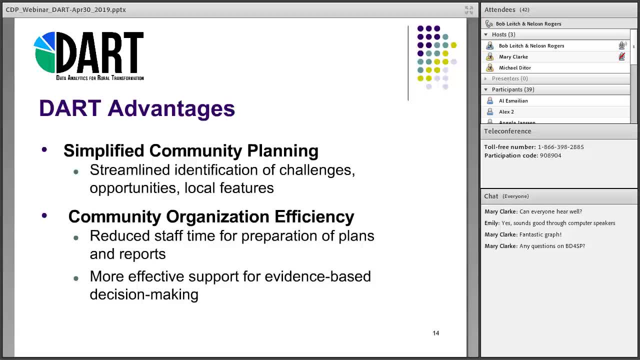 you basically it. that's us go back. okay, so we're going to go back, hang on. we developed the DART organization based on focus groups with potential users, but since it's been promoted by Algonquin College as an example of what their applied research group can do, we've had some interest with several federal government. 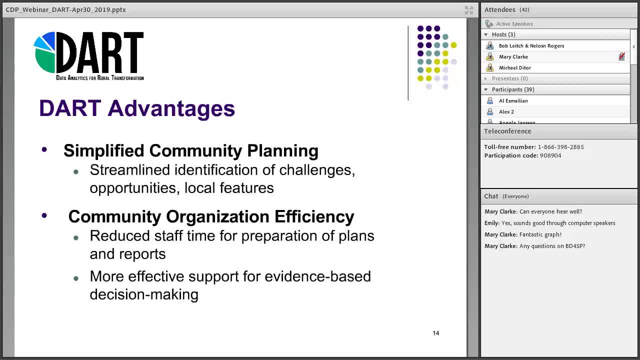 departments and agencies that are looking at the DART tool to simplify the collection of local data and the formatting of it for submission to government departments, as the, for example, Statistics Canada, doesn't have the same, the same type and the same number of field researchers that they. 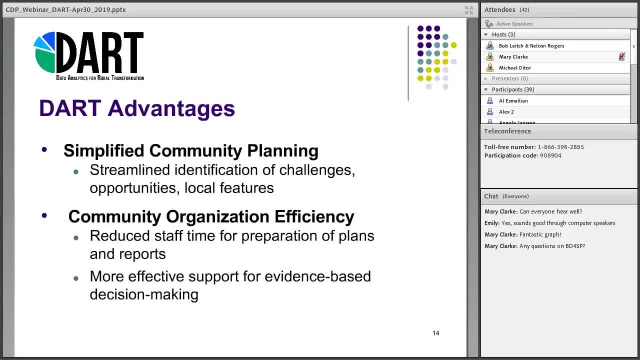 used to have and there are things that come up through local research with the community groups are doing that. it would be useful if it could be incorporated in alongside Statistics Canada data, but there aren't easy systems right now to verify the validity and the reliability of locally collected. 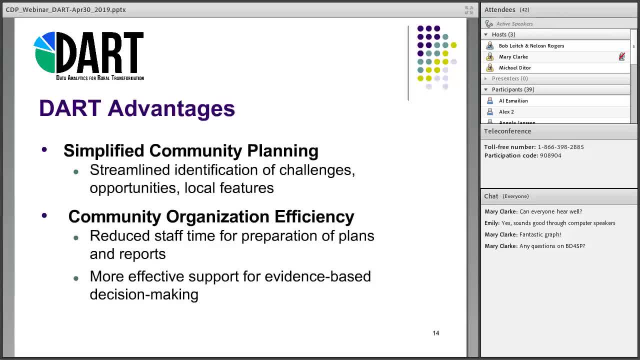 data into a and putting it into a format that's that's easily incorporated into government data sources. so they've been talking to us about adding some features to the DART system to do that. so we had envisioned DART mainly as a data pull system, pulling data down from open data sources to make it useful at the 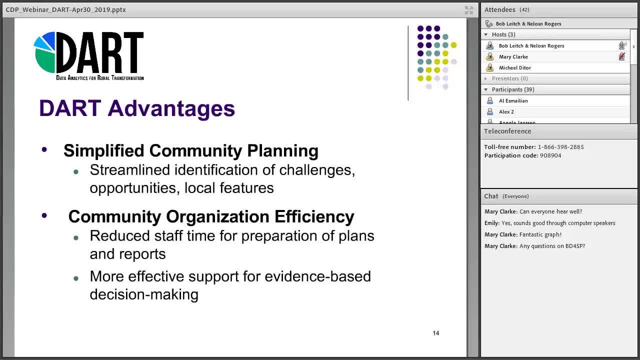 community level, and now we're seeing some interest in data pull the other direction, pulling local data out of the communities and submitting it to departments and agencies. so it's been a fascinating project to be involved in and, by using the college students and college applied research, we've been able. 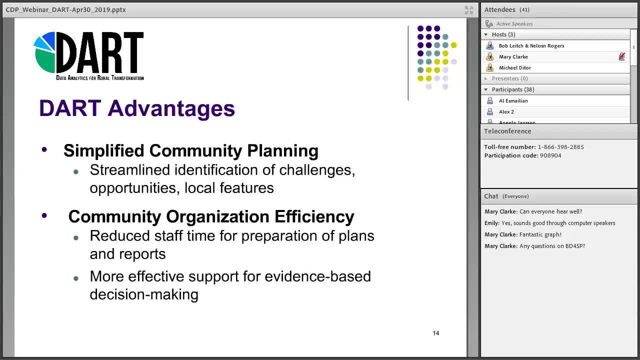 to keep the development costs down so that we expect to be able to bring this to market at a very reasonable price point that small community groups could afford. there are some commercial products out there that they're available for data integration, data visualization, that are quite expensive and and not really flexible. and they're not really flexible and they're not. 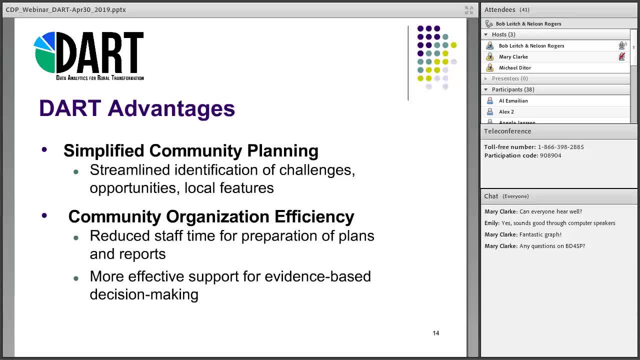 for rural community use, and there are some groups that are struggling away trying to develop their own internal systems to do this, and it's quite inefficient for each group to try and invent their own system. so we think that by making this available we can really support more effective use of data in 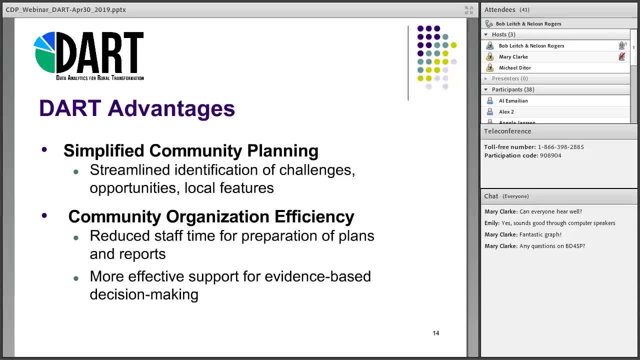 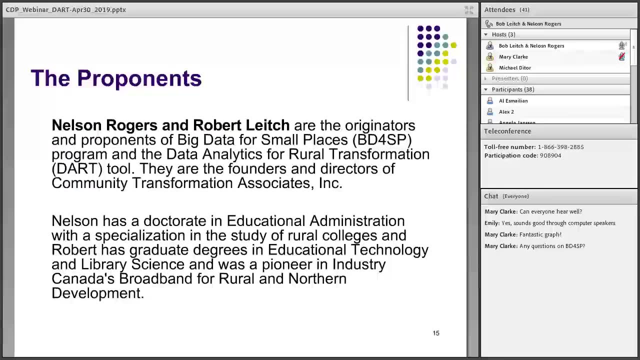 rural communities and by community groups. I guess I should mention that we have a website under construction. it'll be under under the company, the new company named Community Transformation Associates, and it will have a section in it with DART, and what we're going to do is that that is being constructed now and we'll 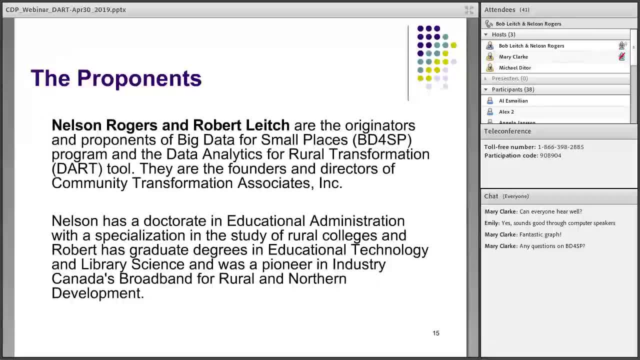 hope it'll be ready at about the same time that we're able to release the first version of DART very shortly, and so we're looking at probably six to eight weeks at the most, and so if this interests you, please let us know and we'll make sure that you're. 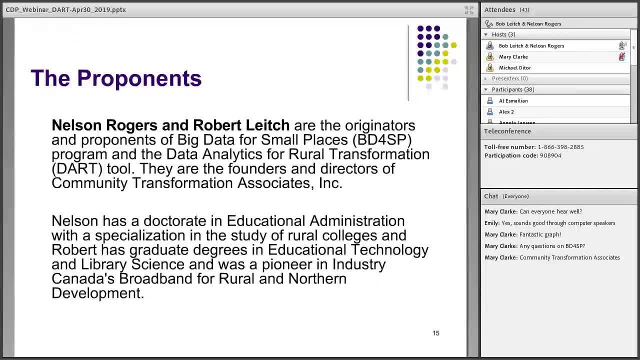 you've at least get the announcement and if you want to follow up, that would be wonderful. we're really excited about this project and we we've talked to a lot of people who are in this world that of data, particularly Stats, Canada, the, the Standards Council of Canada and, in fact, interesting. 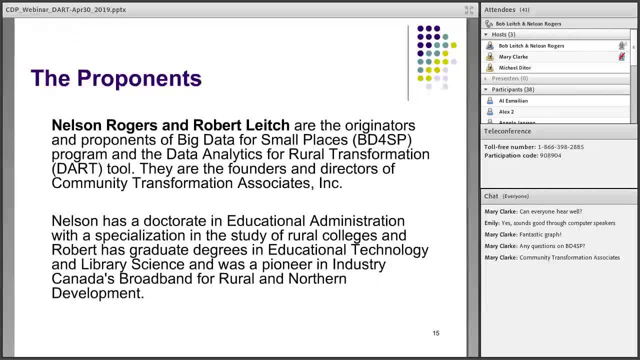 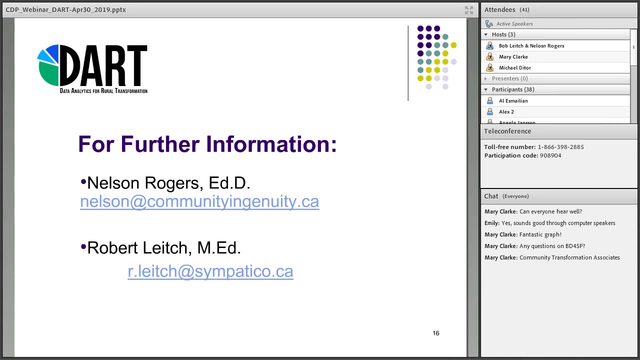 enough, the department national defense, but particularly as it relates to a national public safety and security. so there's there's a lot of interest in this project and we're hoping that your group will find it of interest as well. so, that being said, I think we're able to take questions if you wish. thank you, 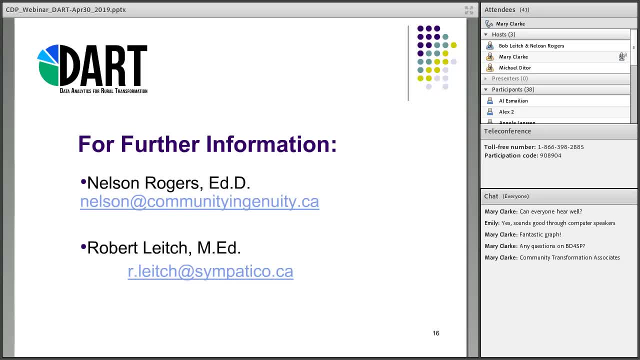 very much, Bob and Nelson. that's great. I think that's a large. thank you very much, Bob and Nelson. that's great. I think that's a large, a large. thank you very much, Bob and Nelson. that's great. I think that's a lot of information for people. we do have about 15 minutes for questions, so 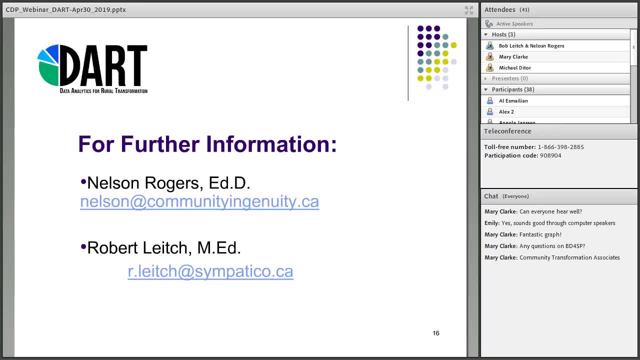 feel free to type in your question into the chat box at the side of your screen there and we have Nelson and Robert's information up on the screen. so, and like they mentioned, please contact them directly if you want to have any of the announcements about the projects as they move forward, and so you'll get the 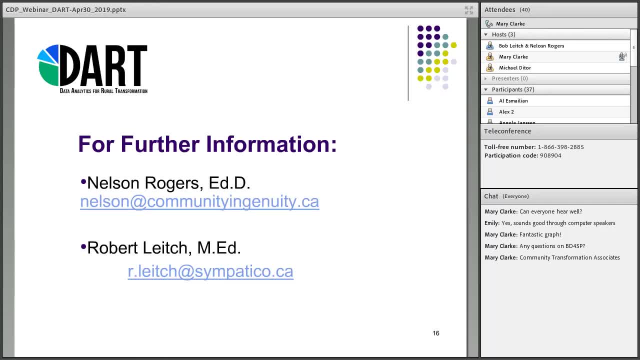 announcements of when things are happening and you'll be able to contact them further if you want to get in touch with them, if you have any questions that you want to figure out how to bring them to your area, or if you had any follow-up questions for them- and they're both, as you can probably tell they're. 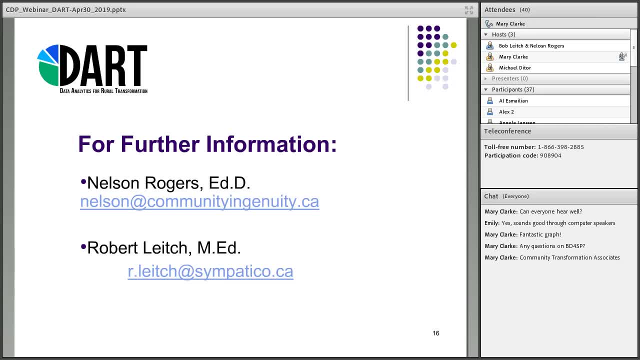 both very easy to talk to and and they're they are very excited about this, so they'd be happy to share and really push this project forward with any partners that want to come on board. you know, for those of you who want to come on board, if you have any questions. 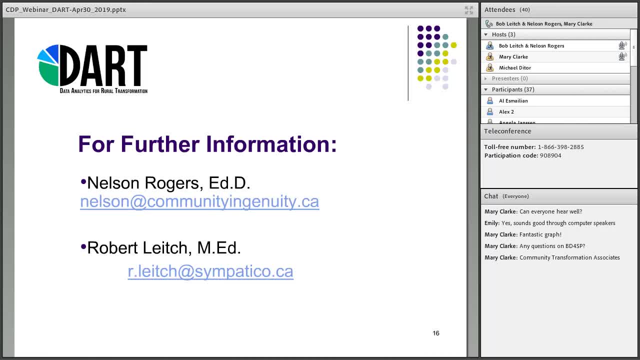 that are kind of crazy and you're not sure what you want to do for your business. but I know there's a lot of people who are- many of you are- high capacity users. do you notice in your organizations, particularly if you're working with in a Rural organization, do you notice that there's a big problem? 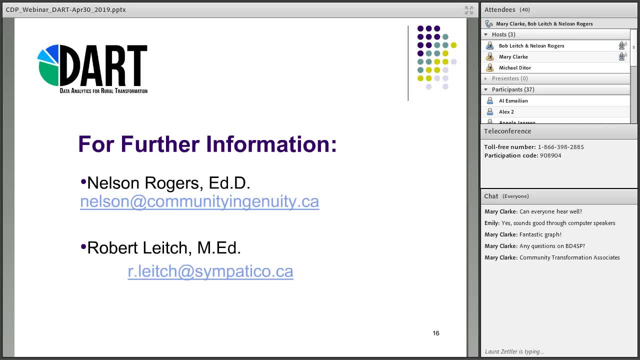 with just capacity and the capacity to work with data. are you often trying to find outside consultants and you know other people. give people a few minutes here to respond by chat. what we found in our work with a number of community groups is the, the designated data experts in. 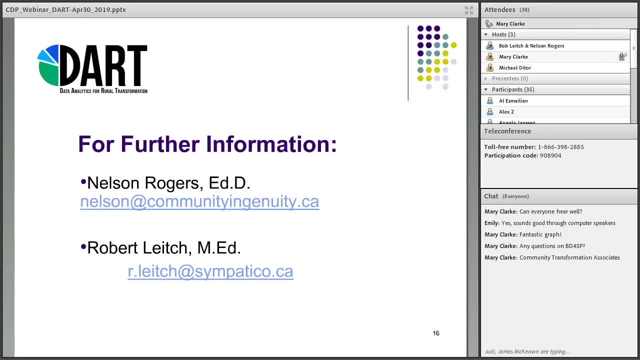 the organization get overloaded with data reporting requirements and really don't have the the freedom and the time to build data literacy across the organization. and and that's you know where that our big data for small places program isn't trying to replace the data experts in the organization by any means. 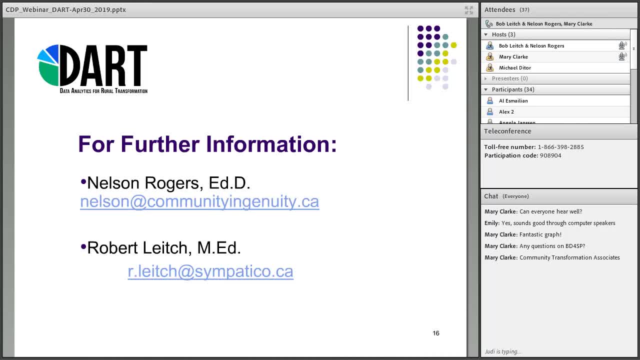 but it it's providing ways to make the data expertise more useful across the organization. so we've had some interesting, some interesting experiments with that, even in those organizations where they have in a certain designated in-house experts in data. sorry, I think we're having a problem with our chat box. I can see. 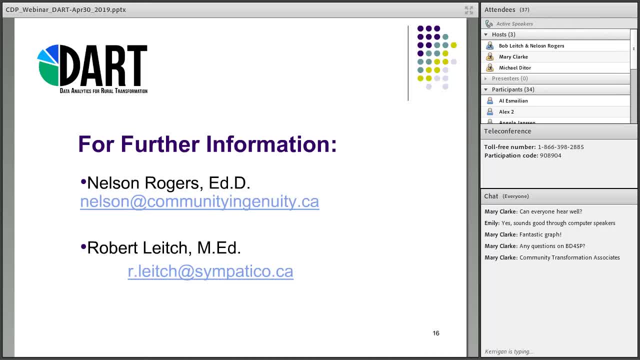 people typing and I cannot see your chat coming up, so I'm going to. we're going to try something. sorry everybody. oh, here we go. for some reason, then you're just taking okay so from question from. Judy was a student at customers and they did a lot of work herewar. 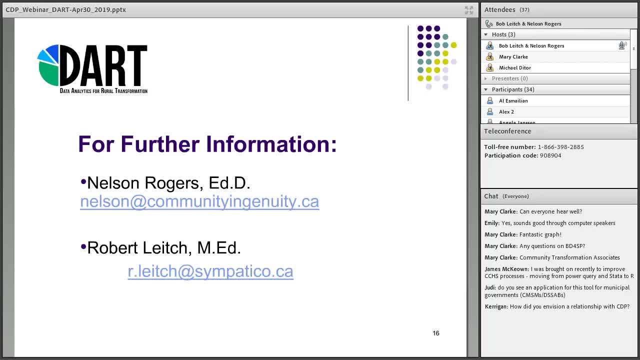 do you see an application for this tool for municipal governments? absolutely, as a matter of fact, our principal audience has been municipal organization, or sorry, municipal bodies at regional and local municipality levels. we also have significant interest coming from in Ontario, in particular ministries that service those municipalities, like the entire Ministry of Agriculture and Rural. 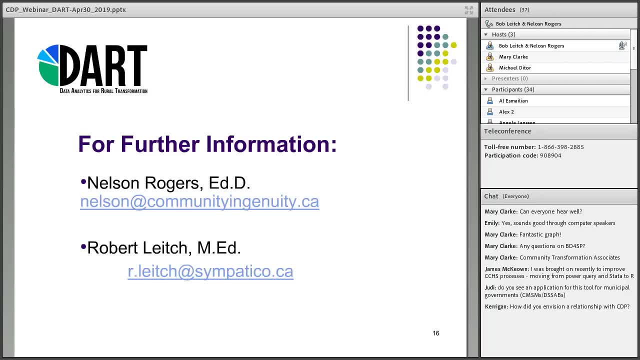 Affairs and the municipal affairs Ministry of Municipal Affairs in Ontario. so there it's very much a significant audience for us, particularly in rural areas and small communities. so that, and we've, I'm not sure so for the question about tool for municipal governments, the, the DART tool. 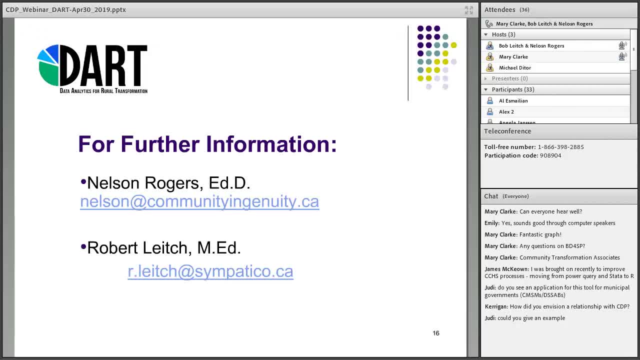 was developed primarily around the results of focus groups with staff at municipal governments, some community service organizations as well, and the commercial products that they had looked at for data integration. data visualization were either too expensive or too inflexible to really meet the needs of municipal administration, and that those are 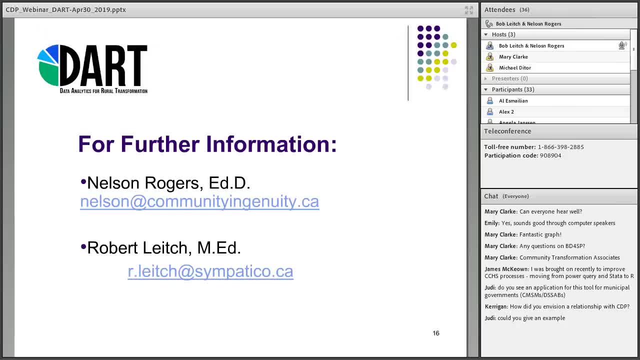 issues that we address specifically in the DART development. you know, as we were developing this both in the prototype and as we moved out of the prototype into the current version, we had ongoing consultation and feedback from a variety of municipalities, not just one, and we went to very small ones that had small 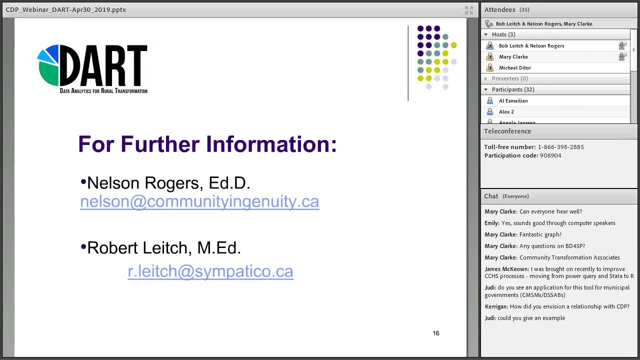 population to a fairly well large, meaning 15, 12, 15 thousand people, and then three cases they were counties. the whole County was involved. so we've got we, as we had the consultation sessions, we did them in person for the most part, although some of it was online and we kept going back to them for clarification about certain. 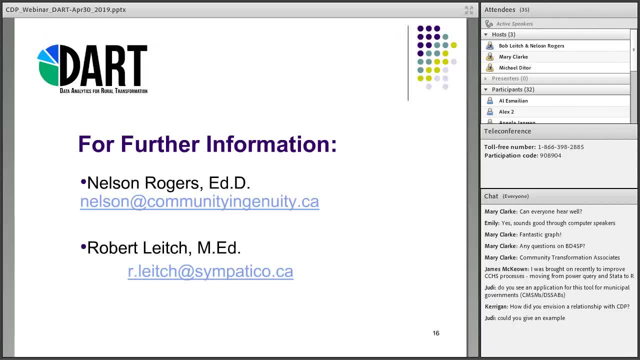 aspects. so we're hoping that the version that we release of DART is going to be more to the local locations and to the local communities and to the municipal departments that have the platform at the local levels and the various agencies that are involved. we're hoping that the version that we release of DART is going to be able to dassive and implement a higher level of information about that. 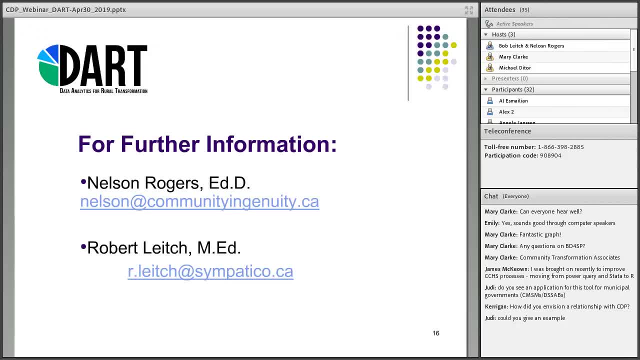 be very well received by municipalities because of that process we went through. we're hoping so. I see the question about in a specific example. so one example was the understanding 911 calls and how to improve response rates. another example we looked at from a similar system that was used by a city that we looked at. 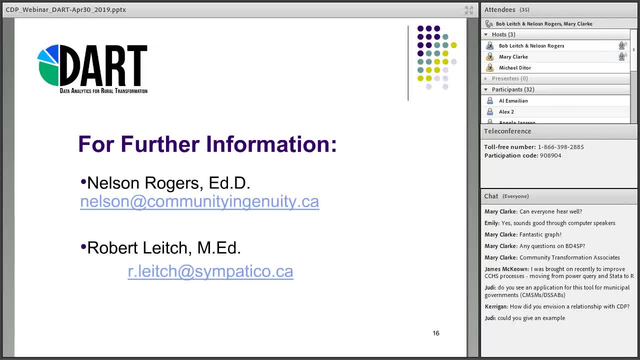 that was doing some work with data visualization is they? they looked at the address of people who come to a hospital emergency department for non-emergency reasons and once they put that data on a map they saw there were neighborhoods where that we're generating a very high percentage of the. 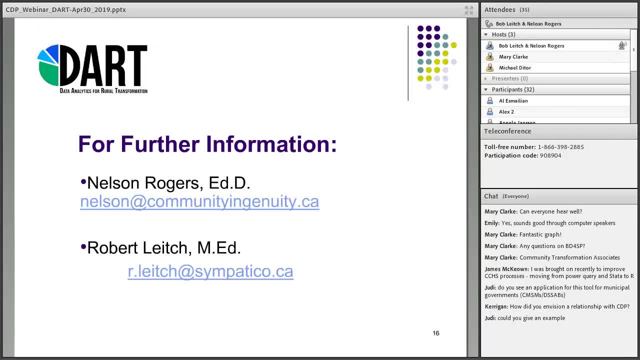 non-emergency visits. so that gave the department some insight into where to locate health clinics, what kinds of public health outreach work needs needed to be done and where it needs to be targeted. so it's that integration of data and then visualizing it on the map gives a level of understanding of local 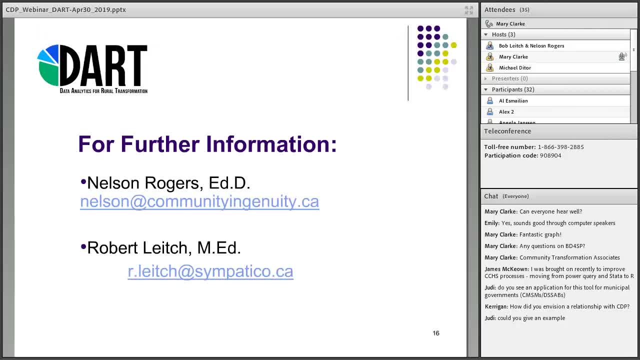 community problems, municipal problems that are difficult to do without that technology. on the other, there's a question here from James. okay, I'm not sure if you're hearing me. okay, yeah, I think so you are. you are on the, on the uto, on the essential data, and there's a question from Hilary, from JACK. 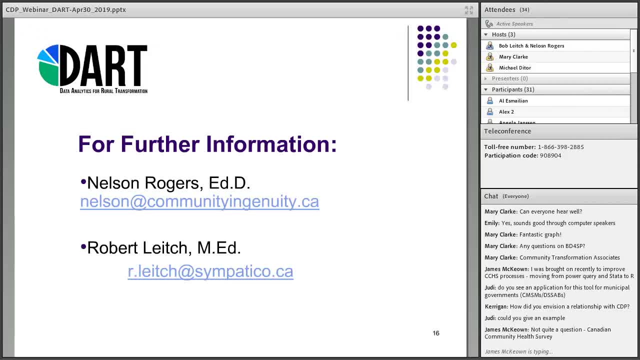 I believe that the health data is helping people with the most difficult health stress every single day in the community, and I believe our data to the end of the year is a little bit more than that. I'm not sure what you're saying. that's all. I'm not looking at too closely for a. so is that the, the, the, the CCHS? is that? oh, that's, um, that's the health data, I believe. okay, I think it was just offering his perspective, his role and what he was just offering his perspective, his role and what he 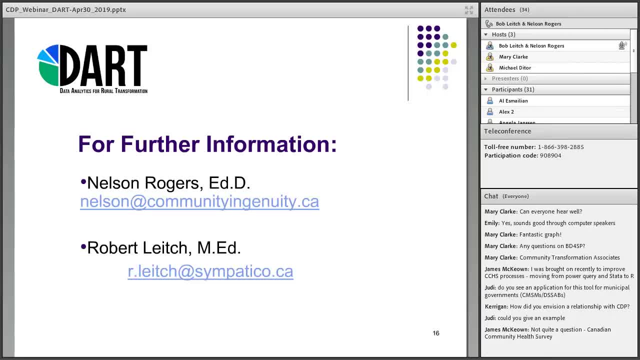 direct contact with one community data consortium in our area and there was the people that were working with that were saying that the participating organizations now had access to a lot more data than what they were making use of and they're just wondering about what the stumbling blocks were that there. 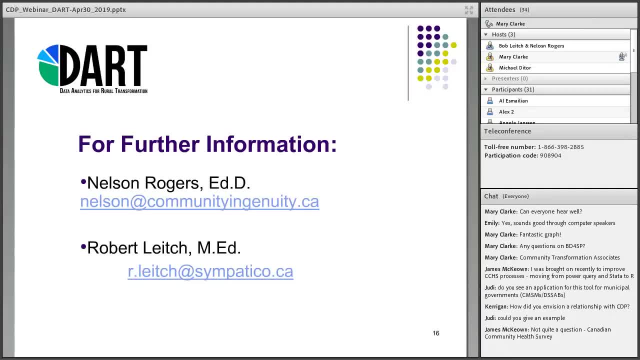 wasn't more utilization of data by local organizations, and we in our conversation we suggested that perhaps some version of the big data for small places program would spread the data literacy across broader groups of people and and that the end results would be much more effective and much more. 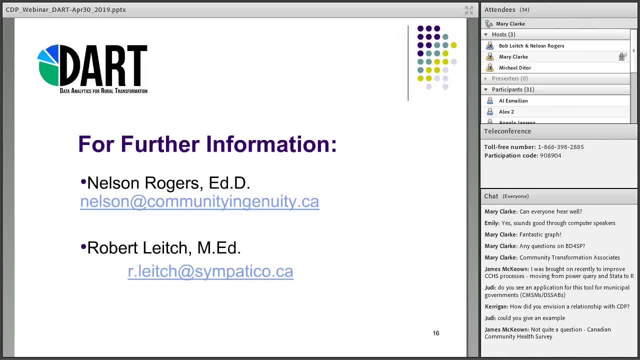 widespread use of data by the members of the community data consortium. so that that was just one example of that that we, that we that we thought came up, maybe, yeah, maybe Mike can speak to this as well, because Mike's been involved with a few of these discussions too. this is just sort of an initial 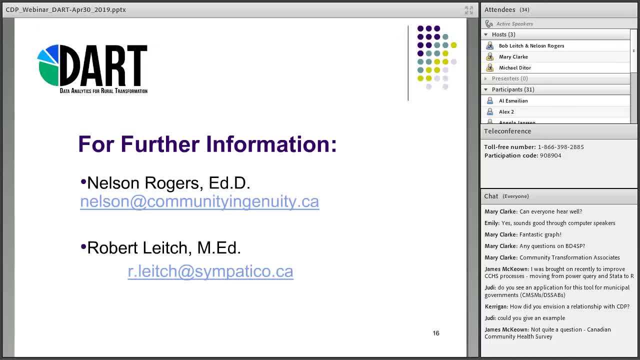 beginning, and so we're really wondering- and maybe this is a question to the audience too- is if you see how this could really benefit to have a formal partnership. could American, I just add- I'm sorry, I didn't mean to it, Mikey- did you want to? 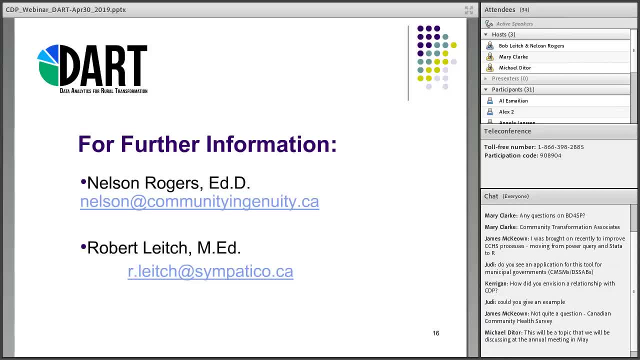 speak. I think he's ice can see him typing right now. so, okay, oh, there he is. yeah, so this is gonna come up at our annual meeting we made just in a couple weeks now in Calgary, and it's our one face-to-face meeting a year, and so this would be a 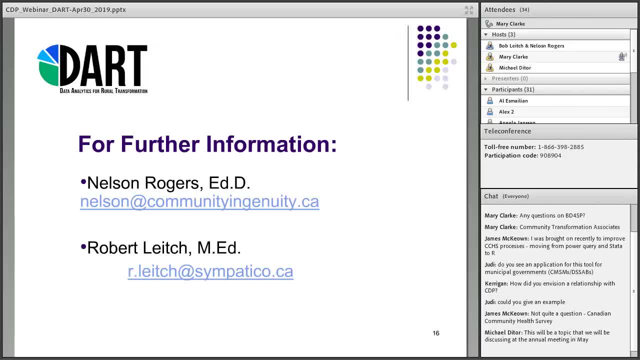 chance for us to talk about what partnerships we want to explore, and so this is actually really great timing to have this webinar, because it means that we'll be fresh in our minds two weeks from now. we'll have time to think about it and discuss it further, so please do that for everybody's participating today. 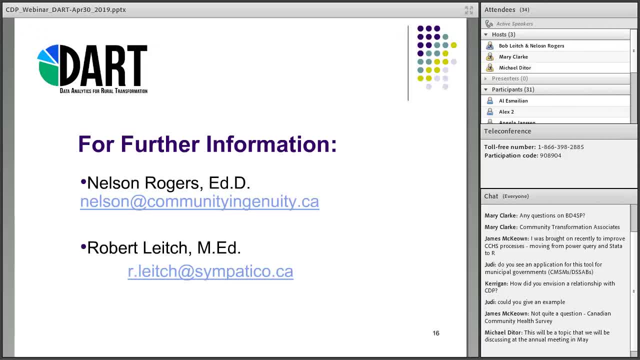 you know, what do you think a partnership could look like? and there's obviously a a lot of natural overlap between what we're doing and what Nelson and Robert have been working on. we believe that as well- in fact, part of the conversation we had early on with Michelle. 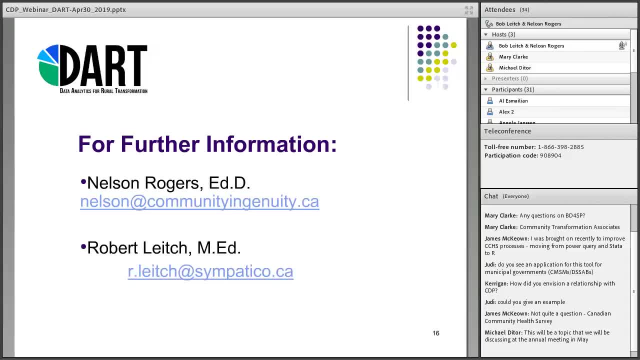 and with Mike I was around the notion of the strategic plan that the community data program had and in particular around a data literacy, developing a better understanding of data and how to use it, and the big data for small places program kind of addresses that and and I would 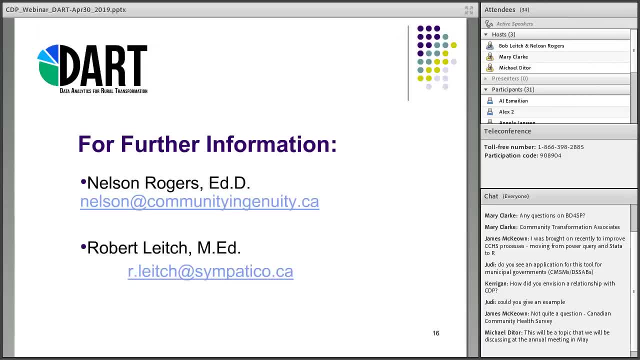 think that if we could work together going forward, it would be to take that, enhance it, perhaps make some aspects of it online, interactive, etc. I wanted to just also just mention to James, who asked a question about the Canadian Community Health Survey. James, I'd be interested in hearing from: 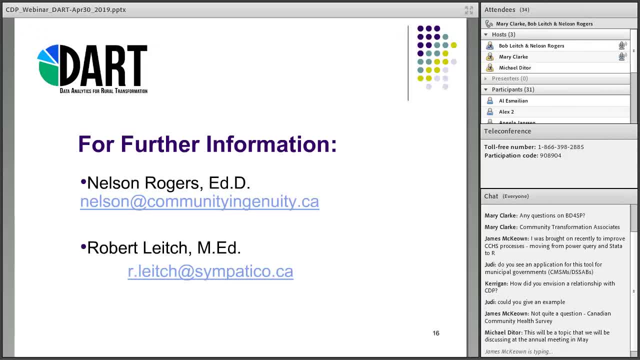 you about the community health survey and what you think about it and what you think about it, and if you want to take my email address there it's on the screen. I work with a governance forum in this region of Ontario and very much involved with the data question, so maybe we could have. 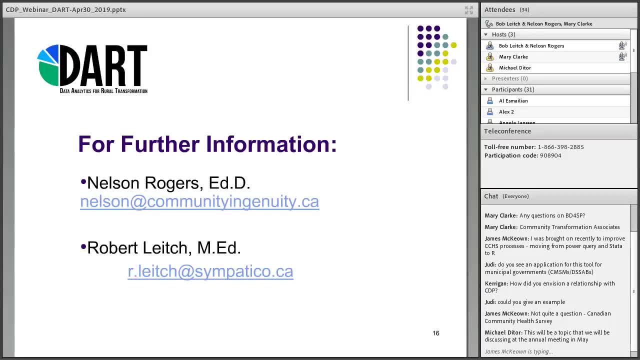 a chat offline and there was. did we answer the other ones? I think so, okay. the other thing about the potential relationship with the community data program. we didn't emphasize this, but we have worked on the development of multiple versions of big data for small places or target audiences and we've sketched out- been Rick, it's been requested from a potential 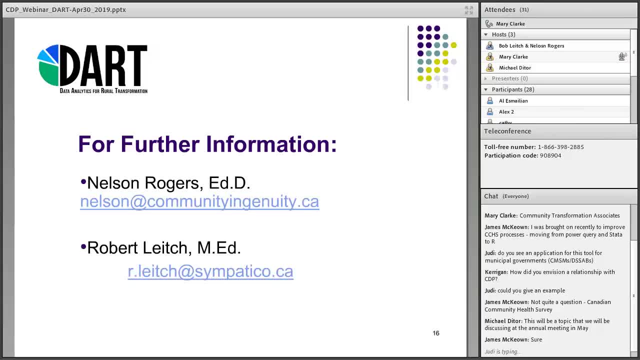 client, a fast-track version of big data for small places for people that have already are already part way up the ladder in terms of data literacy, and I think it's important to emphasize this. but we have some of the resources that we've collected as part of the big data for small places program, so we do. 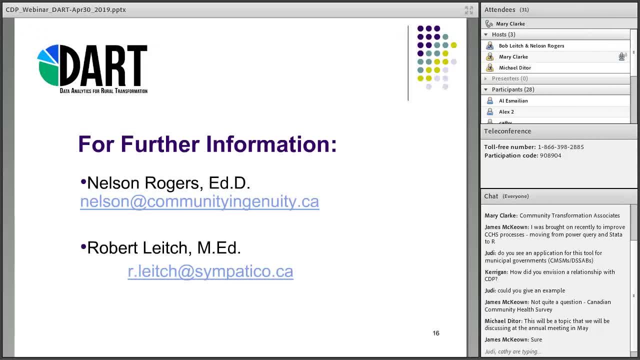 have a fast-track version. that's for moderate to advanced users, and then we have a very general introductory version that's just gives the flavor of the potential of using data for community use. that's a community orientation introductory session. so we've we've sketched out three different versions and we're looking at 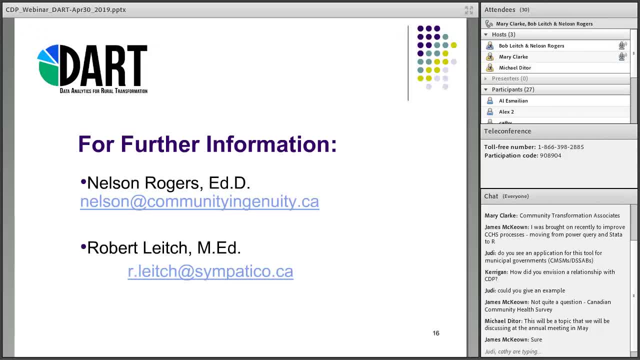 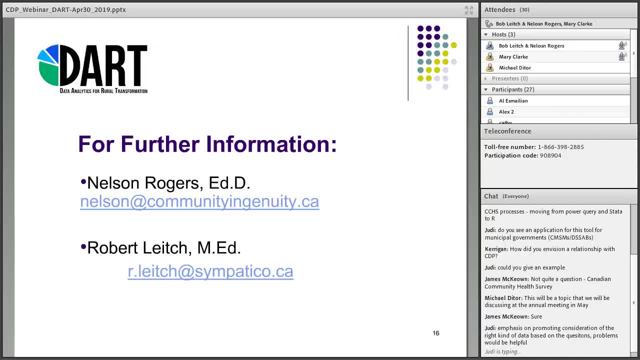 make a last to you is to make it a program, a version of it, that there'd be a program of your own and we would talk about, talk about how that might work. we certainly would like to see more partners involved in illness. the program was developed in response to needs that were expressed to us and as other 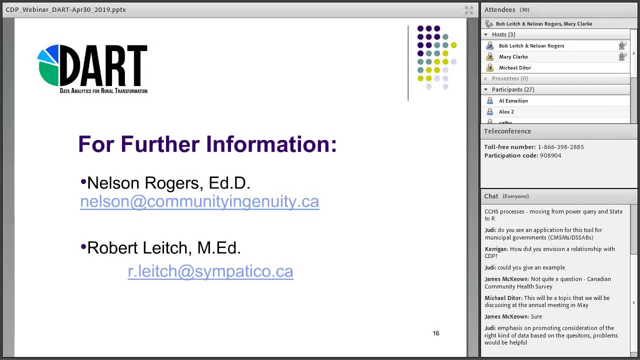 needs become more clear, we're quite able, willing to adapt it also. you know, I think it's really. I should just mention that both Nelson and I have been in our former formal careers, were involved in the the education sector. I was with the Upper Canada District School Board and prior to that, the Leonard County Board of 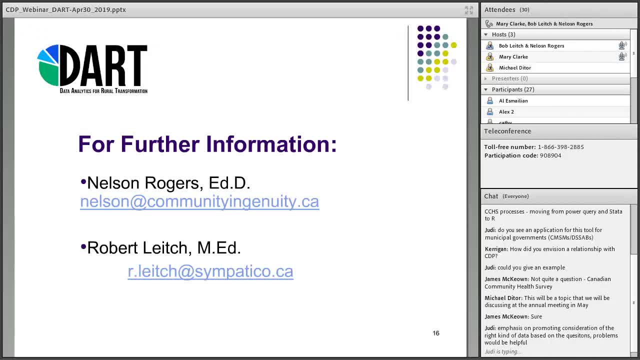 Education as a teacher and a school administrator and eventually a supervisory officer. we're sensitive to the principles and practices of andragogy, adult learning, so we assume, when people come to a new event, a new idea, that we first find out where they are with regards to what they already. 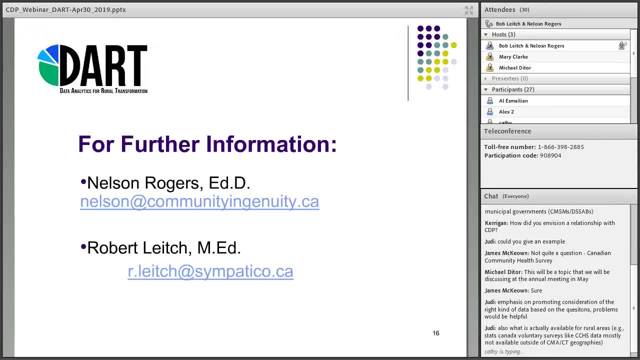 know we don't assume that we have to start from the beginning, so that could be extremely positive in working with a group like yours. I think absolutely yeah, and I'm looking forward to this discussion we're going to have in May because we will probably be meeting. 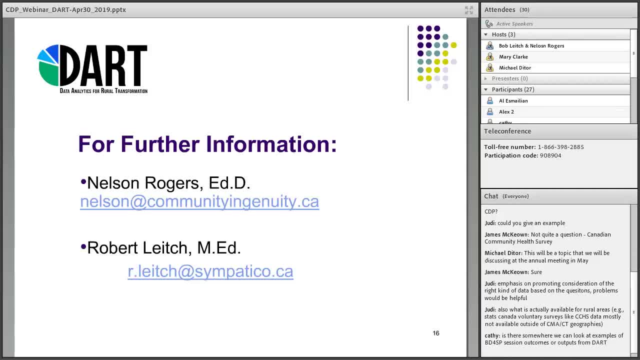 in person in Ontario next year, in 2020, and so that might be an opportunity to actually have an in-person session with Bob and Nelson, so that's something we will definitely discuss coming up. we are coming to the end of our time together and so I'm going to formally wrap us up, so thank you very much to Nelson and to. 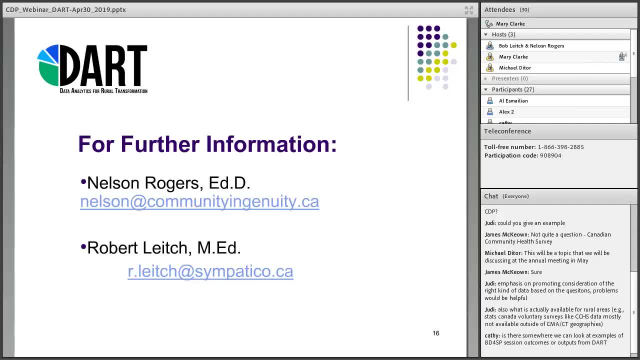 Bob and I think these are wonderful projects and you can see how much work has gone into them and I think that we can definitely benefit from that. Thank you. I think it's really important. we can definitely benefit somewhere down the road here of coming together and doing something together and, in the meantime, 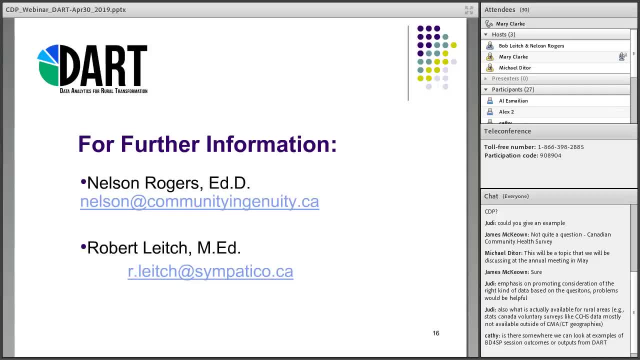 if anybody would like those updates on the projects as they're coming more available and more online, please directly contact. the emails are on your screen right now. take a minute to write them down. we will make sure to get the slide decks up on our website. my colleague, Julie is just on vacation now.